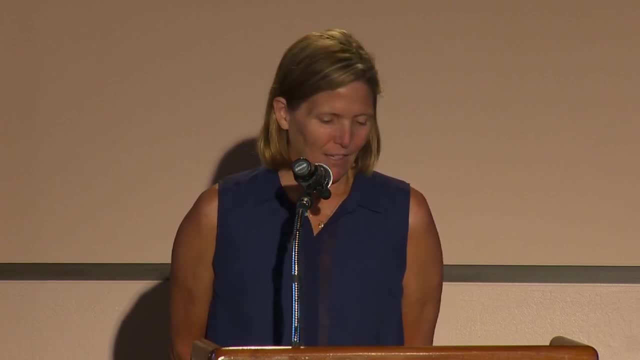 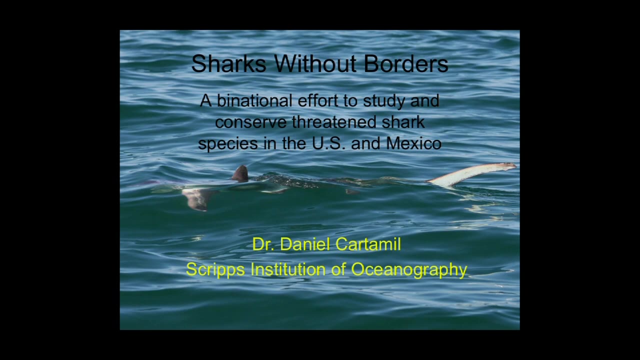 and his PhD here at Scripps. Now there are three things that you need to know about Dan. From the title of the talk you can probably guess. The first one is that he's a shark expert. He's an expert in the. 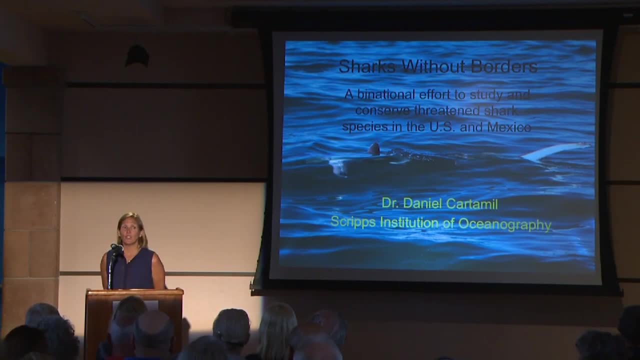 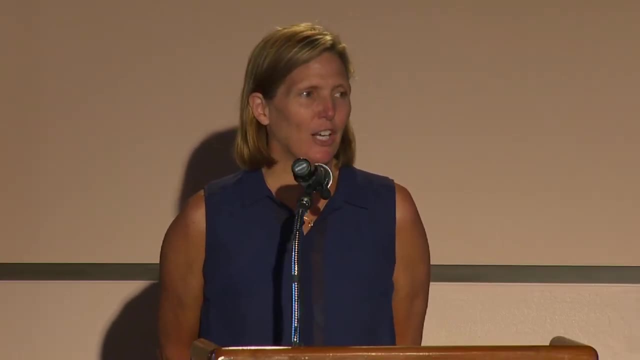 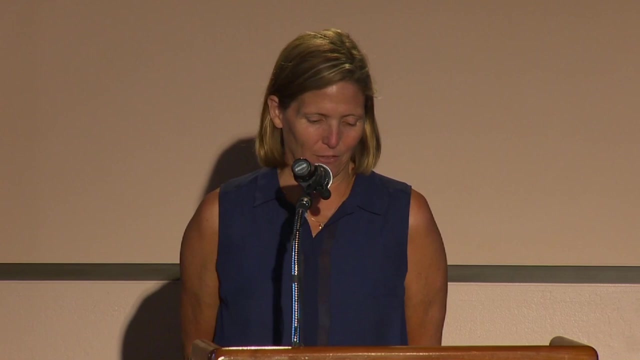 movement patterns, ecology and shark fisheries of open ocean sharks, and that's what he's going to speak to us about this evening. He's gonna talk about both: sharks here off our own California Coast and sharks offshore and our neighbor to the South, Baja California. 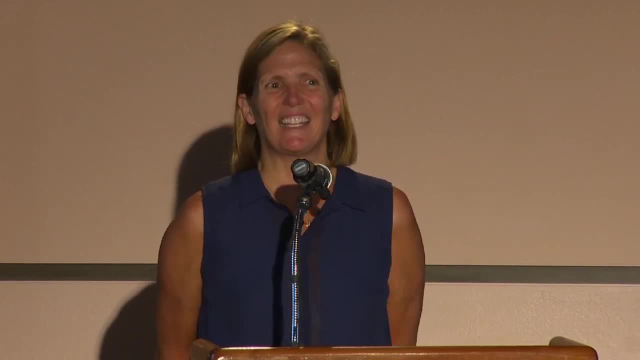 For the day. we'll talk a little bit about romantic allora, Just a couple of tricks that you need to know about Dan. In fact we'll you can talk for the whole of the women's need to know about Dan, and I didn't tell him I was going to say this is that he's. 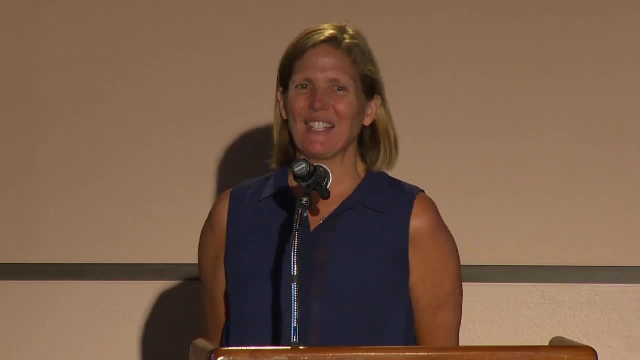 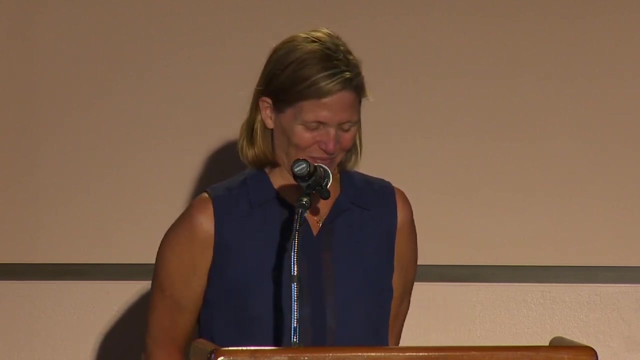 a drummer, And apparently he's been a drummer for 30 plus years and he loves to play things like congas and a whole host of other percussion instruments whose names I didn't recognize. So I'll have to catch up with Dan on that at some point. And then, finally, and perhaps, 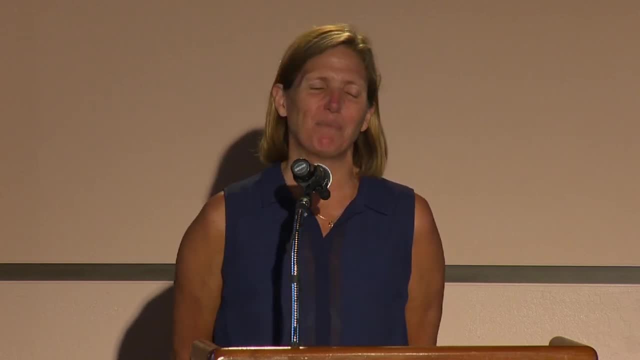 most importantly is that Dan did his PhD degree here under the guidance of Dr Jeffrey B Graham, And then he also served as a postdoc with Jeff, And so, like this lecture series, Dan is actually part of the legacy that Jeff left to this institution, So I hope you'll. 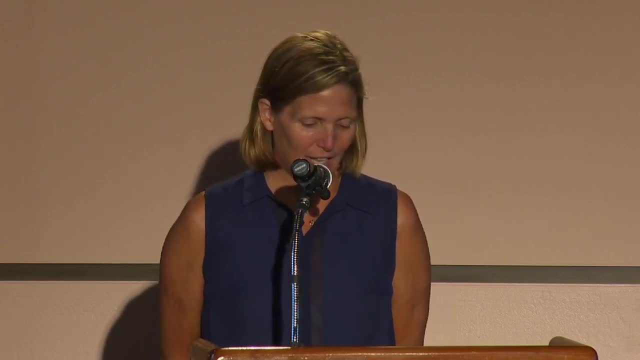 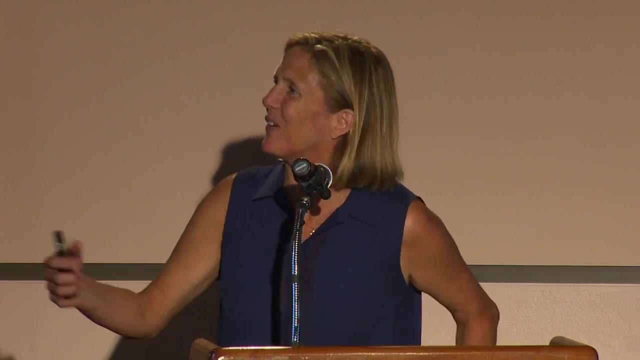 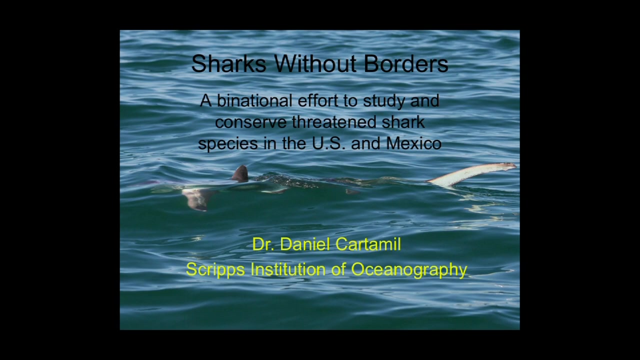 all join me in giving a very warm welcome to Dan Cardemille and his talk titled Sharks Without Borders: a Binational Effort to Study and Conserve Threatened Shark Species. Thank you very much for coming, Dan. Hey, thank you very much. It's a great pleasure to be here at the Jeffrey B Graham. 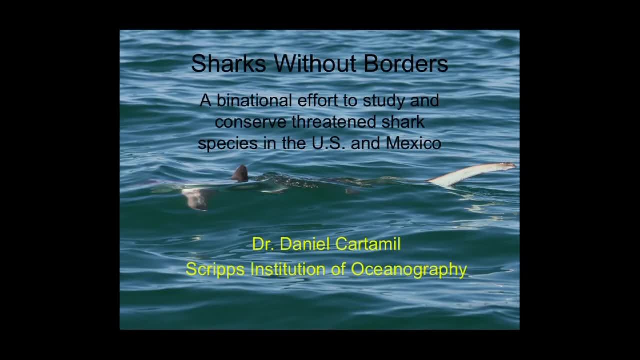 Perspectives on Ocean Science lecture. As you can tell by the title of my talk- and I wish I would have thought to bring some congas- I didn't know that that was going to come up, But the title of this talk is Sharks Without Borders. 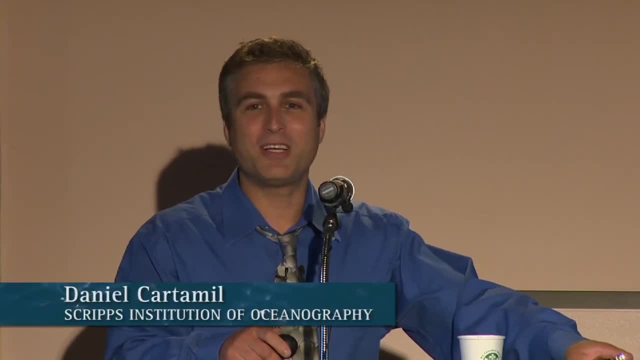 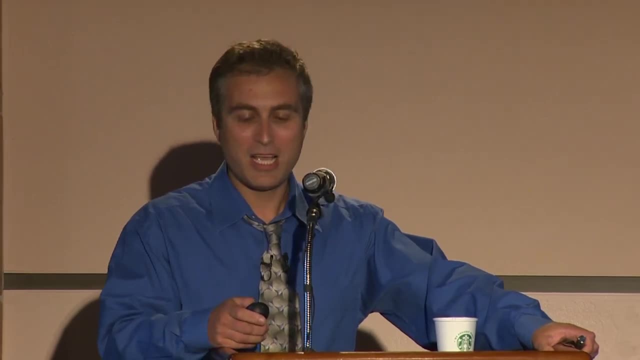 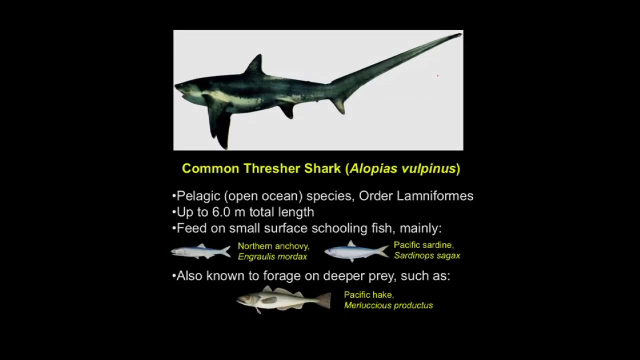 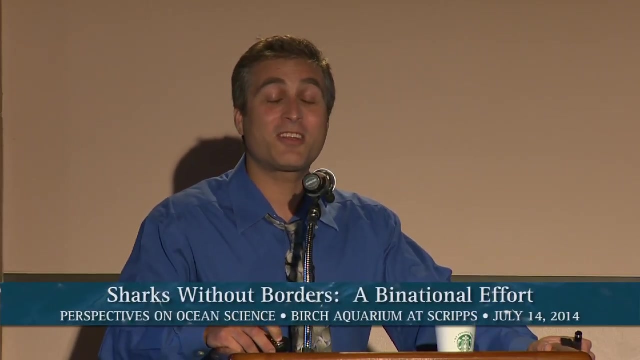 And the talk is going to cover a great variety of sharks and rays and it will cover their movements into different countries. But just to start off, why don't we go back in time a little bit, to 2004.. We're going to go back to 2004, to my starting my PhD here at Scripps. 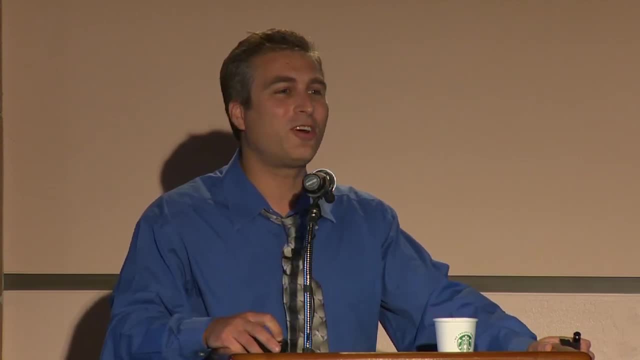 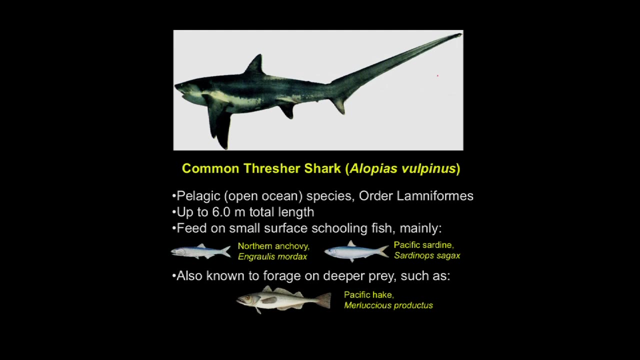 with Dr Jeffrey B Graham studying shark culture. Dr Jeffrey B Graham And I'm going to talk about a shark called the common thresher shark. The common thresher shark you see an example of up here on the screen, And this is a pelagic open ocean species. 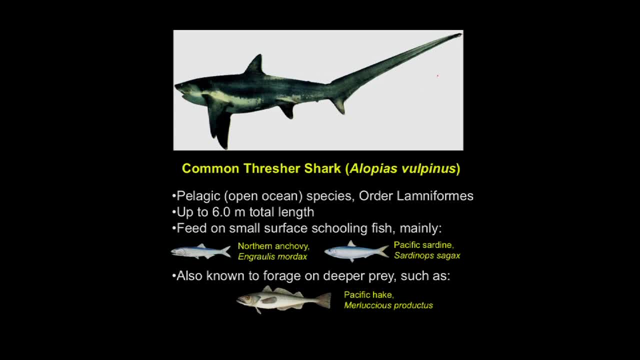 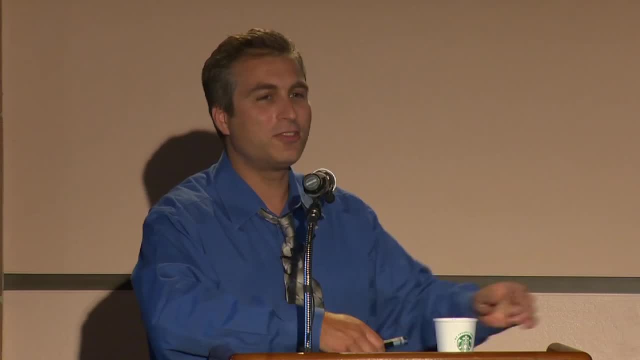 They're big sharks. They get up to about six meters. If you can't do the conversion, that's about 18 feet. So they're big animals. They're beautiful animals And you'll notice something very unique and distinct about the common thresher shark, And that is that it's got. 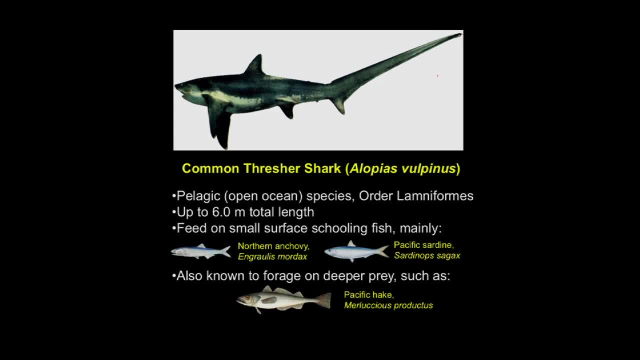 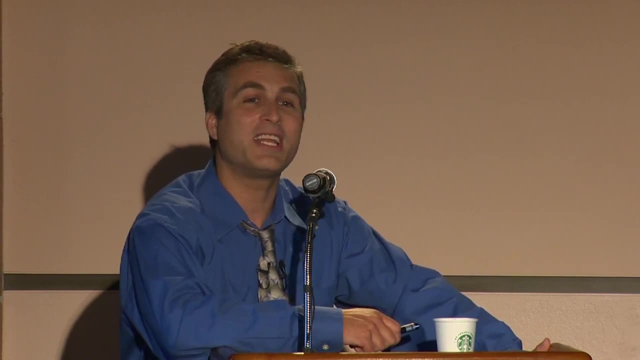 this enormous upper lobe of its tail. In fact, about half of the length of the common thresher shark is comprised of its tail, And that tail is unique also in that it's used for predation. So the thresher shark feeds primarily on schools of small fish like sardines and anchovies, And it will approach. 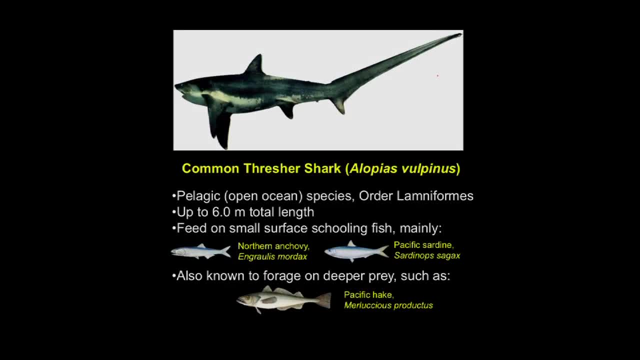 those schools, circle them and then whip the school with its tail, come back around and eat the manned and the injured. It's the only shark that really does that, But they are also known to forage on some deeper prey, like the Pacific hake, which is 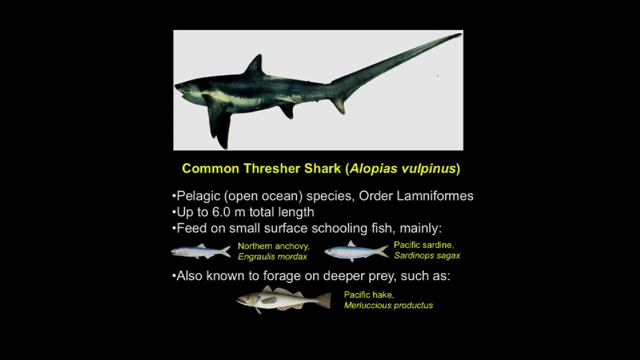 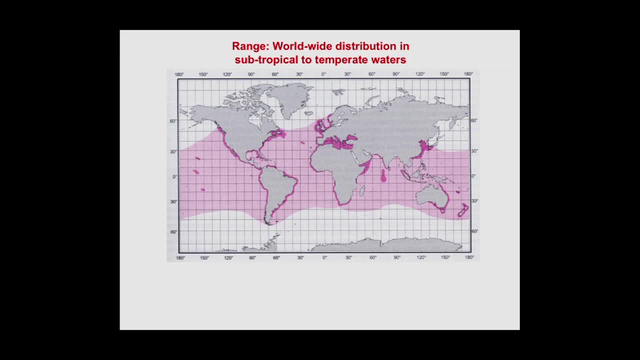 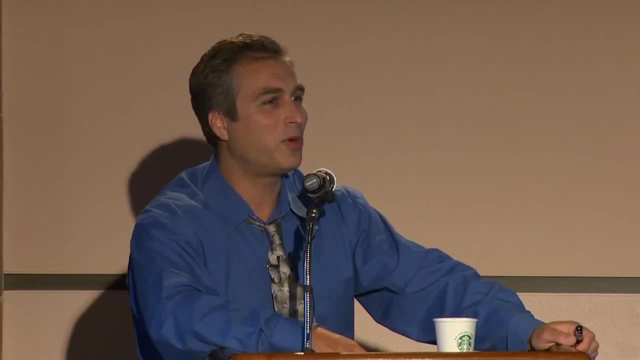 a cod-like species found offshore in deeper waters. Now, the common thresher shark is cosmopolitan in distribution, which means it's found worldwide, But it is generally found in subtropical and temperate waters. You don't find it in the most tropical waters and you don't find it. 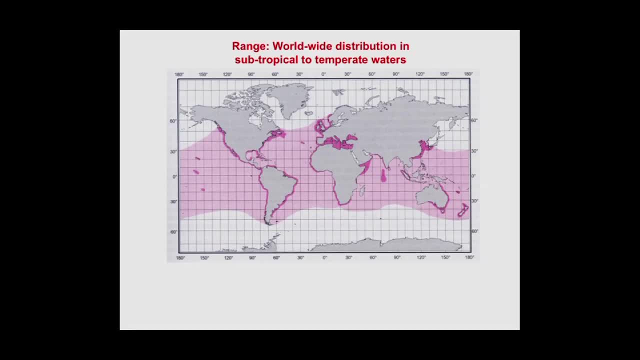 in the coldest waters, You find it in the middle. It loves waters off of California And in fact in our local waters there is thought to be one genetically distinct stock. So in other words, there's a subpopulation of thresher sharks that lives off the northeastern Pacific. 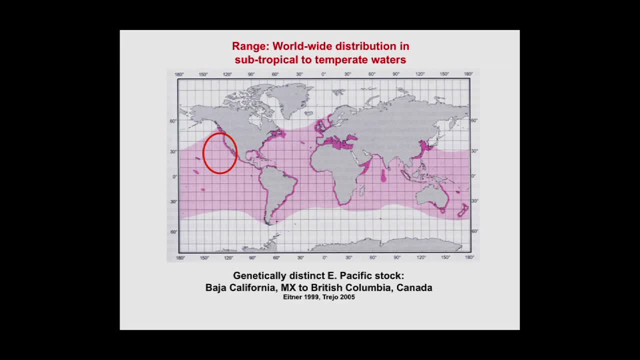 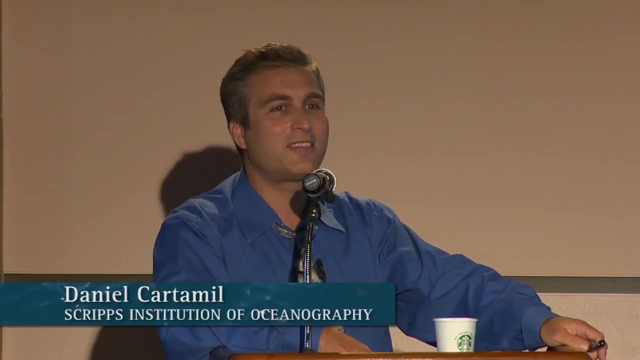 coast of North America And that doesn't mingle very much with the rest of the population worldwide. So throughout its range, worldwide, and especially in our local area, thresher sharks are exploited commercially And this is because they happen to have the really bad luck of being born as a very tasty. fish Now in California waters. the thresher shark is primarily captured in the drift gillnet fishery. This is a fishery where approximately mile-long nets are put out to sea offshore, typically around 5 to 10 miles. Those nets are a mile in length. They hang vertically. in the water column and ensnare anything that comes along. You can probably see the fins hanging out of the water column at about 8 or 9 feet deep And the water column is continuously cut off. It's really hard to see that. there's a lot. 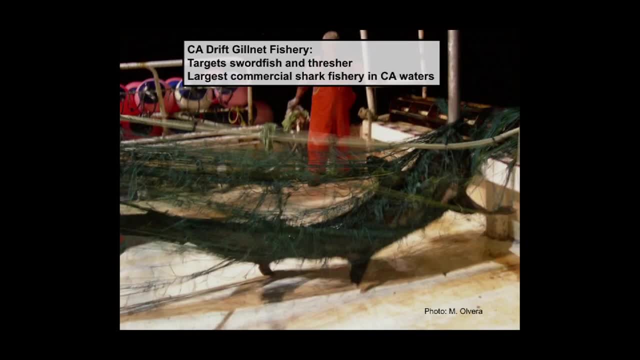 of fish in there. But if you try to see anдеvalo you can see the fish, you can see that the fish is being caught And they are in excessively thick, but you don't find that in the water column comes into the net. it's like a giant spider web and they are targeting primarily swordfish and 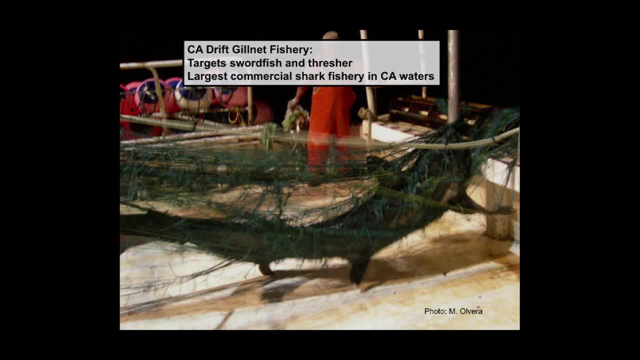 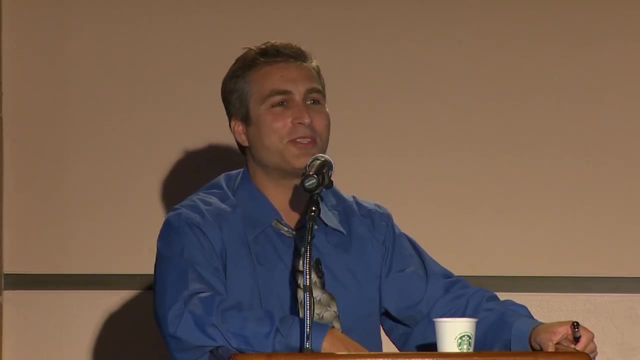 secondarily thresher sharks, but certainly thresher sharks are are a good target species for them. they sell well, and thresher sharks are the largest commercial shark fishery in california waters. however, it is shark week, and so some of you may have been watching shark programs and know that 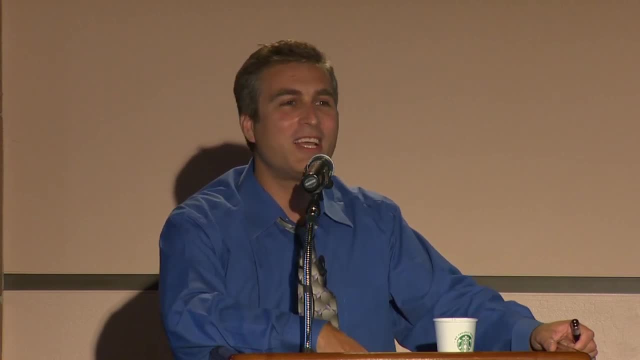 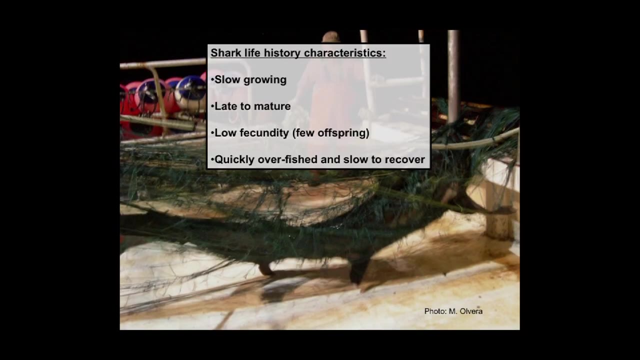 sharks have certain biological characteristics that do not really lend themselves to directed fisheries. so, for example, sharks are slow growing, they're late to mature and they have very low fecundity, meaning they have very few offspring. in the case of the thresher shark, a female thresher- 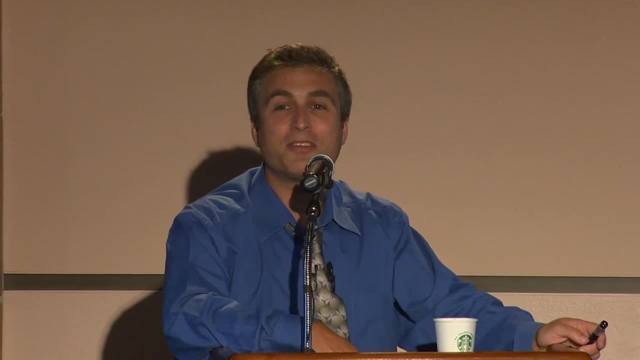 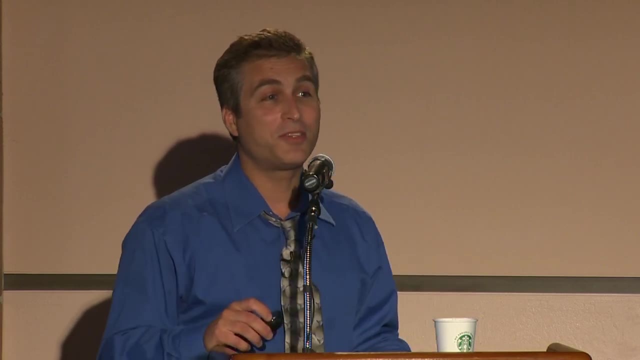 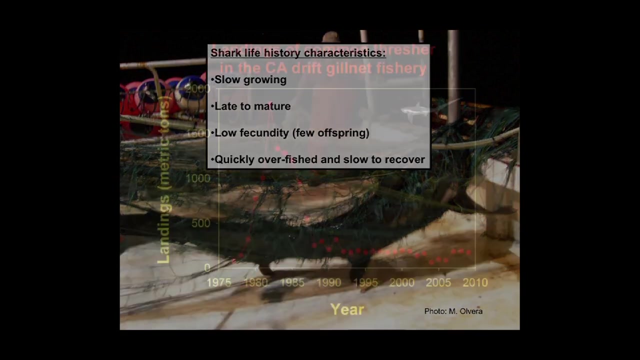 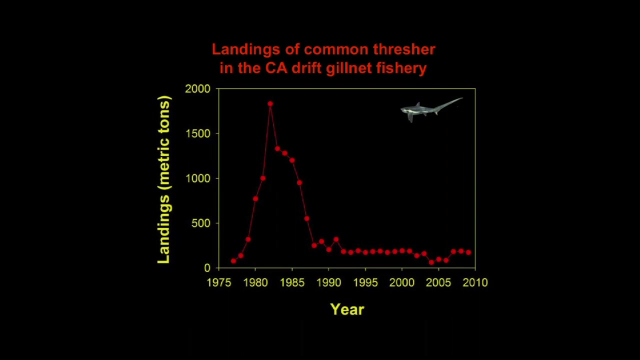 shark will typically have about three pups every other year, so very low fecundity. and because of these characteristics sharks can be quickly overpriced. and once they're over fished they're very slow to recover, even under the absence of fishing pressure. now the textbook case for this is thresher sharks in the california drift gill net fishery. so what? 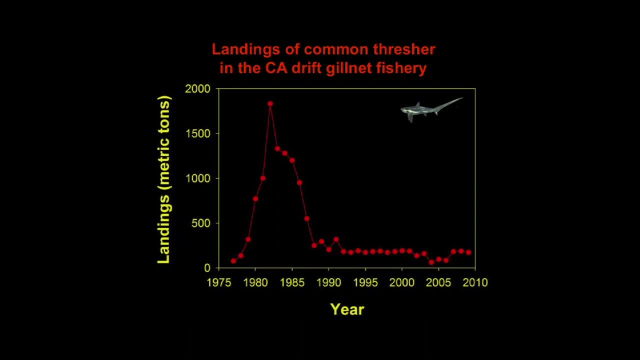 you see on this slide. here is a graph of the catch rates of thresher sharks in the drift gill net fishery since its inception in the late 1970s. you see that catch rates in 1977 were low. they increased exponentially to about 2,000 metric tons in 1981 and then they dropped just as quickly in the next five years. and since that time, they have been steady at around 200 to 250 metric tons per year. part of that is the the effects of the crash subsequent to this severe overfishing and, more recently, that the drift gill net fishery is subject to extremely stringent regulations which keep it from over. 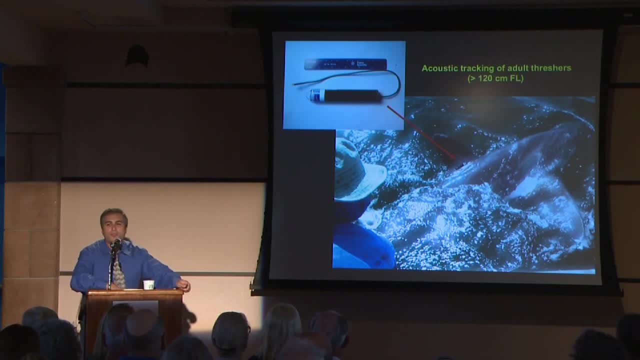 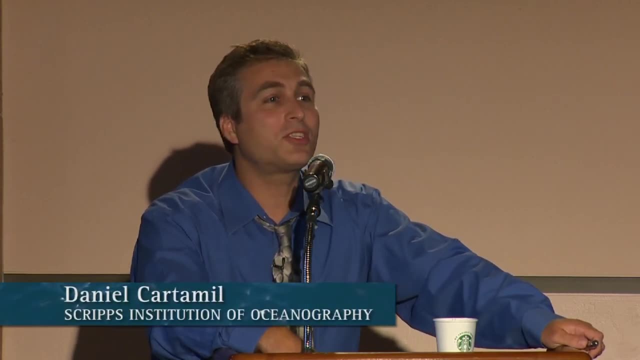 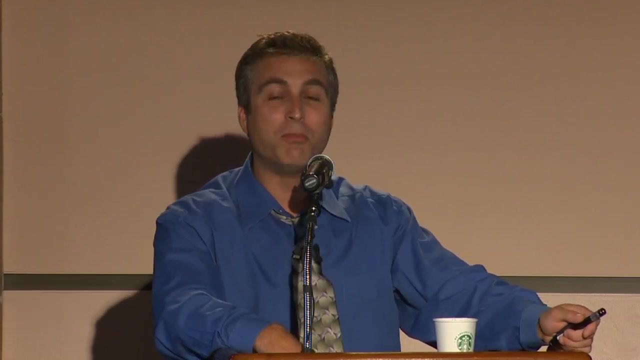 harvest. so Marsmber is the distance fishing permanent delta n and the correlation affecting the analysis is also very interesting. so when I came to- I don't know if Cheryl mentioned this, but when I came to Scripps I had just finished working for three years in the California drift gill net fishery, not 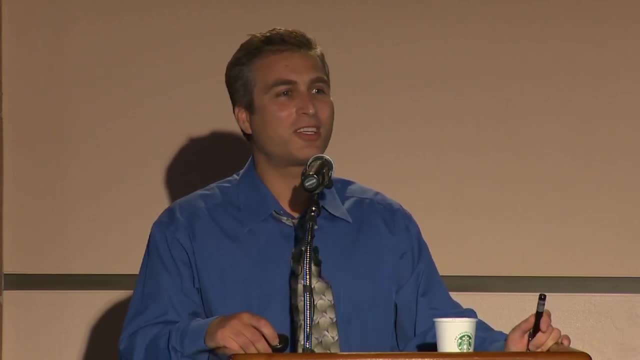 as a fisherman, the biologist aboard the fishing vessels, so I had a very strong interest in open ocean sharks and other fishes that were caught in the drift gill net fishery. when I came to Jeff Graham's lab it was specifically with the intent to the movement patterns of thresher sharks and how those movement patterns related. 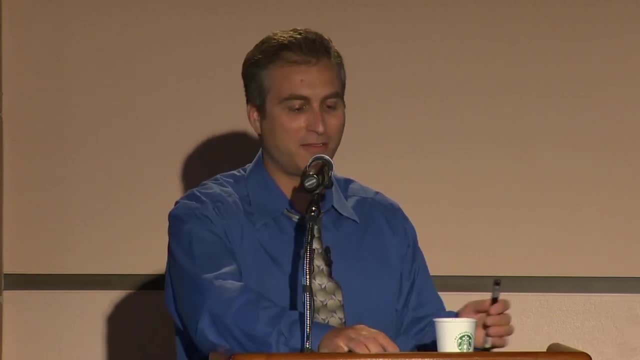 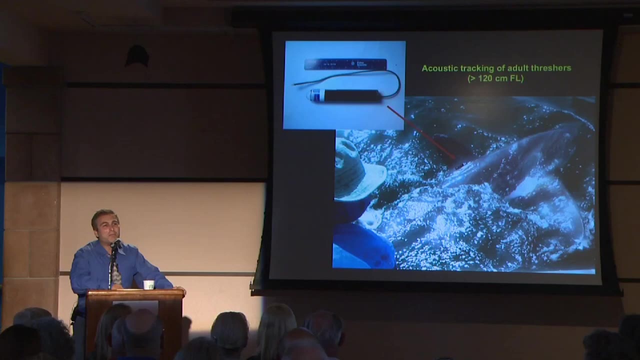 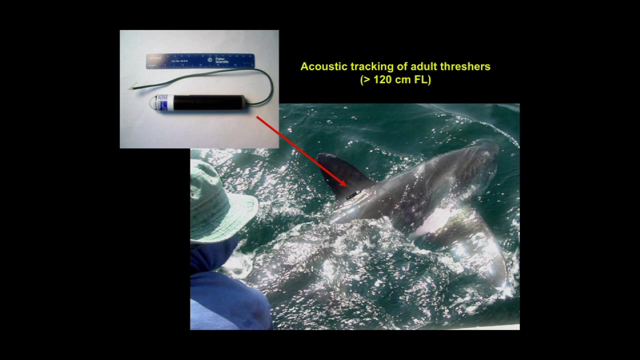 to the fishery for threshers in the California drift gillnet fishery situation. So the first thing I wanted to do was look at the movement patterns of these sharks, And the way that we did this was by using a method called acoustic telemetry tracking. 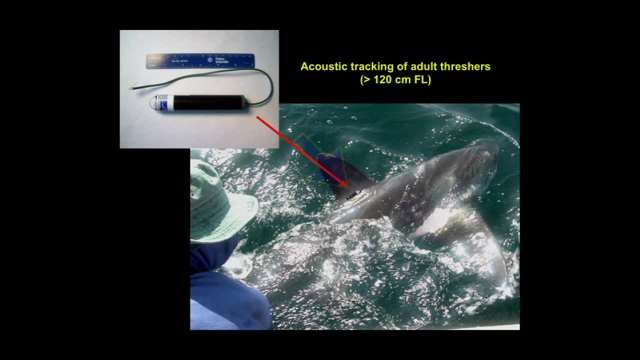 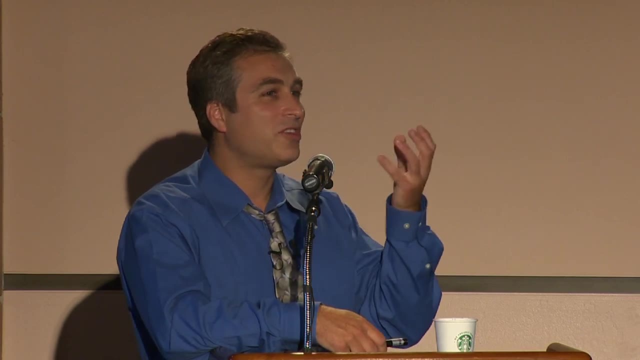 And in acoustic telemetry tracking, what we do is we attach a transmitter to the shark. The transmitter you can see here and here's a close-up of it. The transmitter has sensors which measure depth and temperature And they convert that information into an acoustic signal and transmit it in real time. 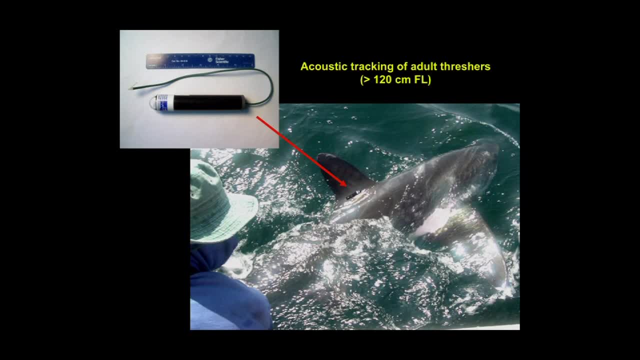 So what you have to do to track a shark like this around the ocean is: you put the transmitter on, you let the transmitter go, and then you put the transmitter on, You let the shark go and you start following it around the ocean. 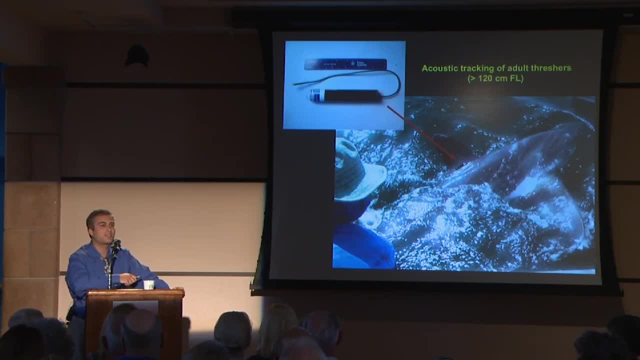 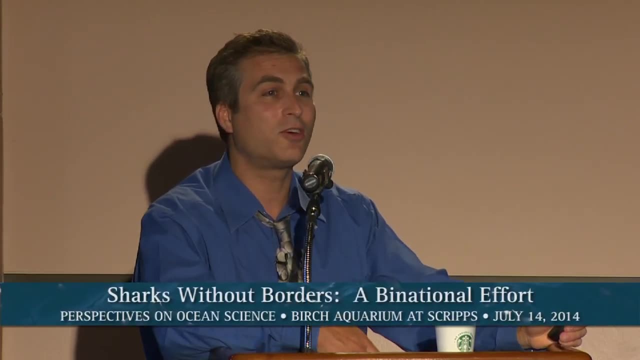 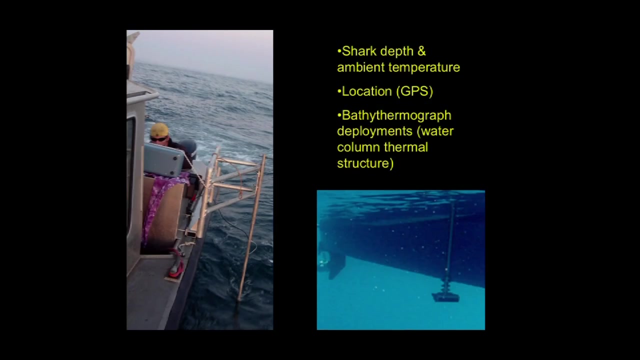 Now I should mention that the sharks we were tracking for this study were pretty big sharks. They were about three meters or so, because those are the size range of sharks that are caught in the drift gillnet fishery. Now, once you let the shark go, you can track its movements by means of a specialized research vessel. 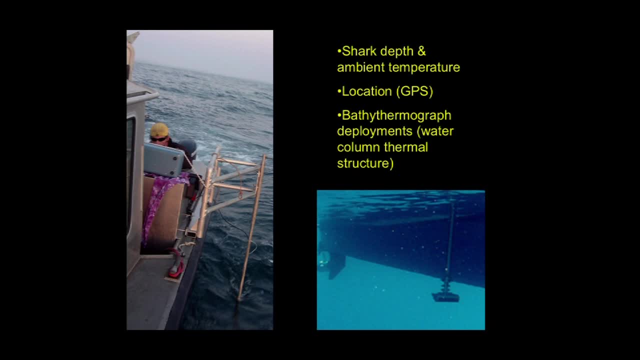 which we have here, and you can see that it has a. it has a, a hydrophone, mounted on the side of the vessel and below. so below the vessel, underneath that, you've got this hydrophone, which is essentially an underwater microphone. 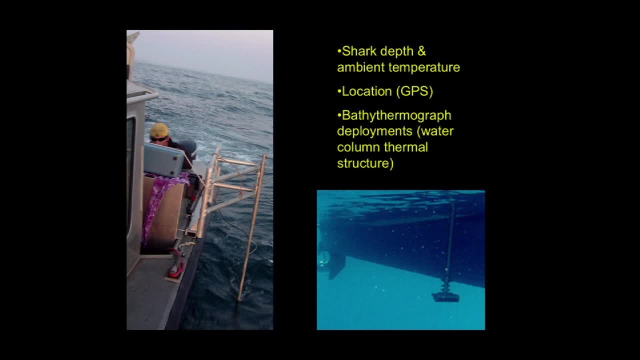 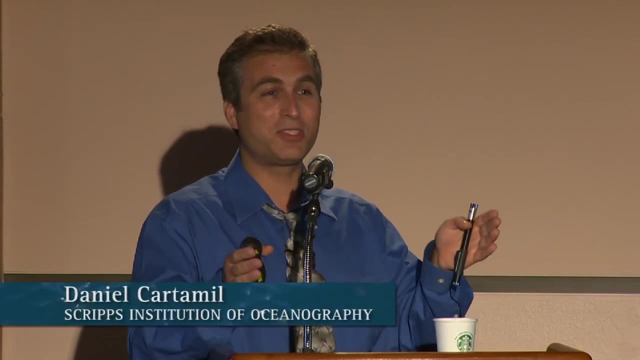 We can use that to detect the signal from the tag, and wherever the signal is strongest, that's where the shark is. So you have to follow. not too far away, so you don't have the, so you have a chance of losing the shark, but also not too close. 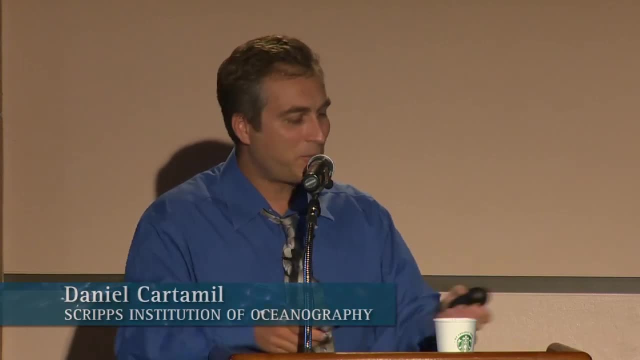 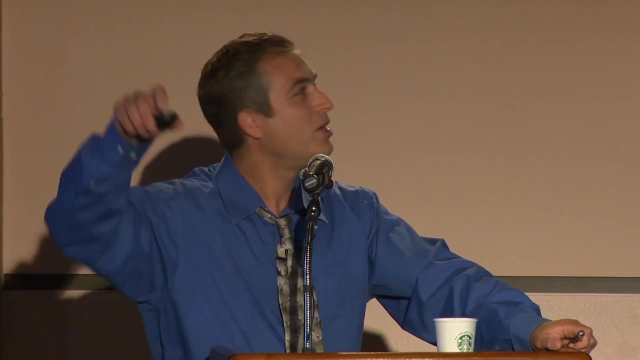 so you don't scare the shark and influence its movements. And I'm just going to show you. this is not a talk on thresher shark movements per se, so I'm not going to go into all the details, All the results from this. I just want to show you one of the pertinent results. 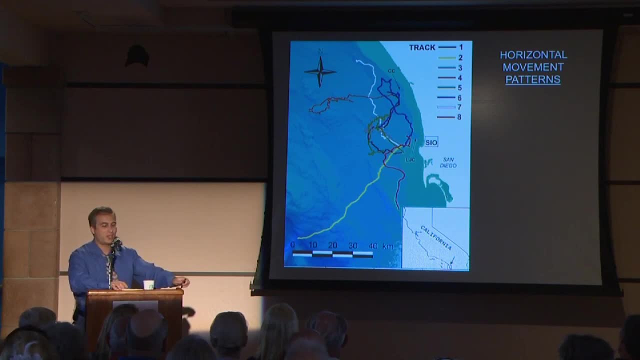 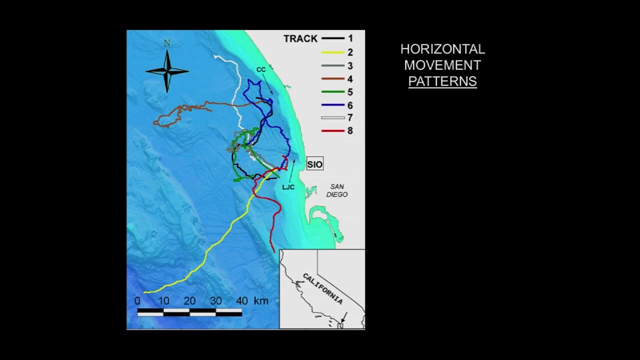 and that is the general movement patterns of these sharks. What you're looking at here is the horizontal movements of eight sharks, which were tracked over periods ranging from 24 to 72 hours. So, for example, this red line here represents a shark tracked. 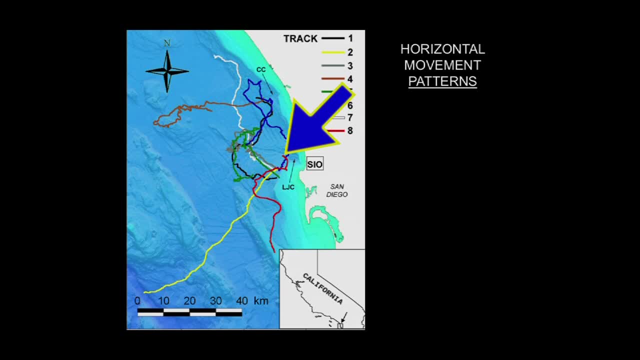 Here's where the shark was tagged, right off shore of Scripps. where we are, This is La Jolla Cove. The shark was tagged and then we followed it for about 40 hours and I think here it hit the Mexican border, so we had to stop following it. 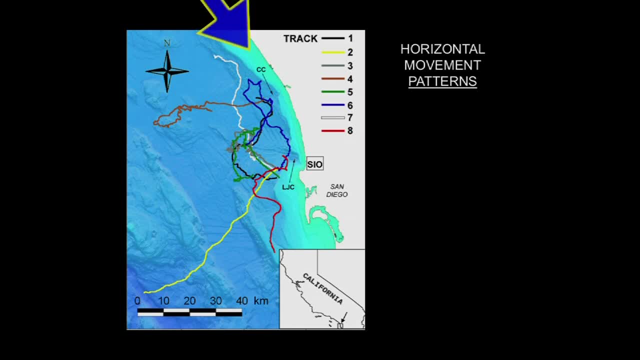 But the really salient point here is that if you look at this map you see there's kind of a lighter area close to shore. That's the continental shelf, which goes out to a depth of about 150 meters, and after the continental shelf the depth drops down to about 150 meters, and after the continental shelf the depth drops down to about 150 meters, and after the continental shelf the depth drops down to about 150 meters, and that drops off very quickly. so we've got the continental slope. 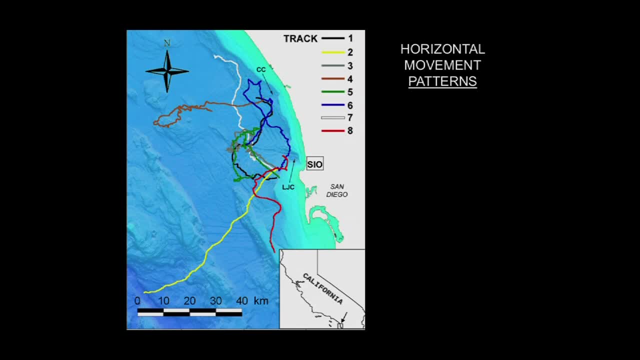 But the continental shelf is the shallow area inshore And what you'll notice is a constant pattern with all of these larger sharks. And what you'll notice is a constant pattern with all of these larger sharks is that, even though we caught and tagged them all close to the edge of the shelf- 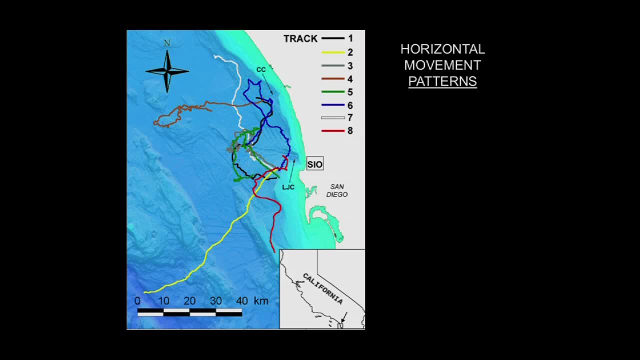 none of them actually moved over the shallow waters of the shelf. So we see that adult thresher sharks of the size range caught in the fishery have a very strong preference for waters offshore of the continental shelf. have a very strong preference for waters offshore of the continental shelf. 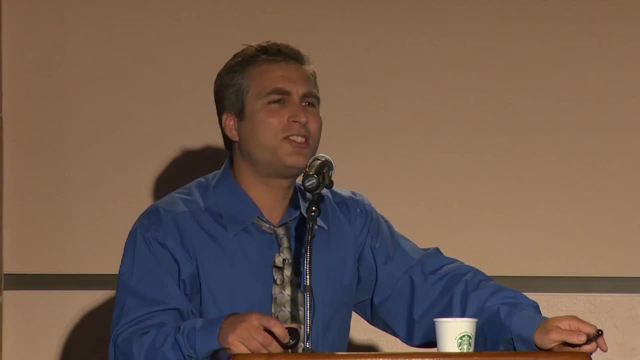 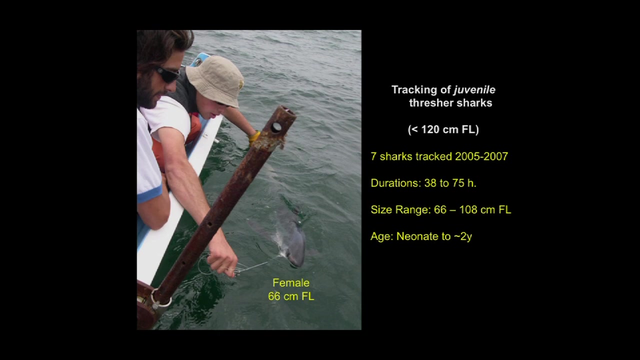 Now, that was all very interesting, but as a biologist, we were very interested in looking at the complete life history of this organism, And that includes trying to find out what the juveniles were doing, because if you look at the catch records of the drift gillnet fishery, you don't see juvenile sharks being 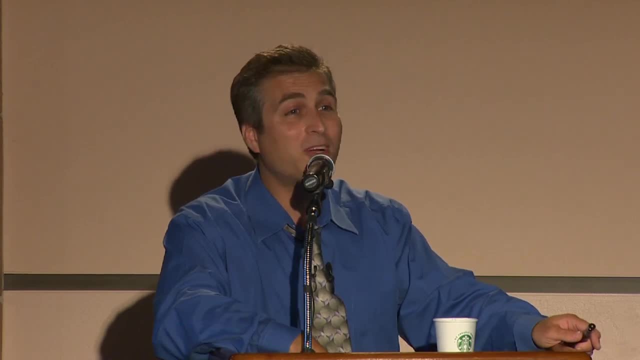 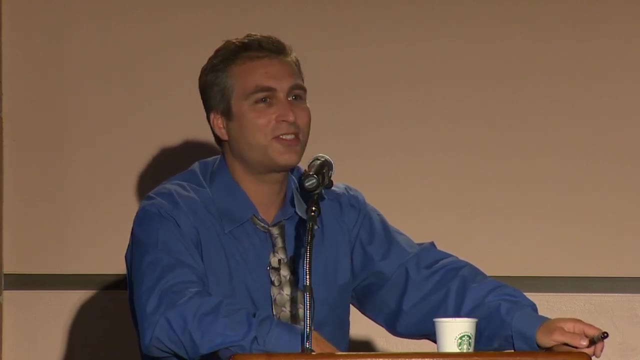 caught in the drift gillnets. So there must be somewhere else where the adults aren't. So we spent a couple of years. it was a long two years, I'll tell you. it took two years to catch seven of these things. 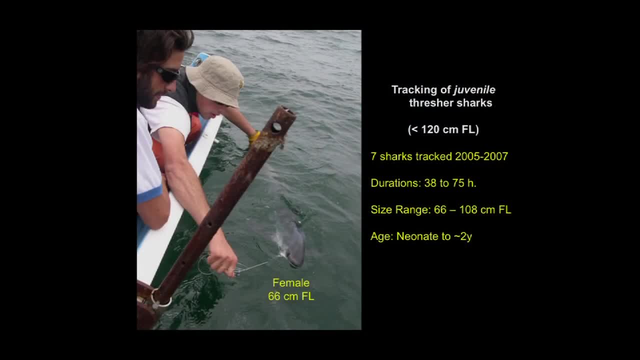 And again we tracked them with acoustic tags for up to 75 hours, and now you can see the difference in size. This is a very small shark- That's actually probably the smallest one I've ever seen- And we were interested in what the habitat differences are between the adults and the. 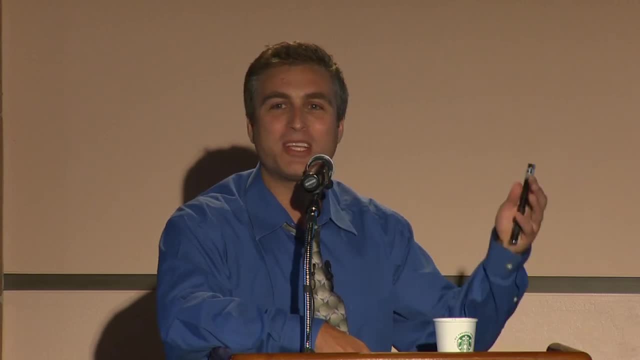 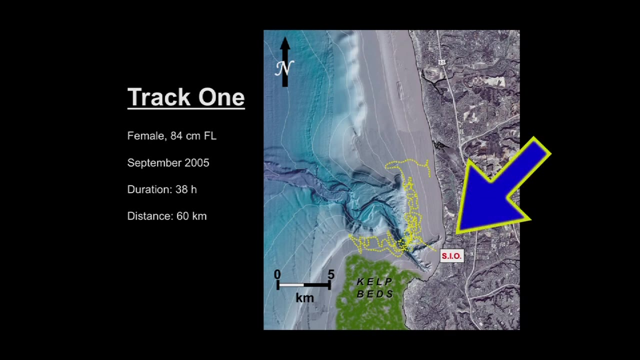 juveniles. I'm just going to show you one track, A representative track. They're all pretty similar. So here on this juvenile shark track. what you see is we're here at Scripps, This is the continental shelf, And the movements of the shark are in yellow. 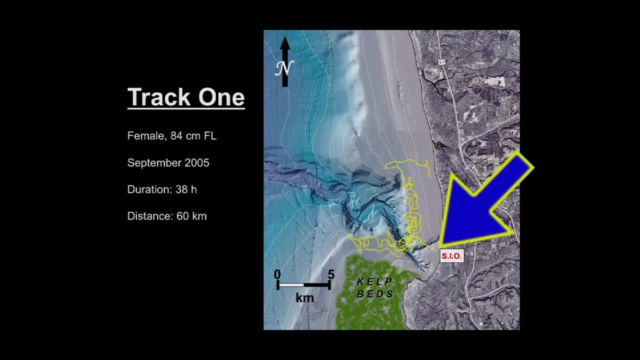 The shark was tagged just offshore of Scripps, just off of Scripps Pier, and for 40 hours it meandered in the area in front of Scripps and we finally gave up the track around Blacks Beach. But what you notice here is that this shark 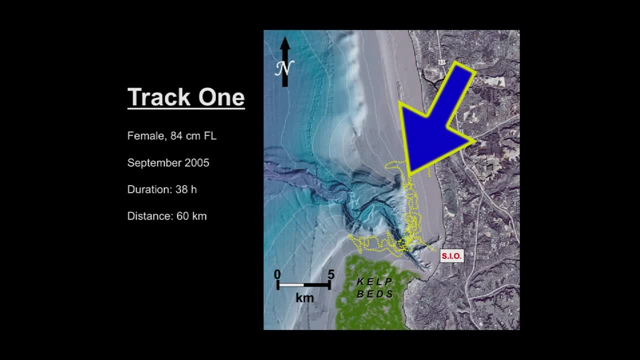 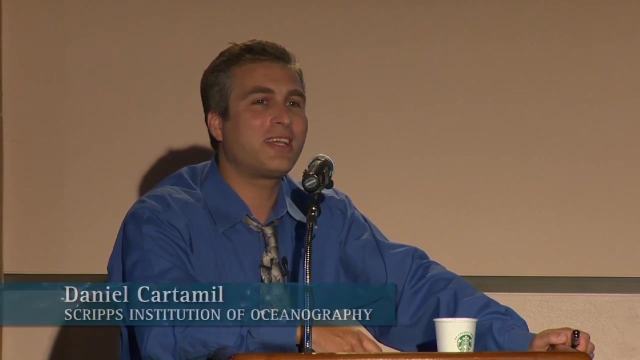 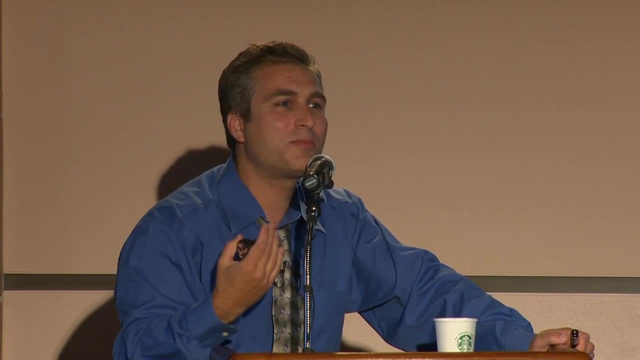 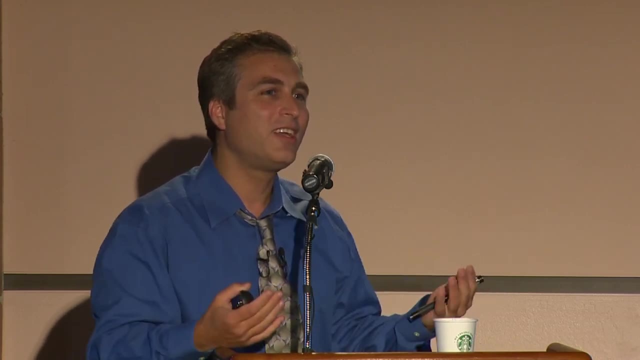 nursery area What that means in terms of shark biology. sharks are known to have nursery areas. A nursery area for a shark is a place where the young spend the first year or two of their lives. It is a place that provides ample resources and 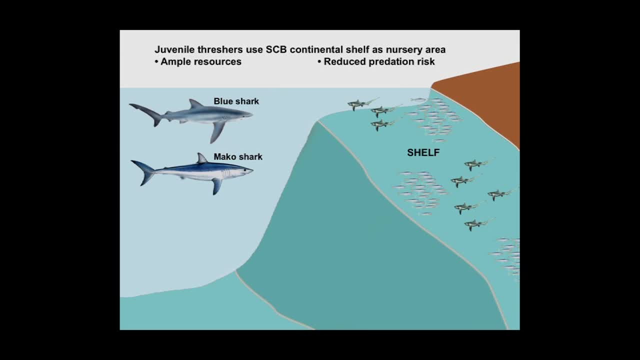 typically provides some reduced predation risk And in the case of thresher sharks, you can imagine how being offshore in the same habitat as the adults would be very dangerous, because there's adult blue and mako sharks that could prey on them, And if you're a thresher shark, 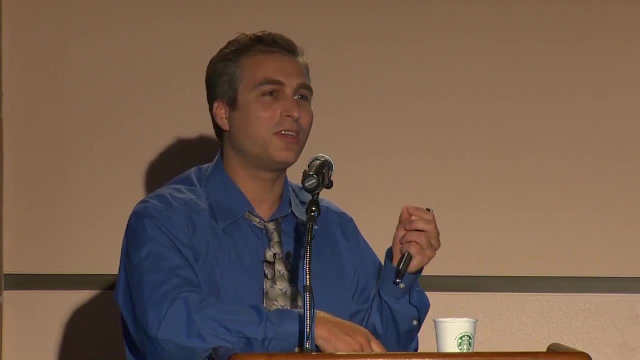 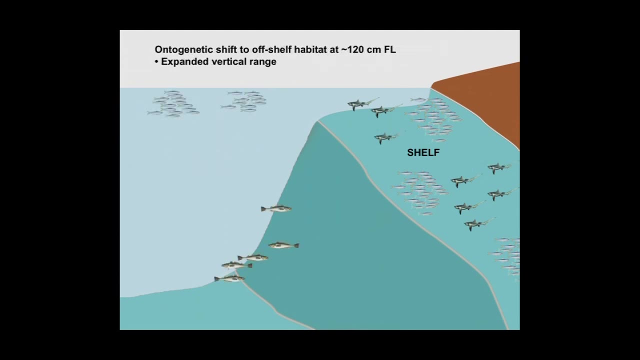 which only has two to three young every other year. you can afford very little juvenile mortality. So we've got these sharks that are living over the continental shelf as a nursery habitat until a size range of about 120 centimeters fork length. Once they reach 120 centimeters, they move off shore. 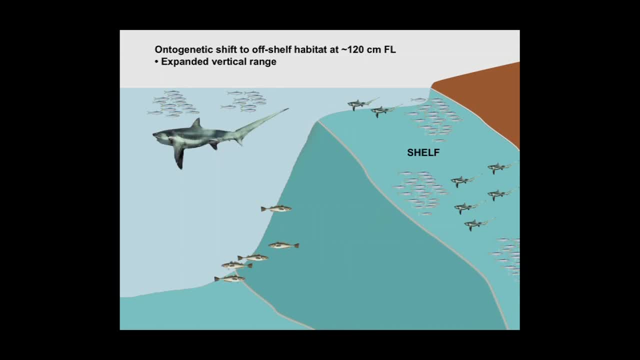 and then they go back to their natural habitat, And then they go back to their natural habitat, And then they go back to their natural habitat, And then they go back into the same habitat as the adults. This affords them the same access to. 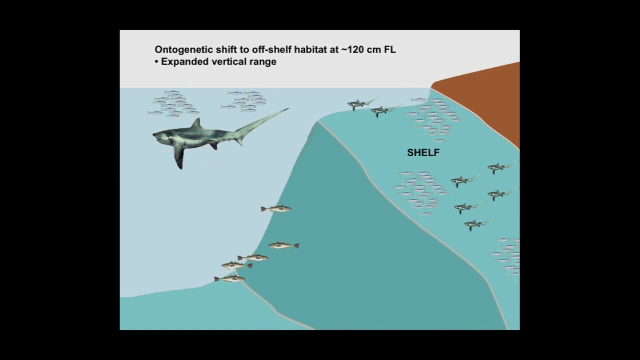 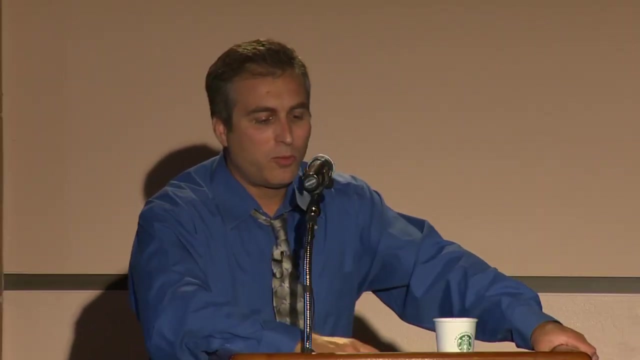 prey. because they're near the edge of the continental shelf. There's still a lot of sardines and anchovies, But once they're there they greatly expand their vertical range and they typically spend a lot of time during the day diving to two to three hundred meters to feed on fish such as Pacific hake. So we were 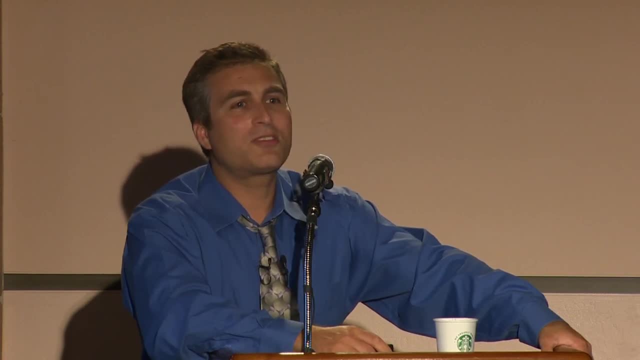 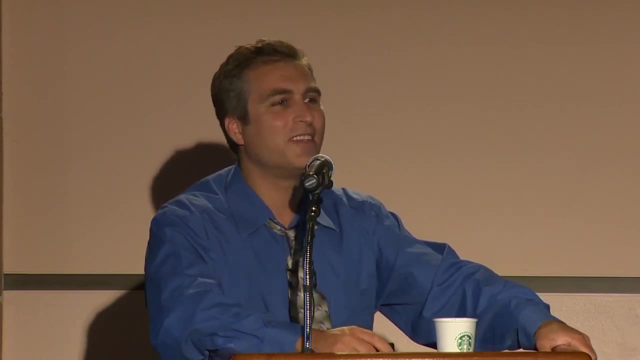 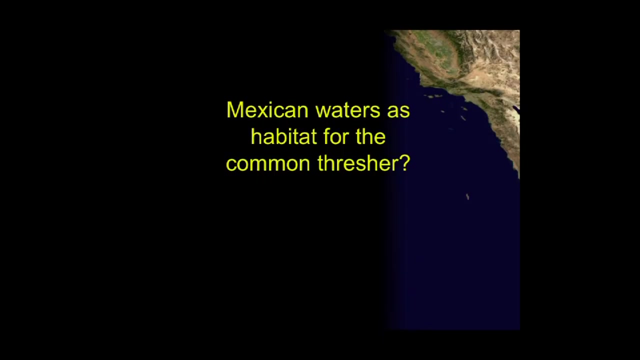 learning a lot about thresher sharks through acoustic tracking studies, archival tagging and so on and so forth. Other researchers in California and Central California have studied their diet and their age and growth, But what occurred to us as I sat in the office talking with Jeff was that all of these studies had taken place in 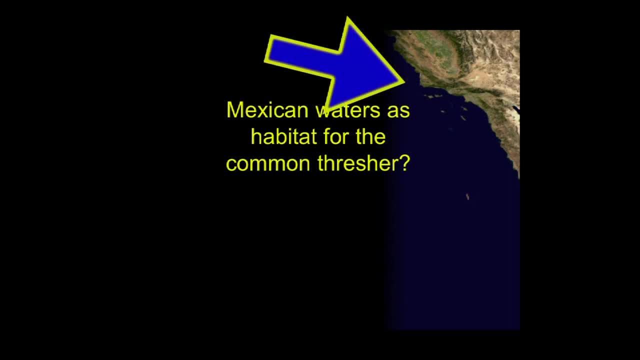 Southern California, But essentially from Point Conception, which is just north of Santa Barbara, to the US-Mexican border, And this is an area which is typically known as the Southern California Bight. The Southern California Bight has long been thought to be one of the most dangerous species in the world. It's a 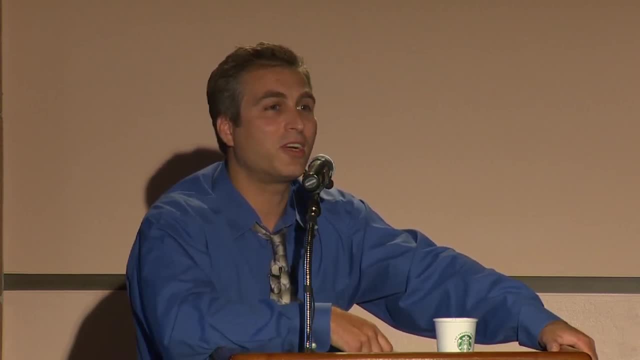 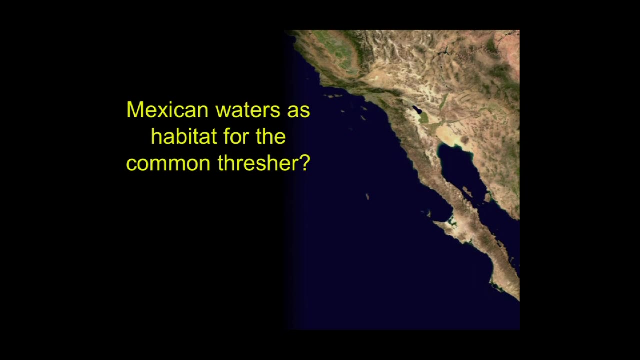 species that is known to be the greatest area of concentration for thresher sharks based on fishery records, And so it's the most well studied. However, we came upon a very interesting question, and that was: why wouldn't sharks move into Mexico? It? 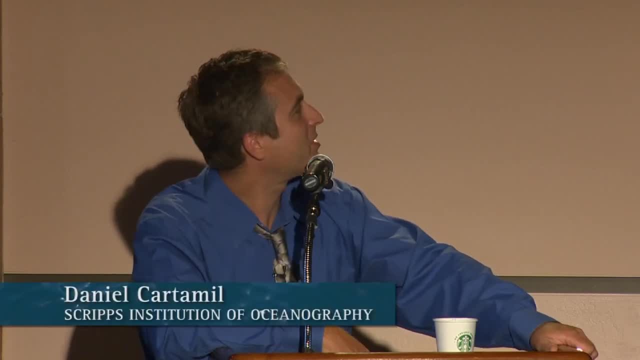 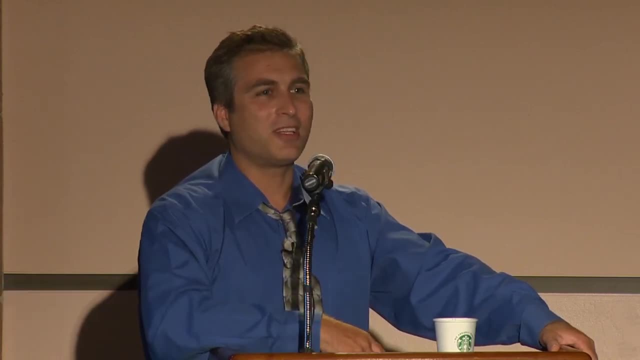 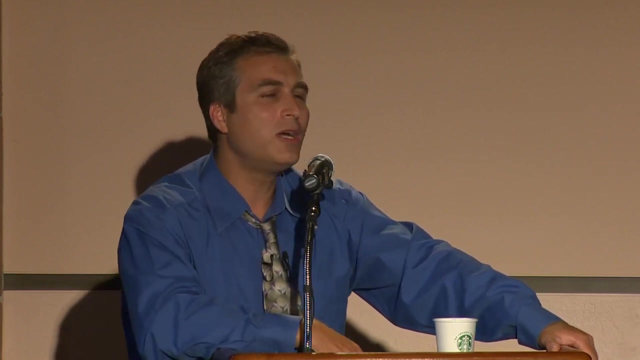 seemed obvious that they would. I mean, we tracked them right down to the Mexican border And this is an important question, not just biologically. We're interested as biologists in the life history of these animals and where they spend certain times of the year and whether they migrate into Mexico. 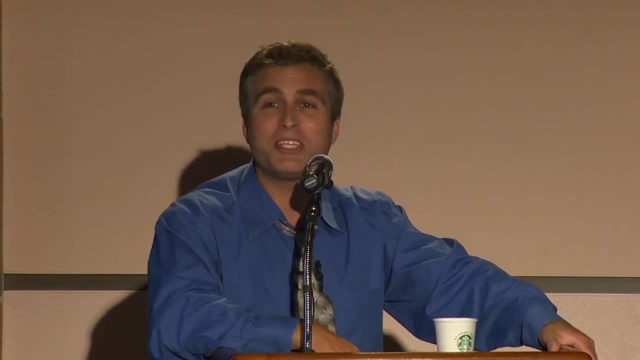 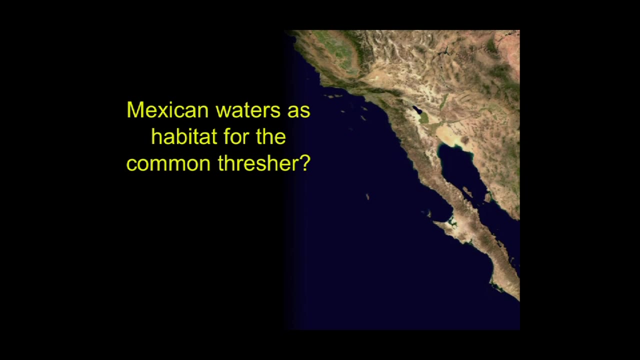 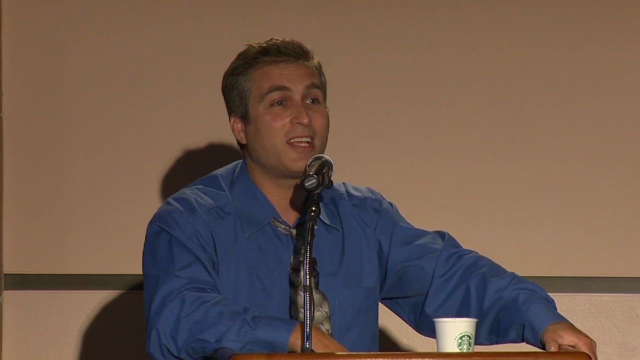 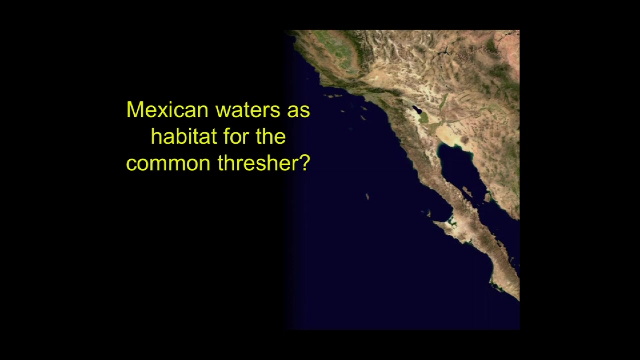 But from a fishery standpoint it's very important information because we think that they're harvested sustainably at this point in the United States, But if they move into Mexico and are harvested in great numbers, that could be a very problematic and unsustainable situation. So we were interested in whether these 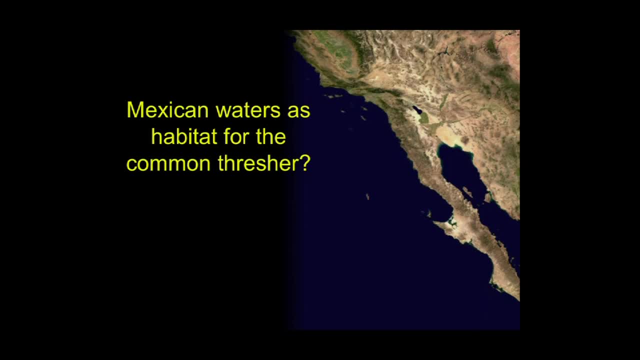 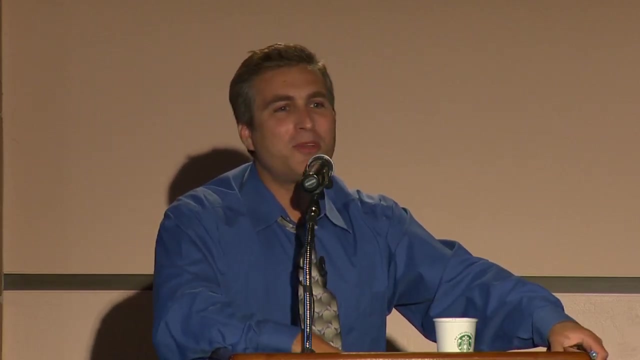 sharks moved into Mexican waters, and specifically waters offshore of the Pacific coast of Baja California. So we began a study to figure out whether Mexican waters were in fact habitat for the common thresher shark. So how do you go about doing that? Well, one way is to. 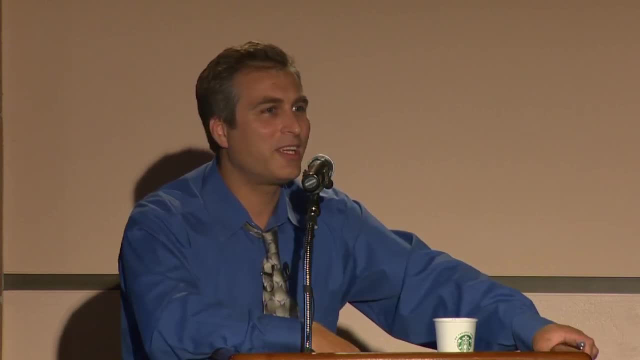 go around fishing forever and trying to catch thresher sharks and see where they are, But that's not very efficient. The easy way is to simply go to the fishermen that are fishing there already and see what they're catching. It turns out that there 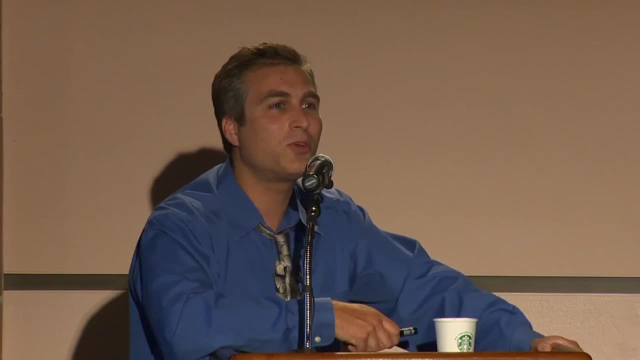 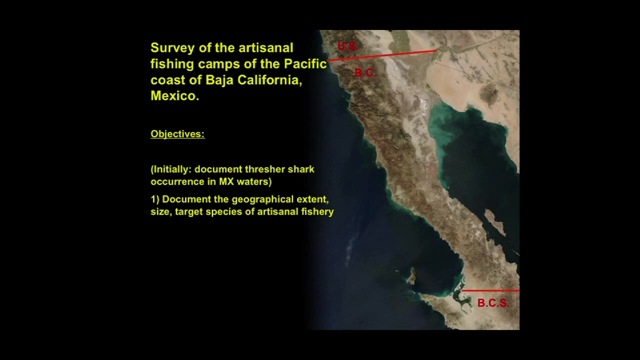 are there. in northern Baja California there is only one big commercial port- that's here in Ensenada, and none of the commercial fishing vessels that were there were targeting thresher sharks, So that wasn't very a viable option to look at thresher sharks and their distribution. However, what we did learn, 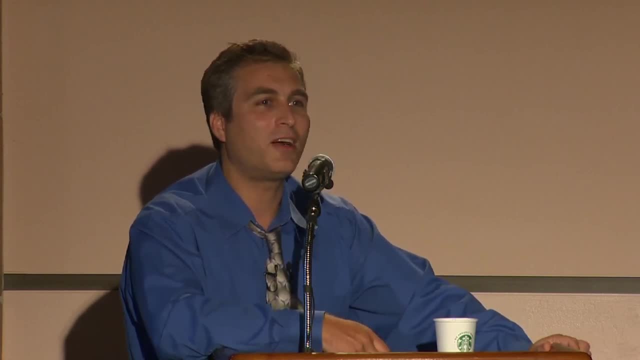 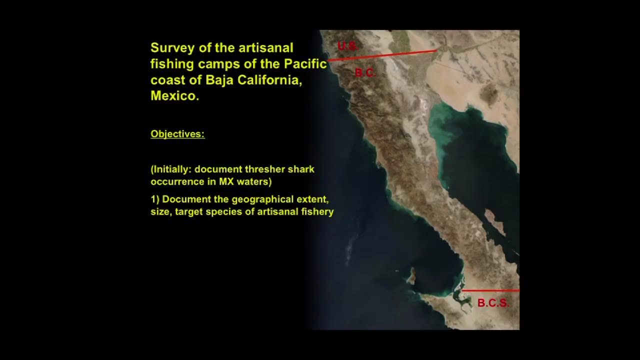 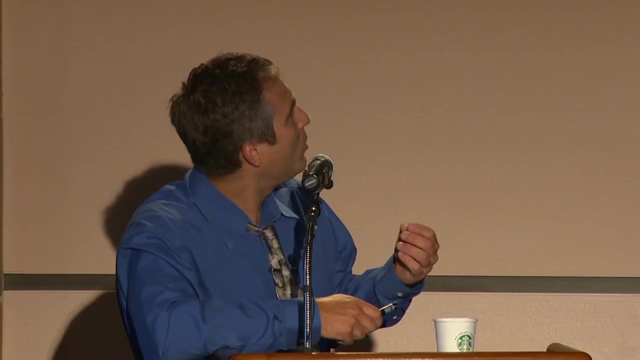 through our preliminary investigation was that there was a network of artisanal fishing camps that were scattered along the Pacific coast of Baja California. Artisanal is a word that means small-scale, traditional, when it's referred to fisheries. So what? we devised a plan to survey all of these. 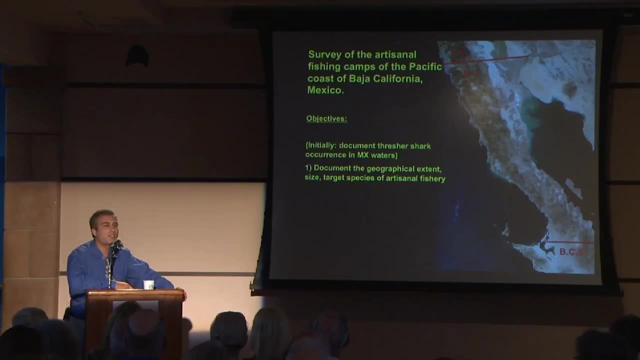 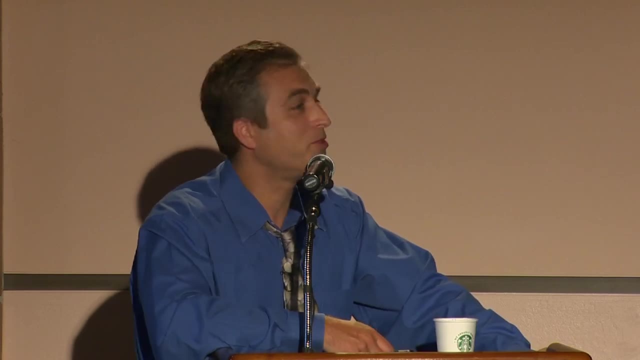 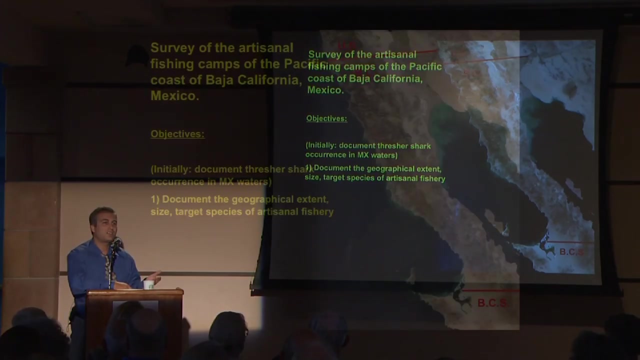 artisanal fishing camps. Prior to this study, nobody knew how many camps there were, how many fishermen were employed there, what they were fishing and what gear they were using, And so this was really unknown territory. So we set out to describe these artisanal fisheries, but also with an eye towards documenting. 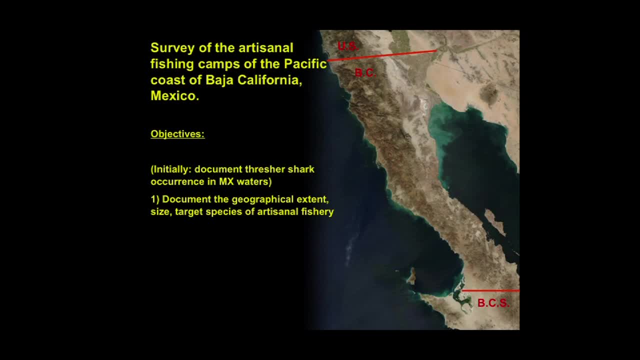 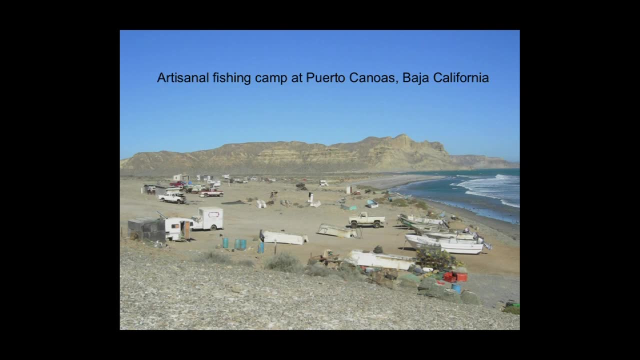 thresher shark occurrence and seeing what that told us about thresher shark biology in that region. So if you don't know what an artisanal fishery is, this slide gives you an idea of a pretty typical artisanal fishing camp. This is at a place called Puerto Canoas. 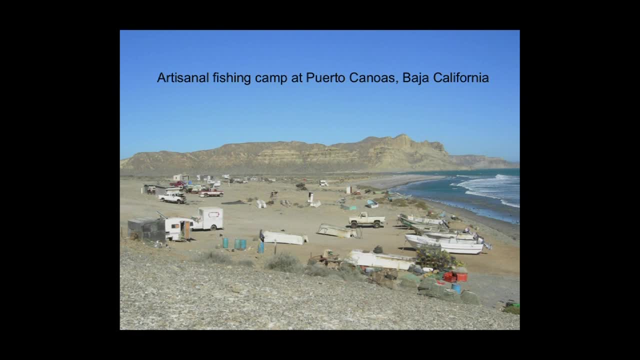 It's in the central part of northern Baja And it's pretty typical. It's really hard to get here. You have to go down about two hours down a really bad, steep, rutted, dirt road to get to this place And it's very remote. Consequently, these artisanal fishing camps. 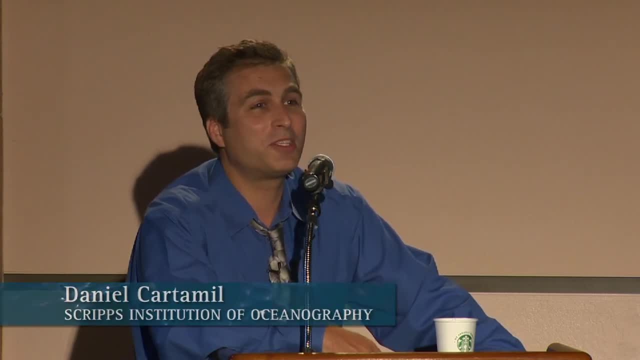 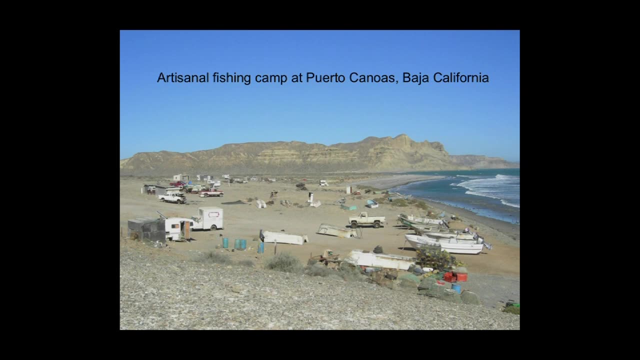 have been very little monitored and historically pretty much unregulated, But this is very typical. The boats that are fishing out of these artisanal camps are these small vessels which are called pangas, And the fishermen are there sometimes and sometimes they're not. It's a seasonal thing and the 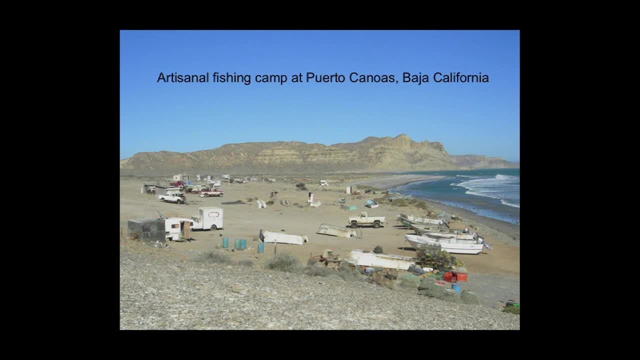 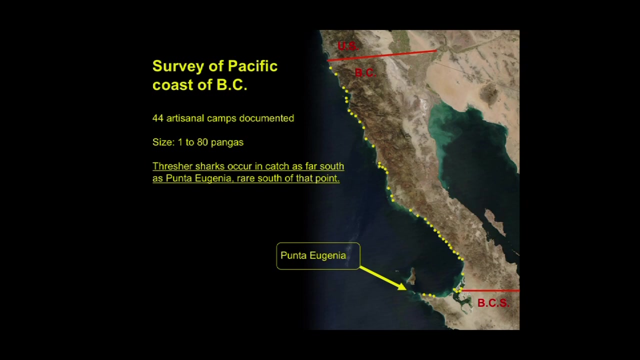 fishermen move from camp to camp. They stay in these little plywood shacks or sometimes in little converted, dilapidated campers. It's a whole different world down there. So we spent a couple of years traveling up and down the Baja coast, the Pacific coast of Baja, And I just want to, actually just for in. 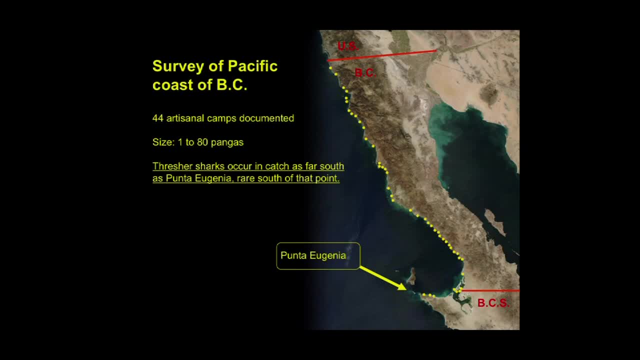 terms of terminology, let me just mention this: The Baja California Peninsula is actually two states: The state of Baja California and to the south is Baja California Sur. So it's a little confusing because most people call the whole peninsula Baja. This is the state of Baja and what I'm 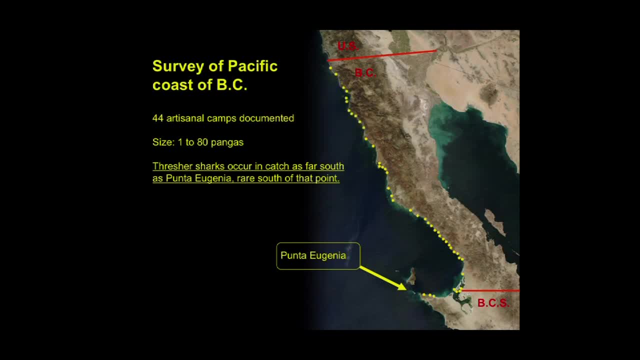 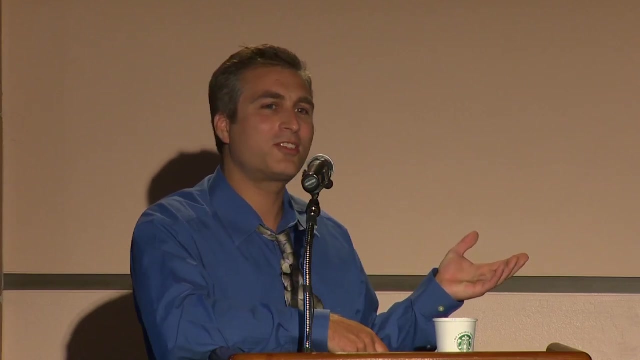 referring to right now is the Pacific coast of the state of Baja California. We found that there were 44 artisanal fishing camps along the coast, most of which targeted sharks and raised at least seasonally. And interestingly, what we found as far as thresher sharks was that thresher sharks were 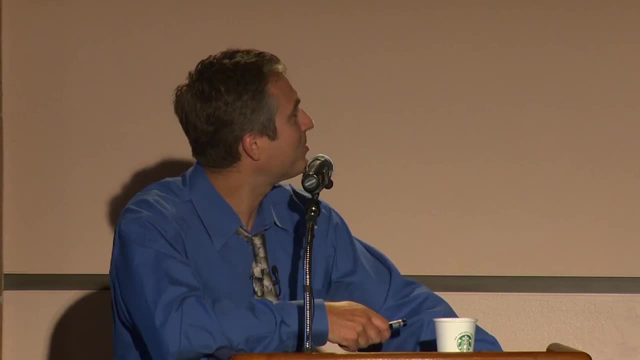 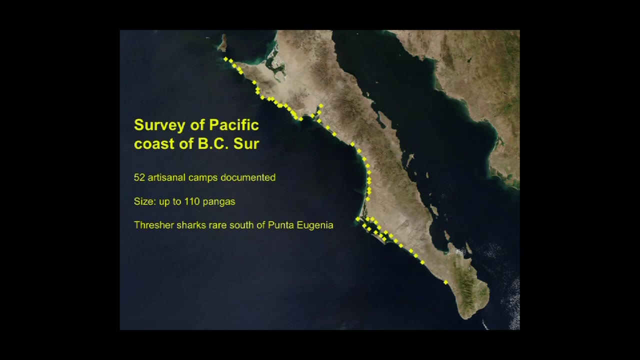 being caught in all of those camps, sometimes in great numbers, And this study was conducted all the way up until this point here, which is called Punta Eugenia. We found thresher sharks all the way up to that point. We received a grant subsequently to survey the artisanal 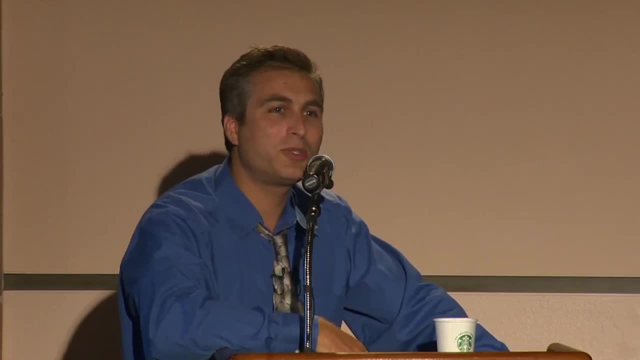 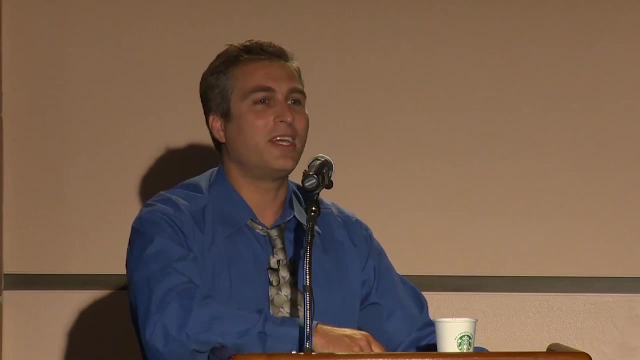 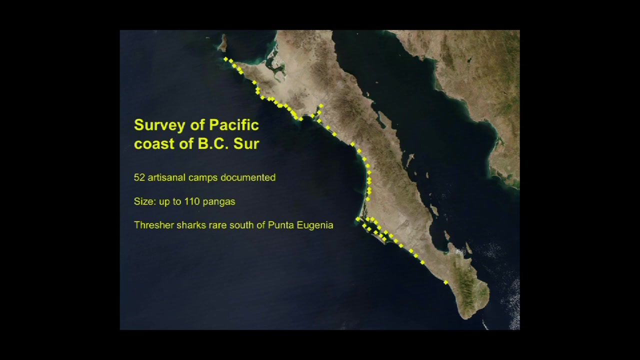 fishing camps in southern Baja California, And so we spent a couple more years doing the exact same thing, running up and down the coast to every conceivable inch of coastline, And we found 52 artisanal camps in Baja California Sur. These camps were a little bigger generally. 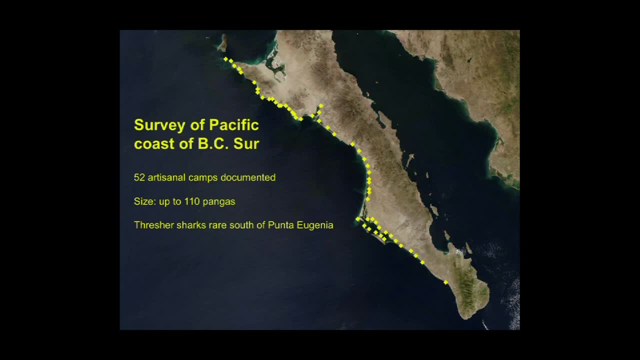 speaking, than the ones in the north, typically about 20 pongas per camp, the largest one being 110 vessels. And interestingly, with regard to thresher sharks, we found that south of Punta Eugenia, here, there were no thresher sharks coming up. There were a couple here in a place called. 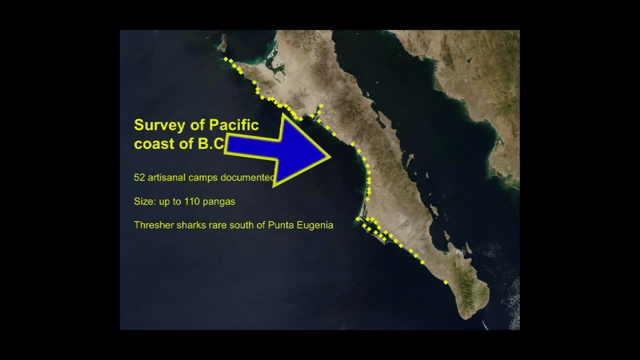 Bahia, Tortugas, but we didn't see one thresher shark there, And so we went down the rest of the Baja California Sur Pacific coast. So this began to paint a very clear picture for us of what the distribution of these sharks is. It is in the northern half of the Pacific coast of Baja California, But more than that. 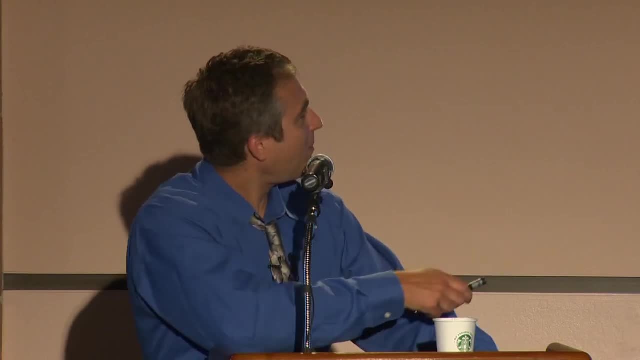 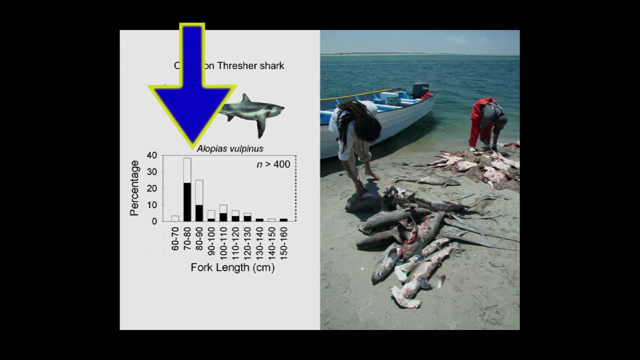 the size range of the sharks that we're seeing was very telling. If you look at this diagram, it shows you the size distribution of the sharks that were, Of the thresher sharks, Of the thresher sharks that we were seeing in these camps. they're essentially all less. 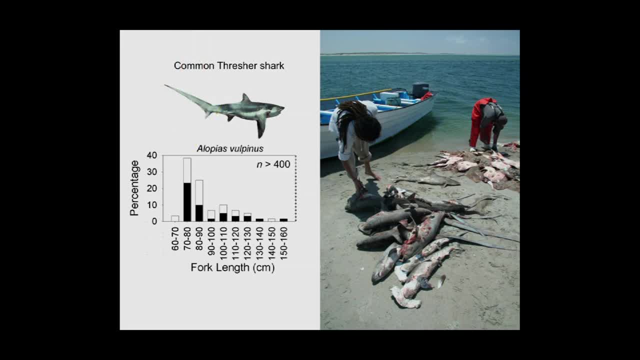 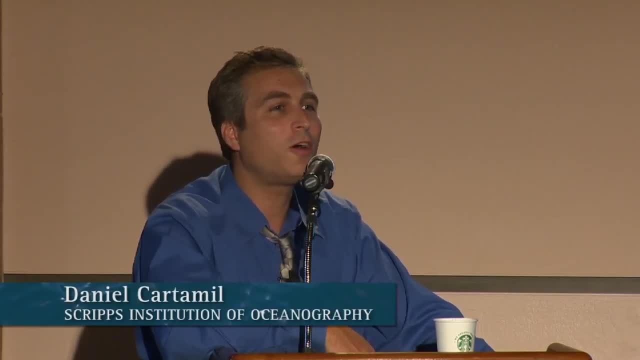 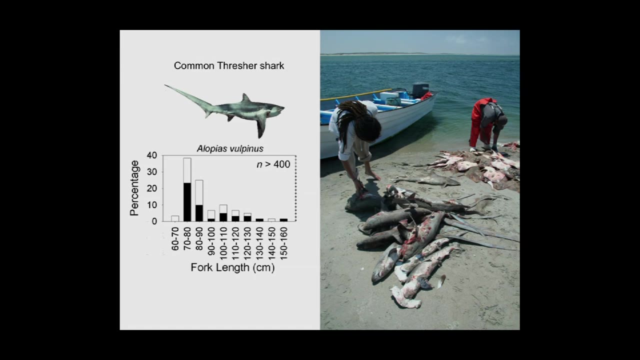 than a meter in length. So what this indicates is that these artisanal fishing camps are catching thresher sharks to as far south as central Baja. All of the sharks they were catching are very immature, so they're fishing in the nursery area, And that's significant. 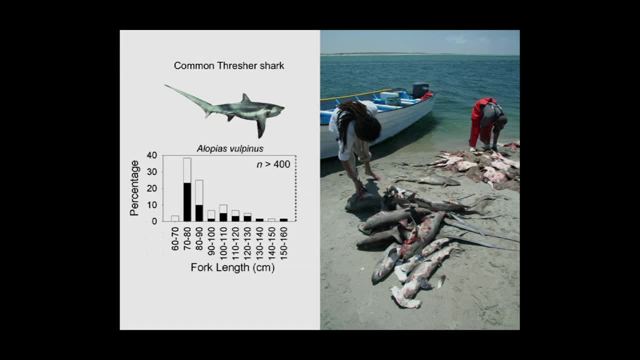 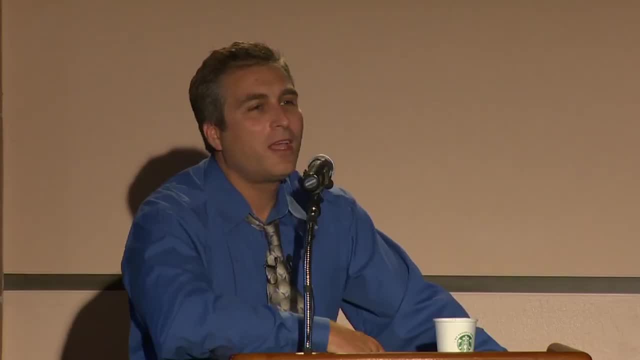 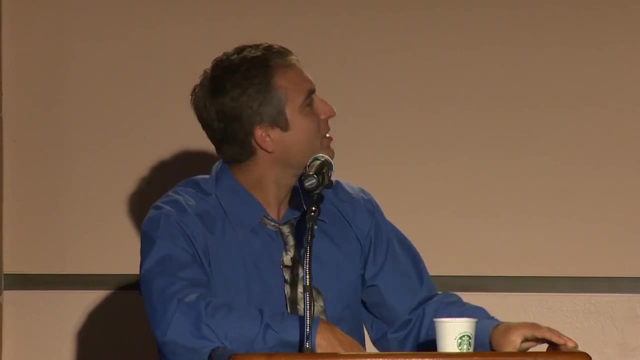 because, of course, juvenile thresher sharks are sexually immature, They haven't yet had a chance to reproduce and contribute to the sustainability. So all of this is showing us the potential for the survival and sustainability of the population. Now concurrent with this study, we were- I was- down in Baja about a week every month. 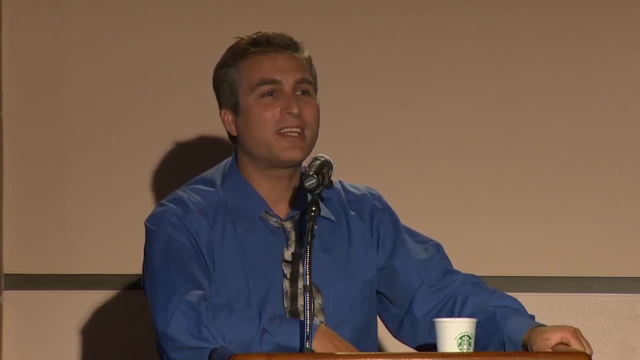 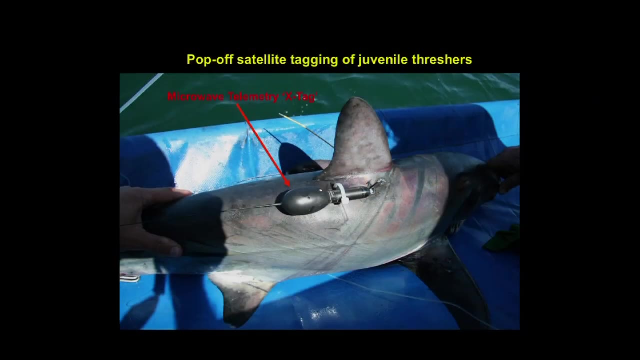 for several years And when we were in Baja, I was up further north satellite tagging juvenile thresher sharks. So this is a different study. Up from San Diego to LA to Santa Barbara- we were going up and down the coast- We found a much better method of catching thresher sharks. 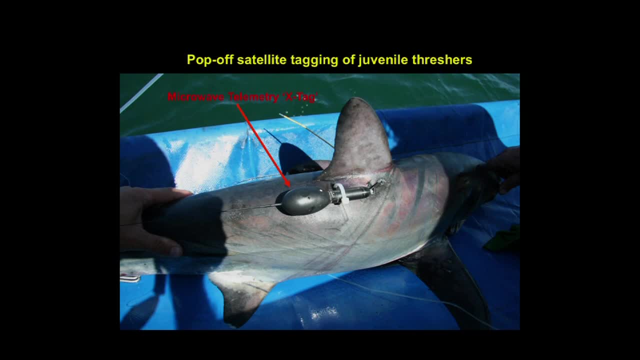 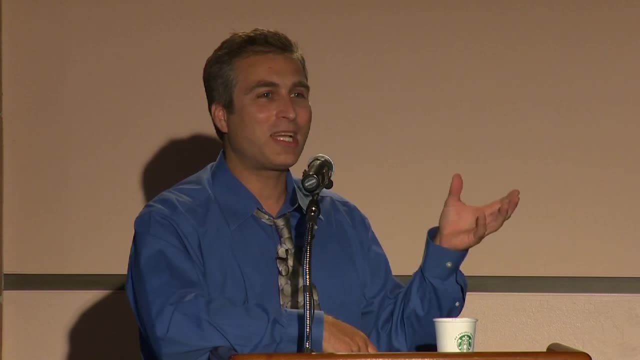 which was to let a commercial fisherman do it for us. we would catch the fish, we would catch the sharks and outfit them with a different type of tag. This is a pop-up satellite tag. Now, this type of tag is different than the acoustic tags I showed you before. 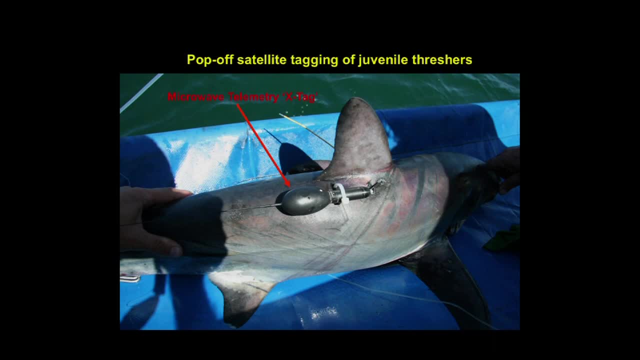 It has the same sensors- depth and temperature- and it also takes note of the location of the shark. But what happens in this case is you tag the shark and you let it go. Six months later, the tag pops off of the animal. 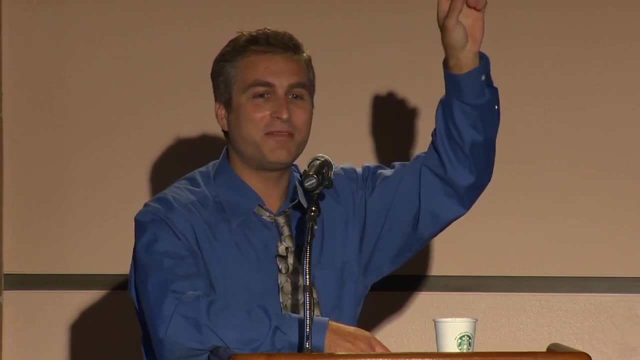 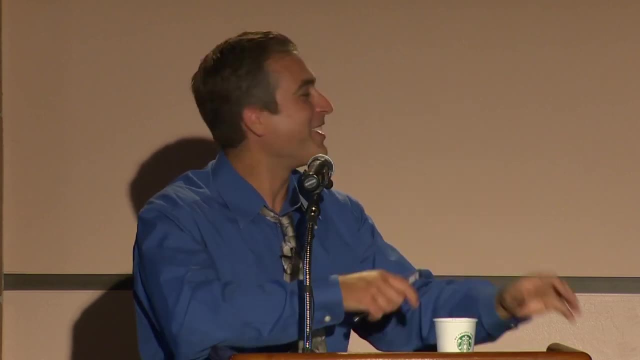 floats to the surface and transmits all of its data via satellite to my personal email account, And I sit there at my desk saying, hey, this is great, So you get a huge amount of information, the trade-off being you don't get as fine-scale resolution. 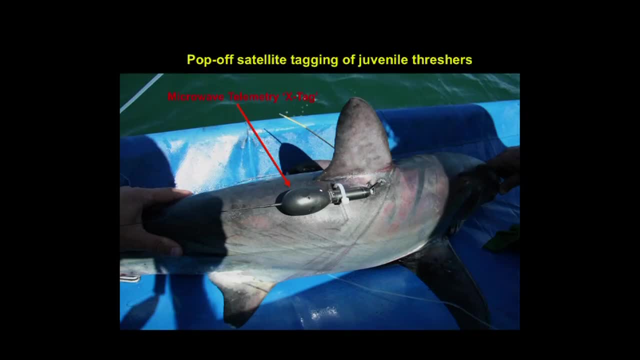 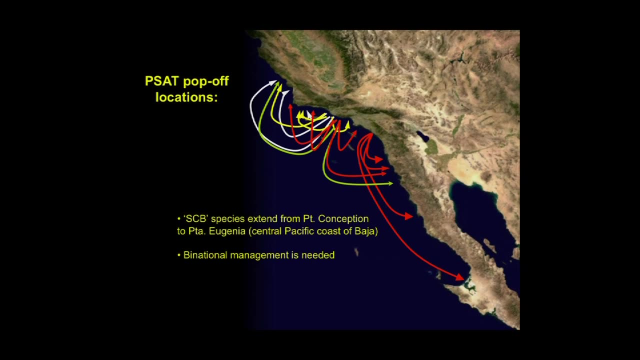 and it's much more expensive. And again, that would be the subject of a whole other talk. but I just want to show you the one pertinent result to this talk, which is that the sharks were, they were all tagged in the Southern California Bight. 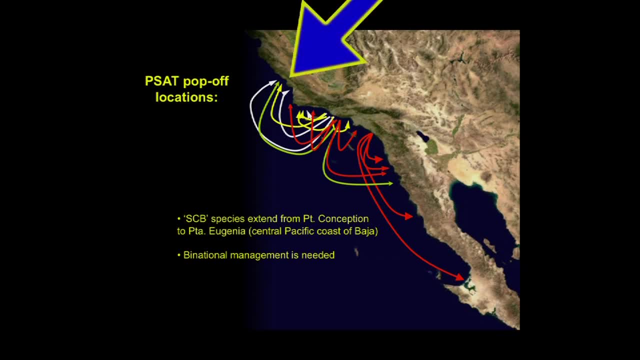 and a lot of them stayed in that area. Some moved just north of Point Conception, but we saw quite a bit of movement into the waters offshore of Baja California to as far south as Punta Eugenia. So these results were pretty much the exact same. 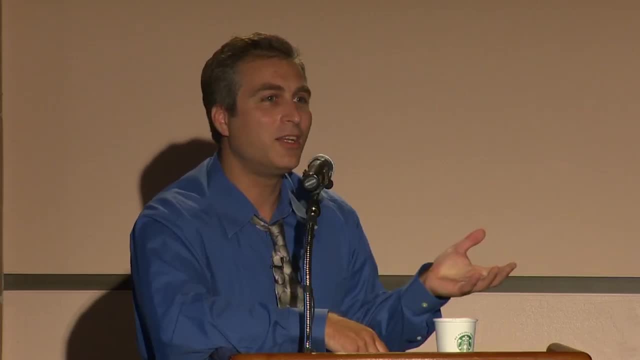 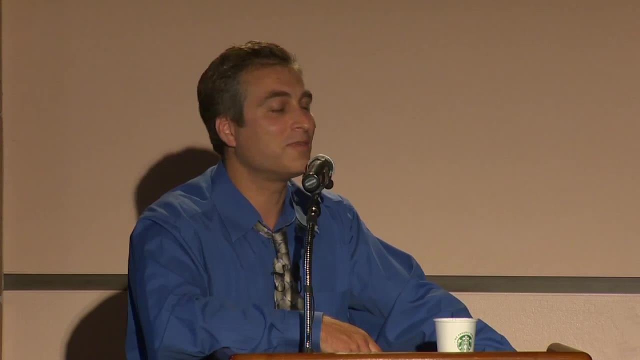 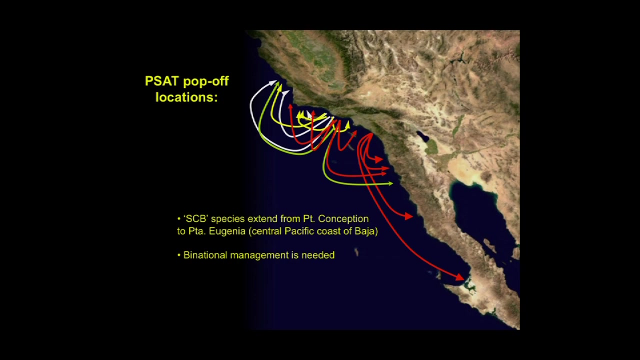 as what we saw with the artisanal fishery and really validated what we thought we had learned about the geographic range of juvenile thresher sharks On the Pacific coast of North America. And what it also tells us is that, much like many other species that inhabit Southern California waters, 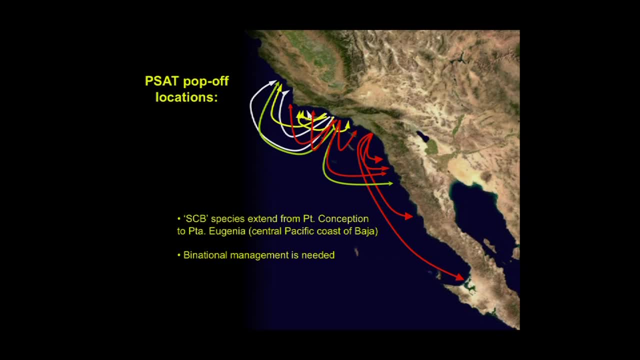 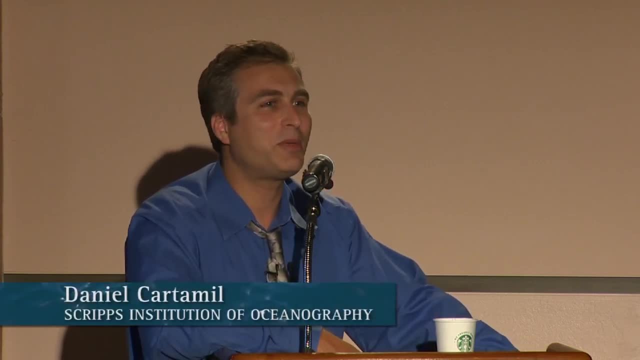 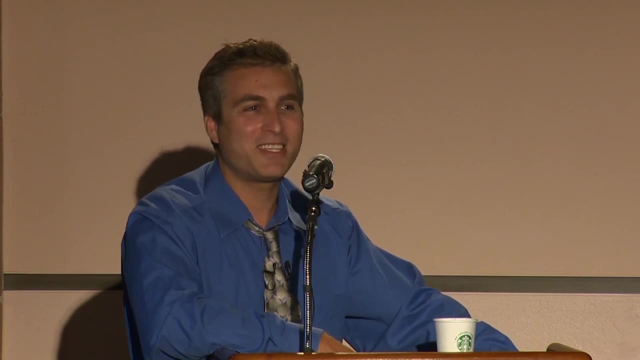 we can't count on them to stay in that area. They're sharks without borders, And it really highlights the need for binational management and research. That is, the people that make the rules as to how many fish can be taken out of the sea need to collaborate. the Mexican 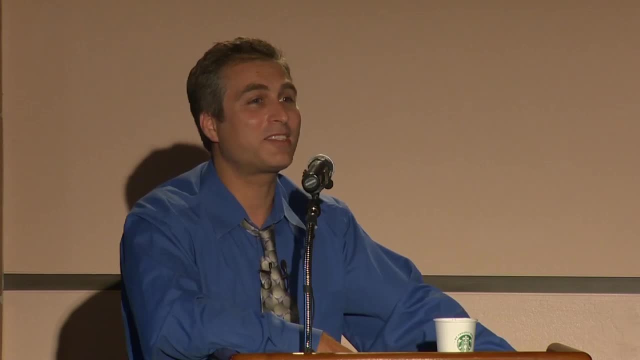 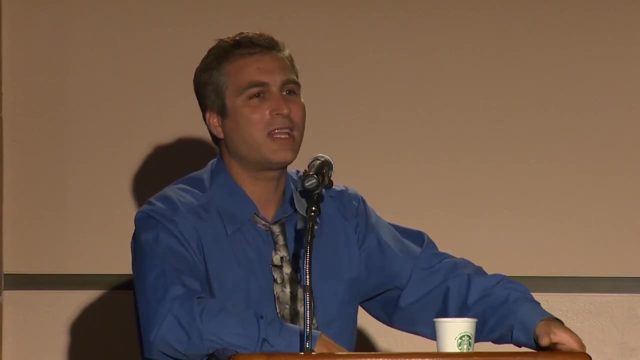 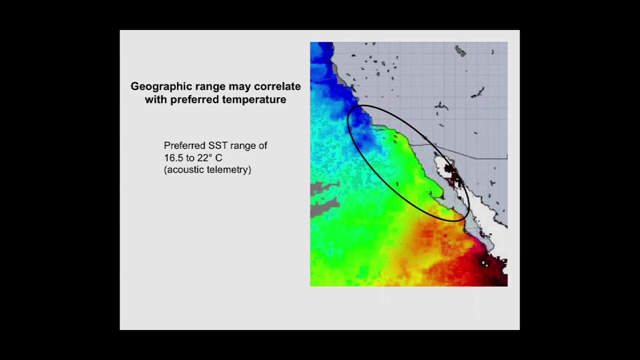 the Mexican fishery managers and the United States fishery managers, as well as the Mexican researchers and the United States researchers, And that's what we've been building over the last decade is a very strong binational collaboration. I just want to mention one other thing about this distribution. 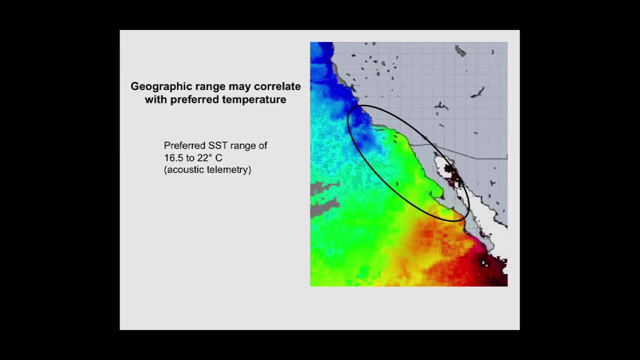 which is that I've mentioned a couple of very important points: Point Conception and Punta Eugenia. Point Conception kind of is the upper limit divides Southern and Central California And what these two, the reason these two points are so important in terms. 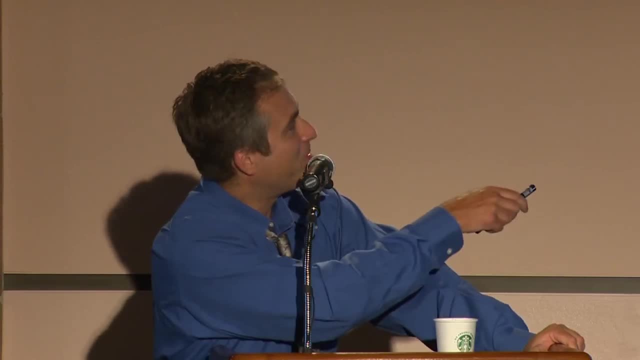 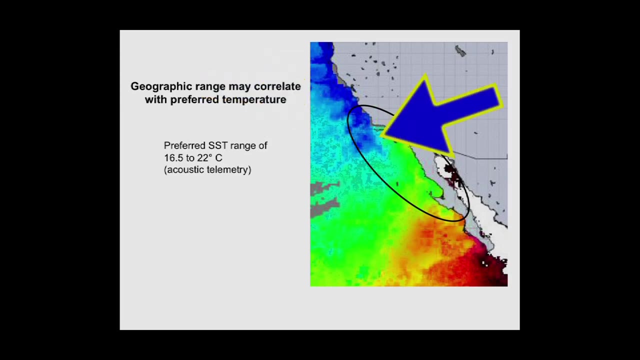 of the geographic range of sharks and other animals is because very cold water is coming down the Pacific coast And when it hits Point Conception, that cold water gets deflected offshore. At the same time, you've got very warm tropical water coming from south of Baja. 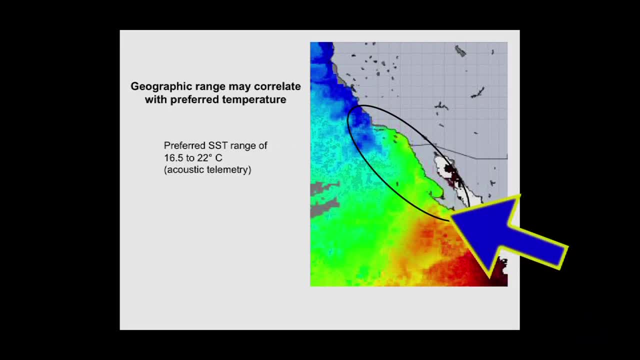 and moving up the coast, And when it hits Punta Eugenia that gets deflected offshore. So in between these two points we've got a very characteristic temperature regime, and so that reflects itself in a very characteristic Southern California bite fish population. 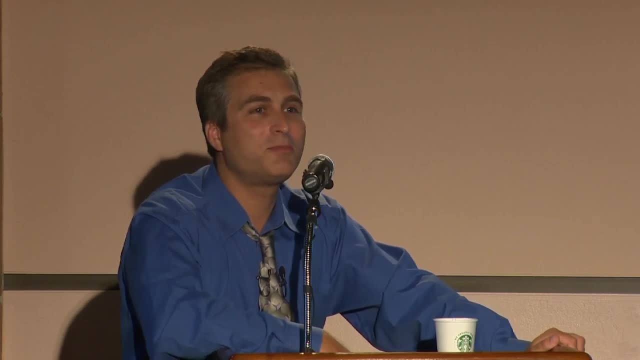 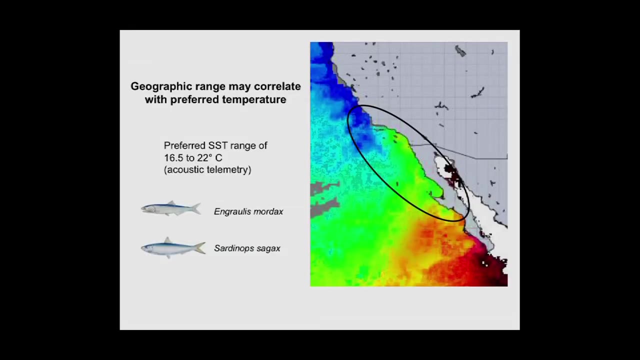 Not surprisingly, the preferred temperature range of thresher sharks, as measured by our electronic tags, corresponds very strongly to the temperature range which you typically find within this area, And that's also the temperature range which is favored by its prey, which are sardines and anchovies. 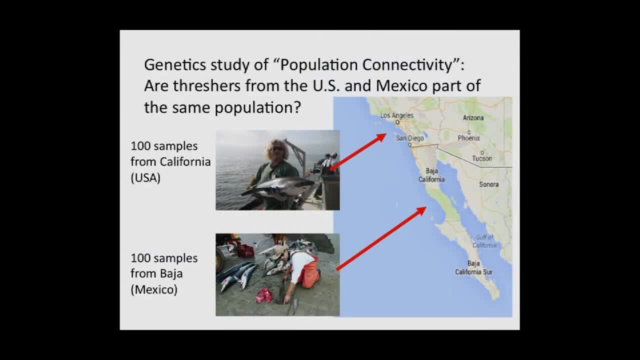 Here's a different kind of map. it's about a Google or that looks more like a Yahoo map, but it's the same area. and what? the point that this- that is, that I'm trying to make with this slide- is that, yes, we've got thresher sharks. 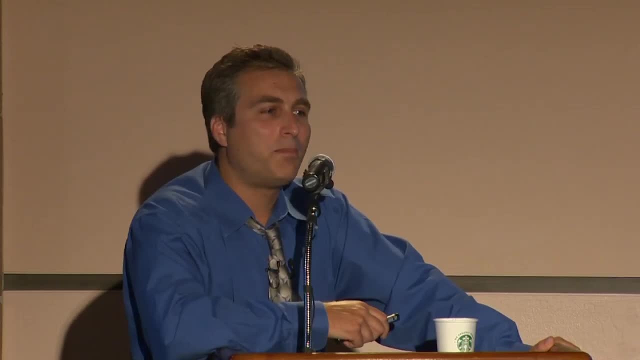 juvenile thresher sharks that are in this range, But in terms of fisheries management, in terms of how many of those sharks can be harvested from the sea, there's some important points to important biological concepts which we need to get a hold of. 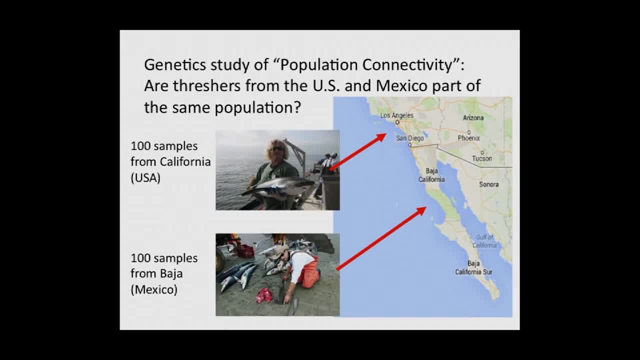 One of those is the concept of connectivity, And what that means is we want to know if that, if there's one big population that's ranging up and down throughout that area, or whether there are several sub-populations that stay in, stay in their own area. 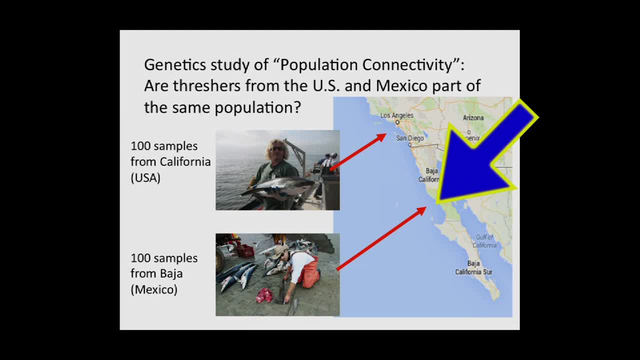 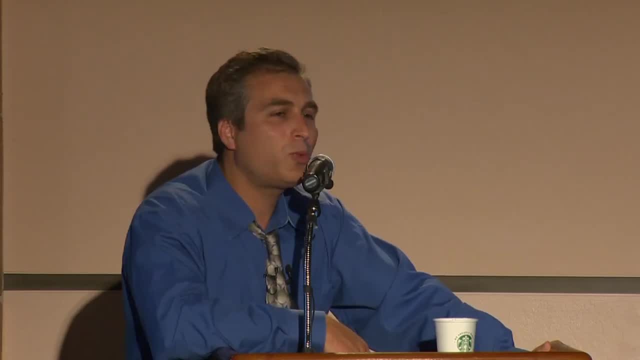 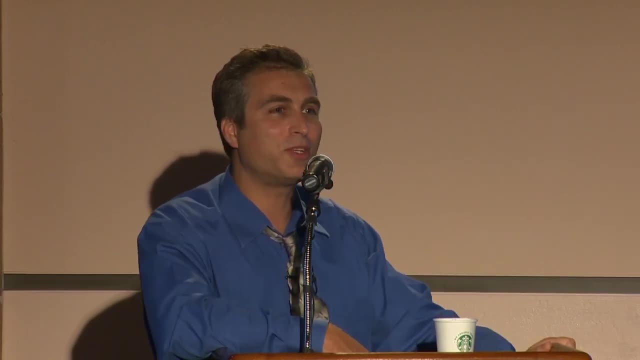 For example, if you can imagine if there was a sub-population down here in this bay, it would be pretty easy to wipe them out with some strong, directed fishing effort. So what we did was move up, go up to all of those sharks which we were capturing in California waters. 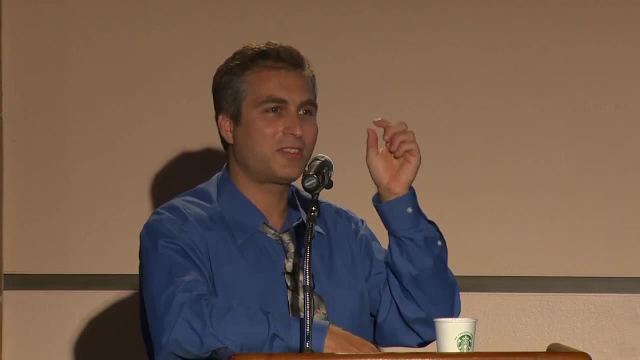 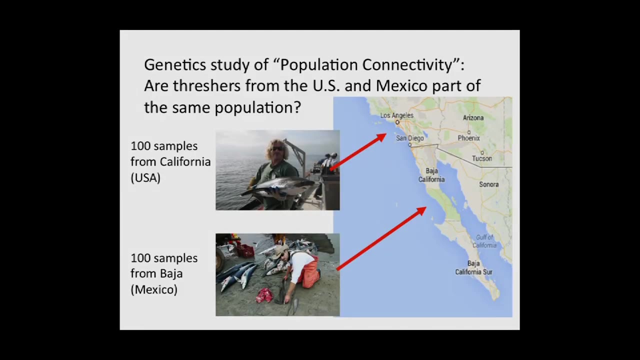 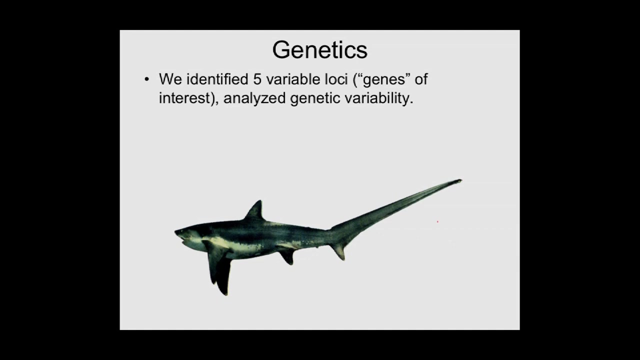 we took a little fin clip, just a little like a little tiny piece of tissue, released the shark. We did the same thing for 100 sharks that we caught in Baja California waters And we analyzed those tissue samples genetically. We analyzed the genetic variability of those tissue samples. 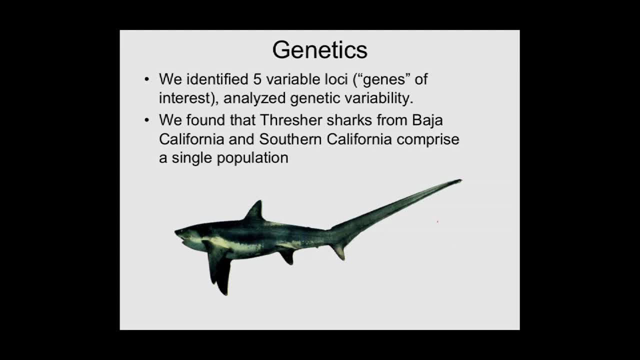 And, to make a long story short, we found that thresher sharks from Baja California do comprise the same population as those that we found that we find in Mexico. There's a lot of mixing going on there, And so the conclusion that we can draw from this is that thresher sharks, if we 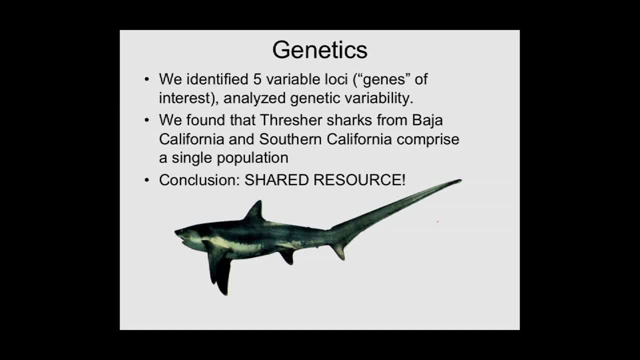 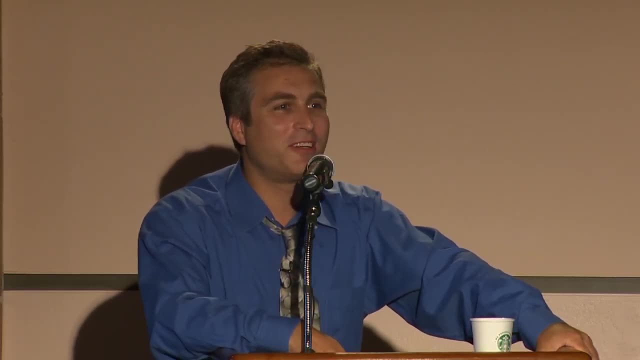 if we think of them in terms of a food or economic resource. they are a shared resource between the United States and Mexico And they've got to be managed as such. So a couple of other interesting things since I. I know that most people have not visited an artisanal fishing camp in Baja. 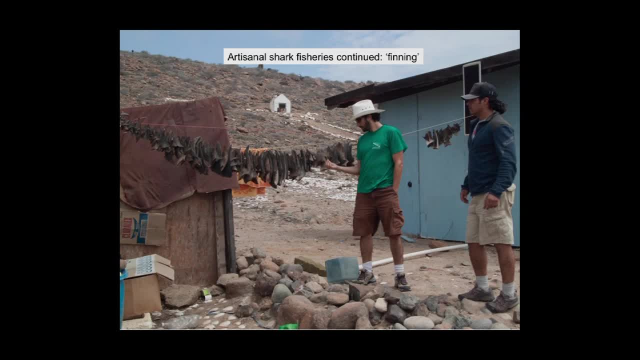 There's some interesting things that you see. For example, when you visit an artisanal fishing camp, very often you see a lot of shark fins drying on lines or in racks, And that would lead us to believe that a lot of finning is going on. 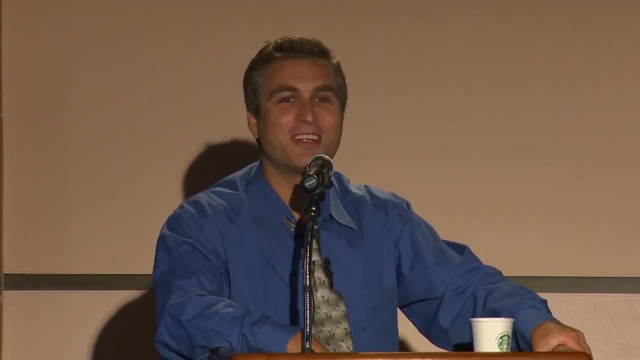 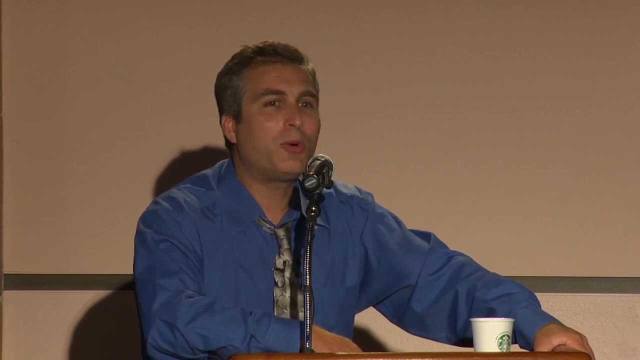 Probably shark week. I never watch shark week but I assume they cover the fact that shark finning is a major source of population declines in sharks worldwide. However, the technically finning is just taking off the fin and throwing the shark back dead. 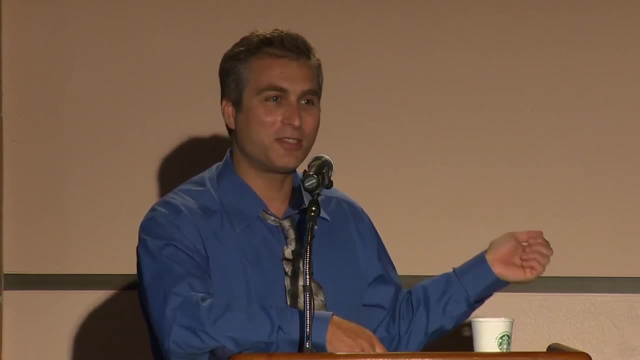 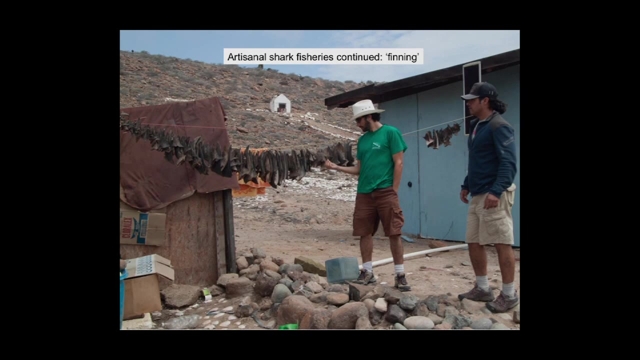 That does not occur, at least in these camps in Mexico. It's illegal in Mexico. It doesn't occur in these artisanal fishing camps, because they do get a substantial portion of their income from the actual shark. However, the fins are worth as much or more than the rest of the shark. 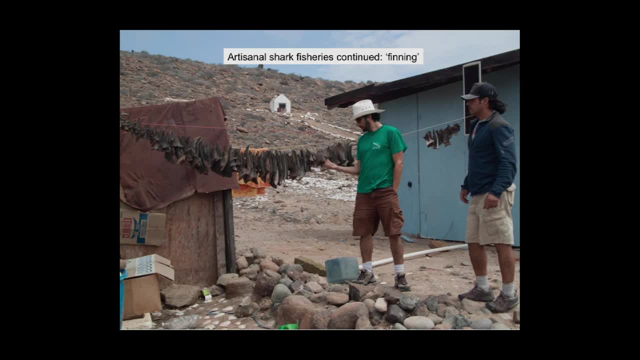 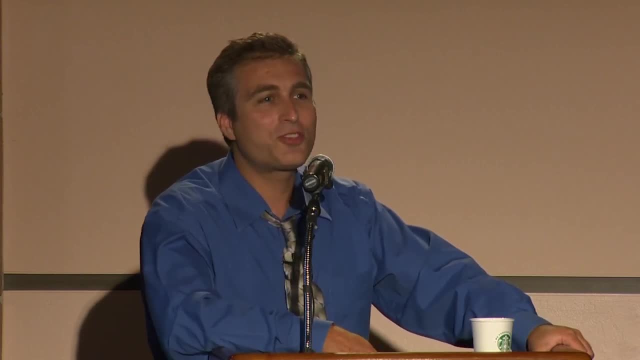 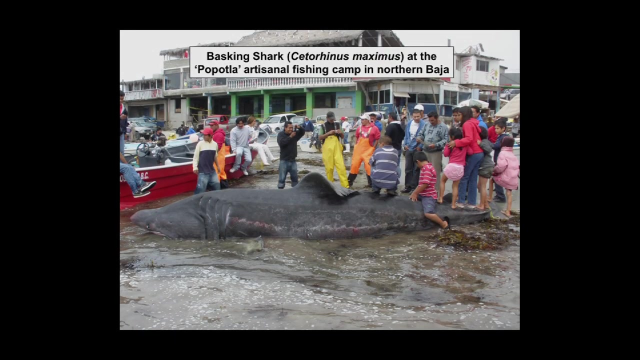 There are typically Asian buyers that will visit the camps occasionally, buy the fins and ship them back to China or Hong Kong or wherever it is, And so there is a strong, a strong driver for the shark, for shark fisheries. A couple of years ago we were visiting the camp at the artisanal fishing camp at Popotla. 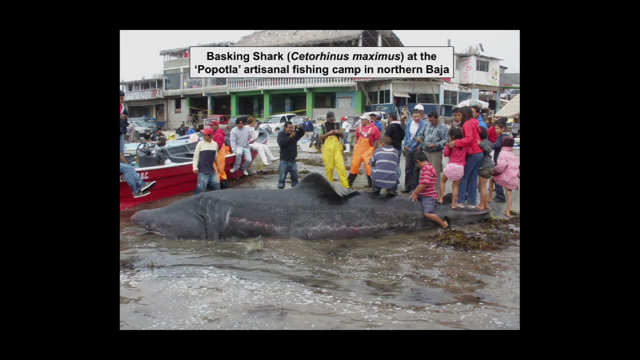 and we saw this basking shark come up in a in a fisherman's net. This was shark. the shark was just wrapped up in the net. It's just one of the amazing things that you see periodically when you're visiting these camps. 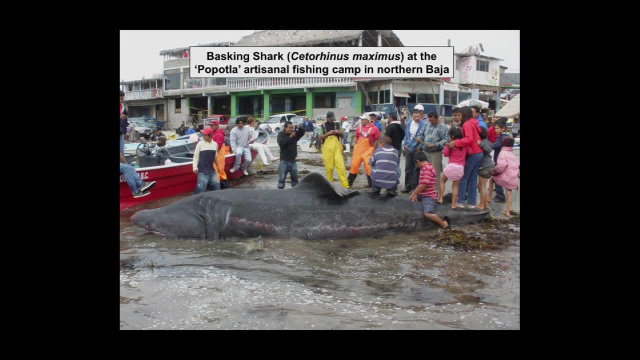 And I show this just one because it's a real cool picture. but the other thing is to highlight the fact that these are very local issues. I'm talking about artisanal camps and you look at this and you say, wow, this is another world altogether. 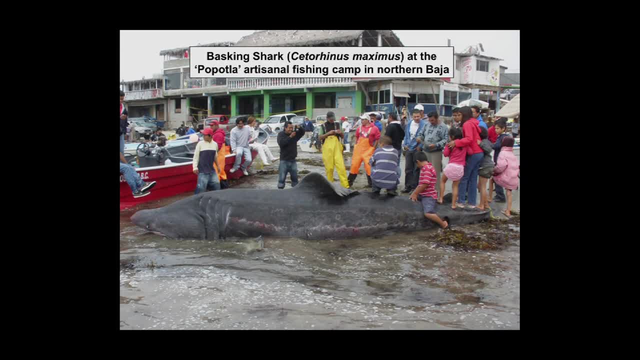 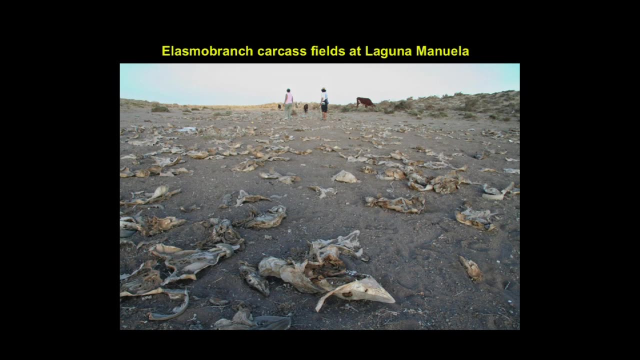 If we left Birch Aquarium right now, we could be in this. we could be at this spot in about an hour and 10 minutes, So it's not that far away. Probably the most bizarre thing that we saw at the artisanal fishing camps was at one of our very first visits. 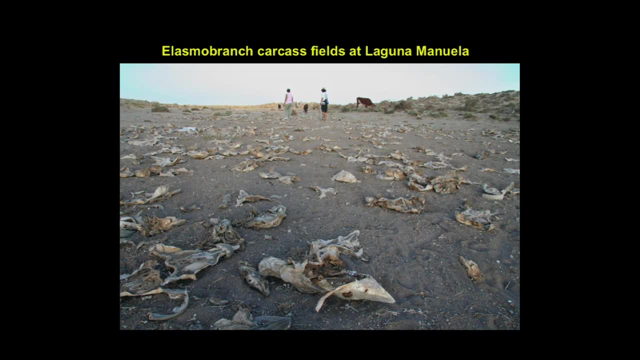 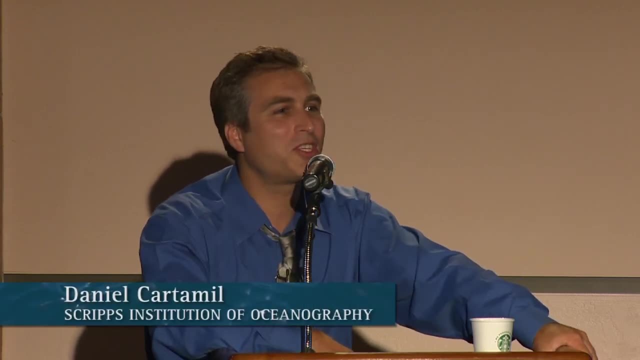 And these were the Elasmo branch carcass fields of Laguna Manuela. So Laguna Manuela is a fishing camp which we had heard about and we wanted to visit, And as we approached this fishing camp, we started to see the mummified remains of shark carcasses scattered throughout the desert. 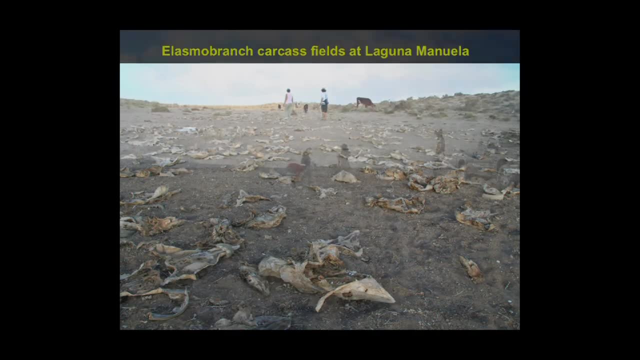 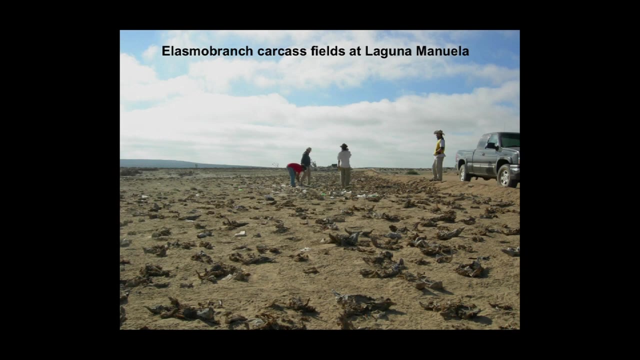 And as we got closer and closer, we saw more and more, And eventually we realized that there were many square miles of desert that were covered with the mummified remains of these sharks. And what it turns out is that these fishermen, because they're fishing in a biosphere reserve, they can't clean up the fish. 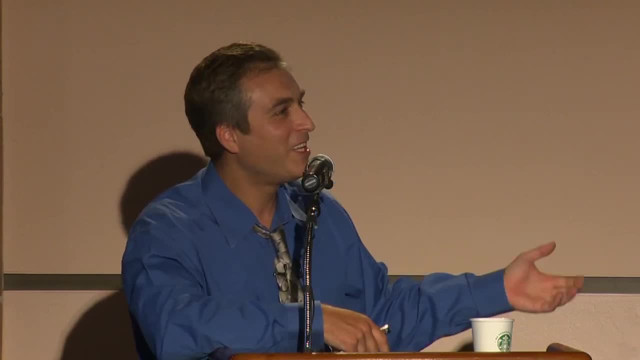 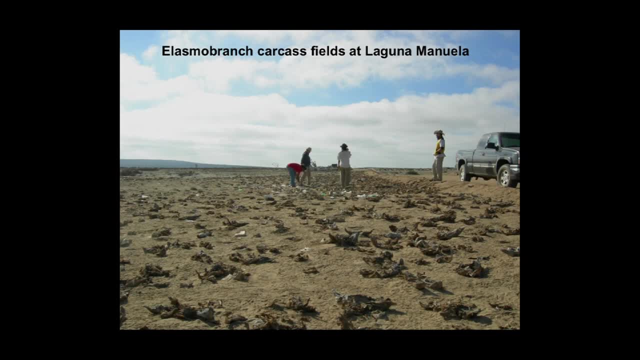 And on their way back home, they would dump those in the desert. The entrails would be eaten by coyotes or birds, And what's left are these thousands and thousands of skulls that become mummified because of the extreme heat and low humidity. 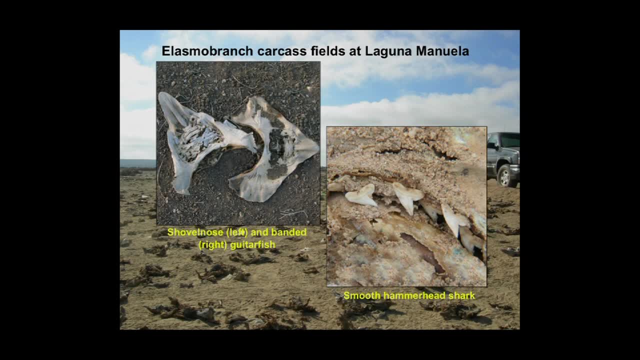 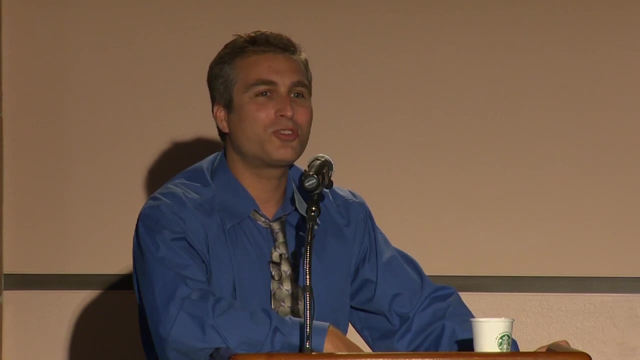 But, interestingly, what we found was that we could identify these remains Based on things like the shape of the head, the size of the sharks and the shape of the teeth, And so we set about to try and characterize the catch rate, the catch of sharks and rays at this camp, based on mummified remains. 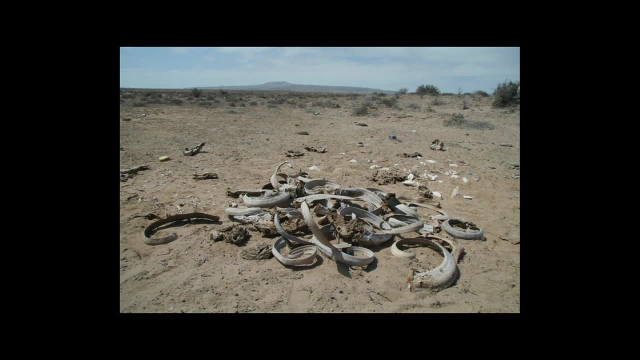 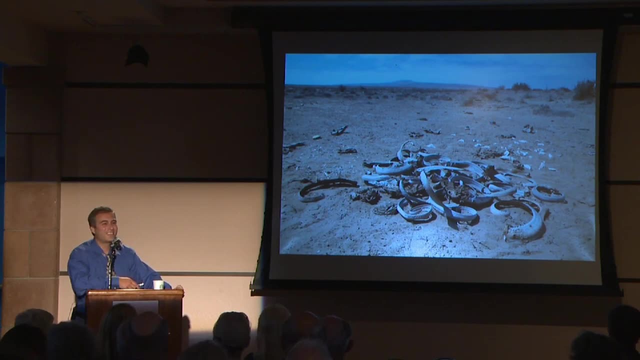 Now here's some mummified remains. I'd like to see if anyone in the audience can figure out what animal this is. You've got to get this. Somebody's got to get this one. This is a tail. I'll give you a clue. 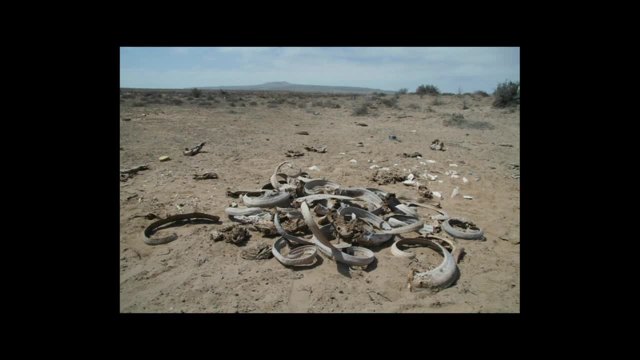 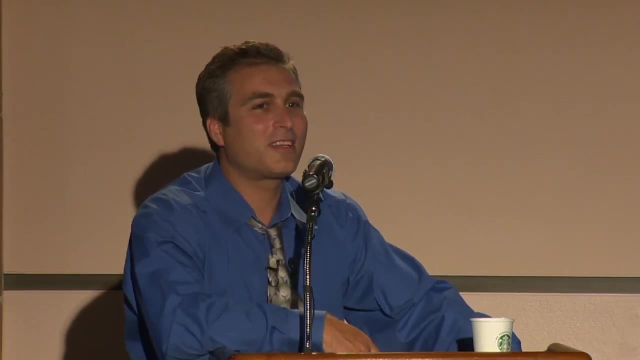 It's a thresher shark, They're a thresher shark. So when you find mummified thresher shark remains, what you find are these very long tails. So a friend of mine and collaborator, Omar Santana, did his master's degree. 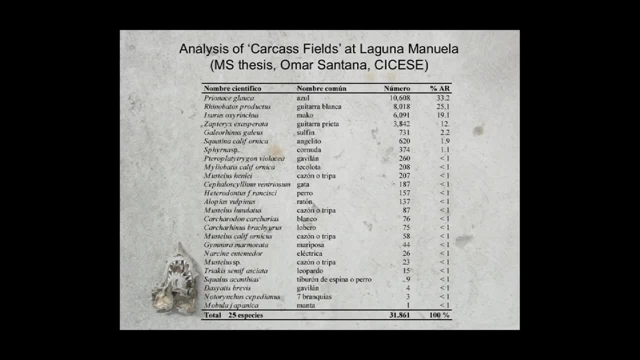 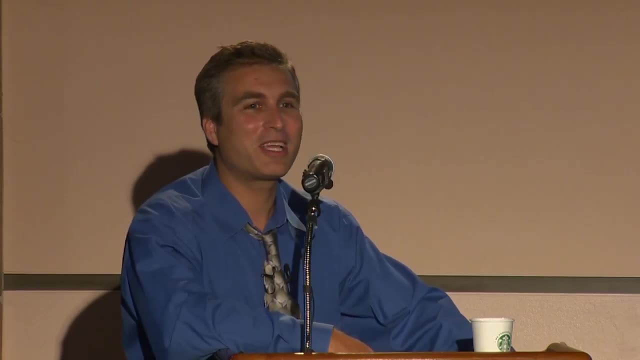 I was in the field a lot with him on this And we identified almost 32,000 of these Mummified carcass- which was all of them- And as far as I know that's the first time and only time that mummified shark remains have been used to characterize the catch composition at an artisanal fishing camp. 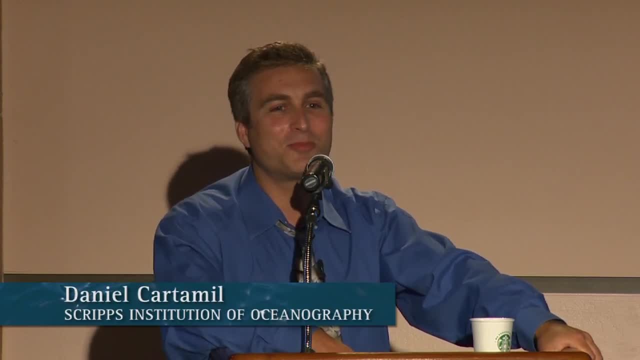 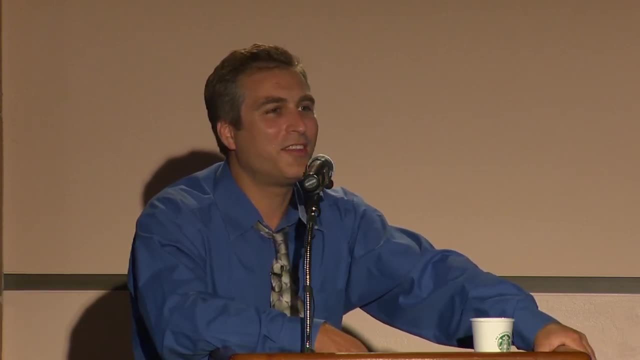 But of course that has severe limitations. One, you can't count on finding a field of mummified remains And second, that doesn't tell us anything about the size of the shark, the sex of the shark, what gear was being used. 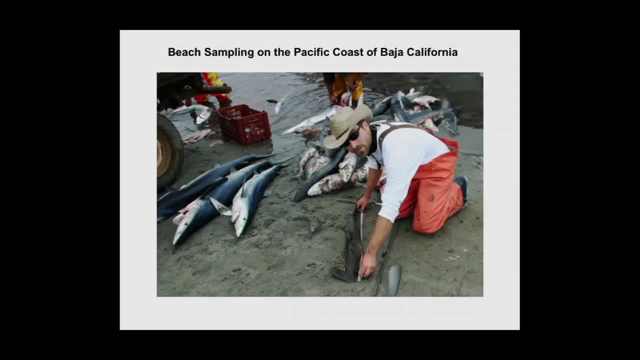 How many, How many boats were out fishing and that kind of thing. So for that we relied on beach surveys. This was where we would go visit a fishing camp, set up our tents on the beach next to the camp with the collaboration of the fishermen. 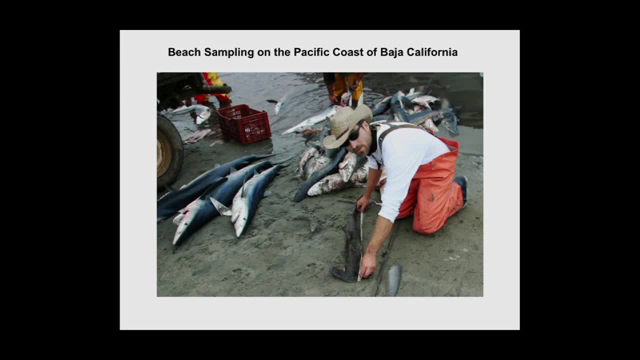 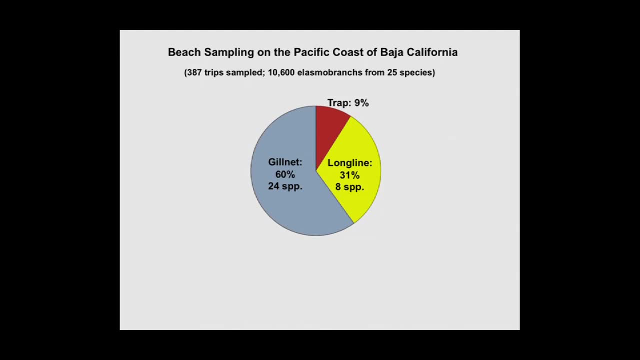 And every time a boat came in, we would run out there and collect data on every single shark in red, And this gave us a really good idea of the fishing effort along the Pacific coast of northern Baja California. So really what? 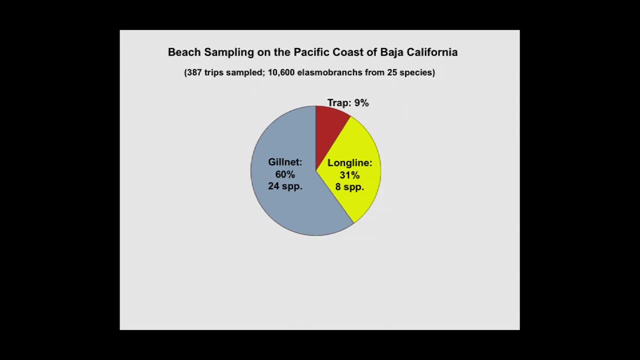 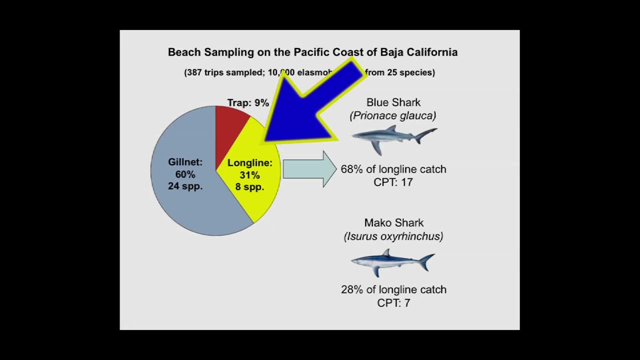 We found out of this, just to summarize, was that there were two primary types of fishing that were going on that were catching sharks and rays. One was long line fishing, which accounted for about a third of the activity and caught eight species, primarily blue sharks and Makos. 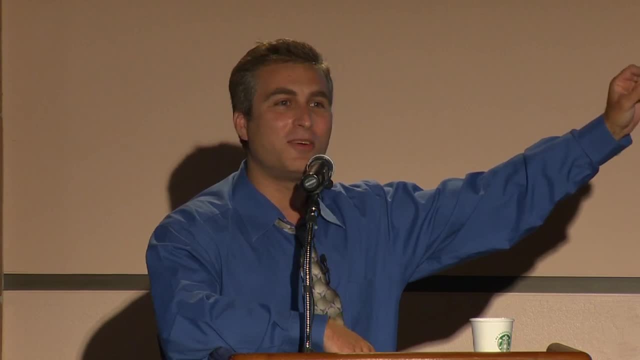 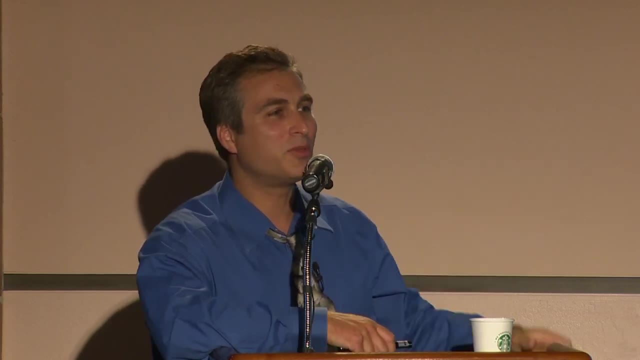 So a long line is simply a long line with hooks hanging off of it that's put offshore- about 10, 20 miles offshore- and baited with fish, And it catches a lot of blue and Mako sharks. So 95% of these sharks were immature. 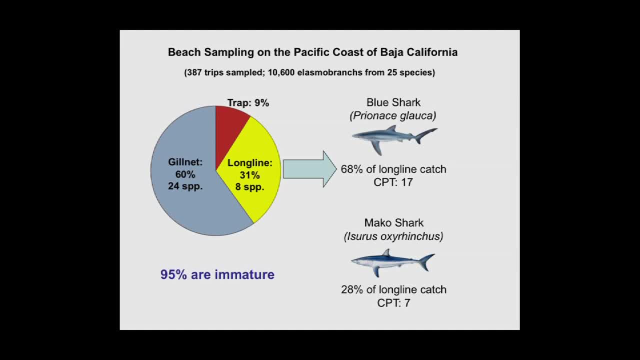 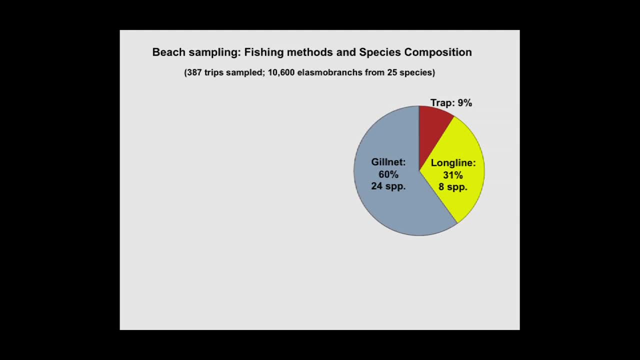 So they're catching very small blue and Mako sharks, obviously fishing in an offshore nursery area for these. Now, the other method that we find is gill net fishing, which accounts for about 60% of the fishing effort, And they catch primarily two species of rays which we can find right here in La Jolla Cove. 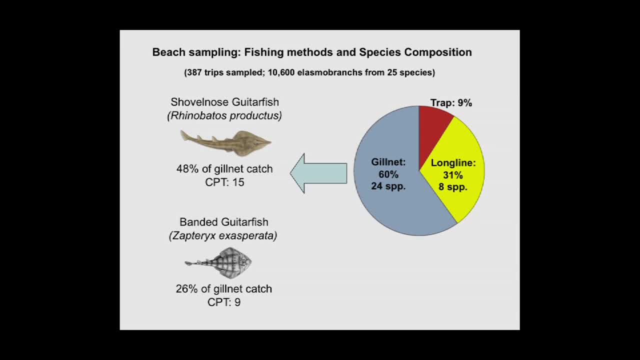 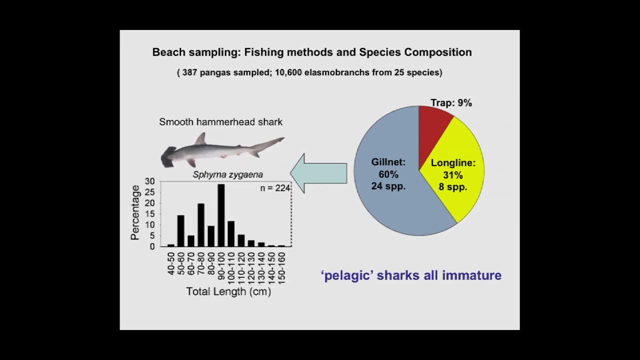 They're called guitarfish, a shovelnose and a banded Guitarfish, But there were 24 total species that were caught with gill nets, including some species that are typically offshore, such as the hammerhead, the smooth hammerhead shark. 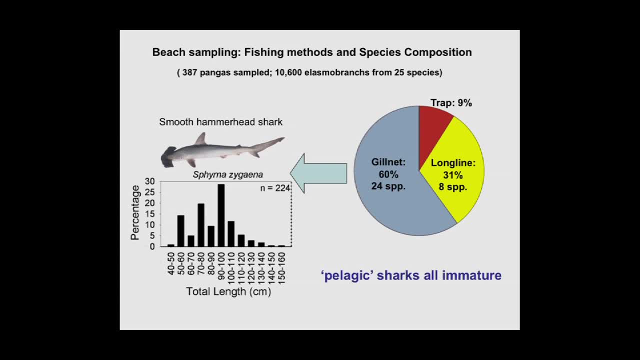 And if you look at the size distribution of smooth hammerhead sharks, again, they're typically about one meter or less in size. So what's happening is these offshore sharks are coming in to give birth. The smooth hammerheads are using the coast as a nursery area. 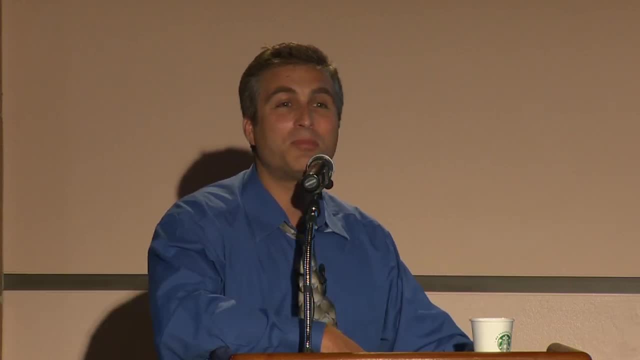 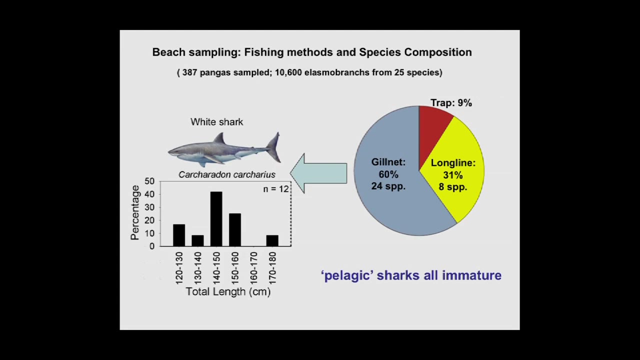 Just like the Thresher's, and they're undergoing a lot of fishing pressure in that area. We saw the same thing for white sharks. We didn't expect to see a lot of white sharks. We'd never heard of white sharks in that area. 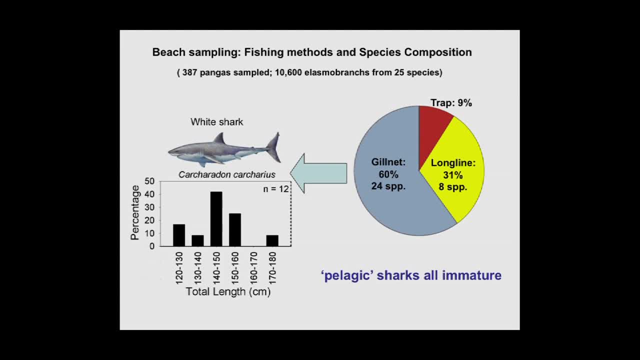 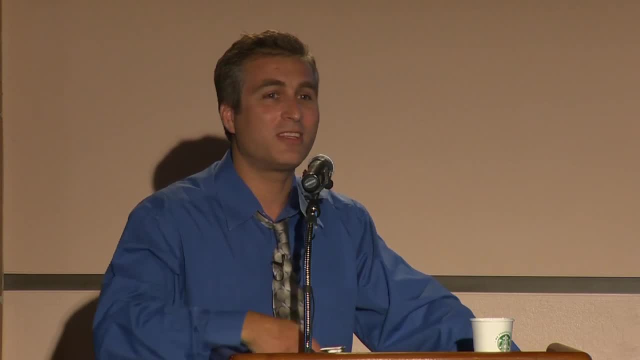 And we only saw a few in our beach surveys, But we saw many, many in our carcass in that carcass field, indicating that we're just probably not there at the right time There's, but that there's a lot of juvenile white sharks being caught there. 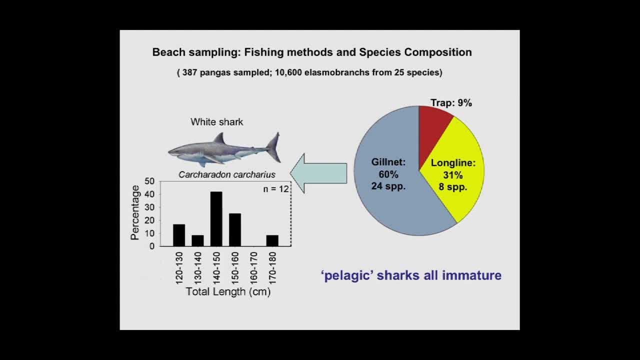 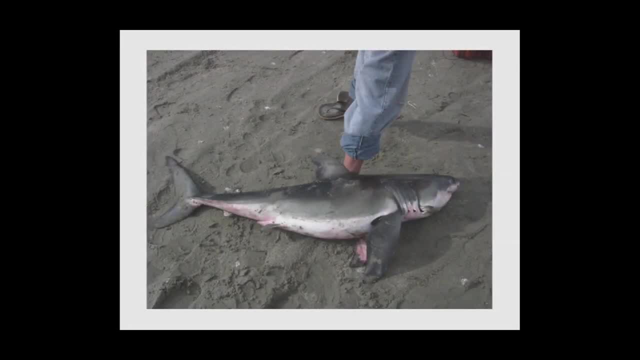 And again very small, about one point five meters in length, Which Corresponds To a newborn, to one year or two years of age juvenile white shark. And this is pretty important because white sharks are one of those highly charismatic species that are the focus of a lot of conservation work and and effort. 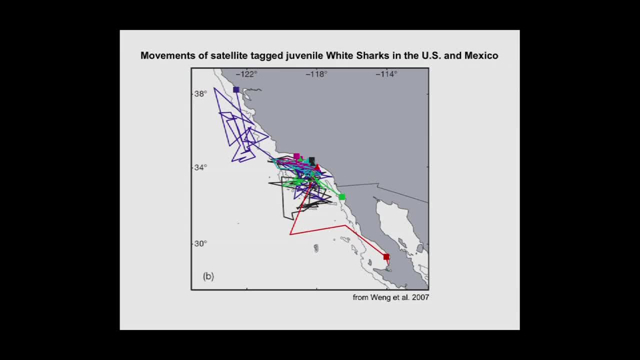 And these are just the results of some pop off satellite tracking, results of a friend of mine, Kevin Wang, up in Monterey, who tagged juvenile threshers with pop up satellite tags And they had a very similar distribution to what we saw with the thresher sharks and mostly in Southern California, but some of them moving into Baja California to use the inshore waters as a nursery. 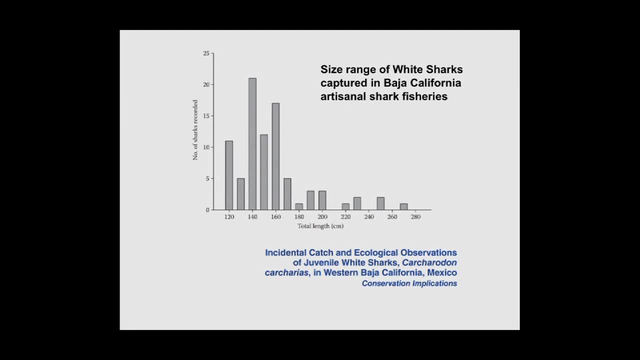 And so those results are. results of white sharks were just recently published in a book on white shark biology and cited in a recent update to the status of the white shark population on the west coast of North America. So there's a couple of take home messages with regards. 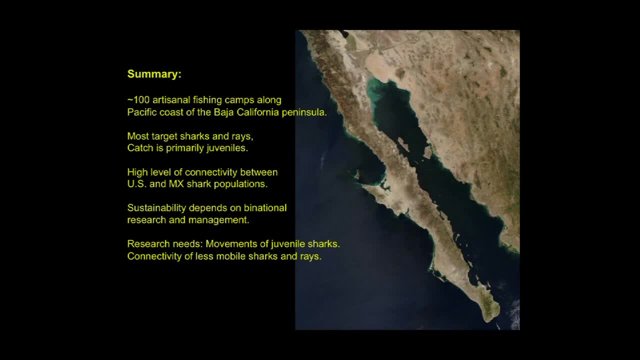 To artisanal fisheries, That is, there's a. there's approximately 100 artisanal fishing camps scattered along the Pacific coast of Baja California, many in very remote places where they're essentially unmonitored. A lot of them target sharks and rays, at least seasonally, and most of the catch consists of juvenile sharks. 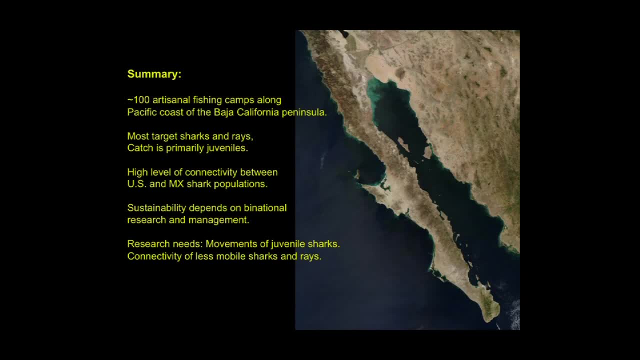 We've been finding so far that there's a high level of population connectivity between US and Mexican populations of the same species. So sustainability of those species depends greatly on binational collaborative research and management endeavors. So we've identified a few research needs, that is, we're that we've just recently been funded to study, and those are the movements of juvenile sharks. 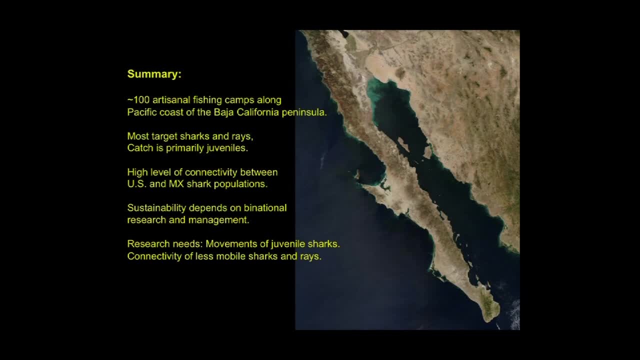 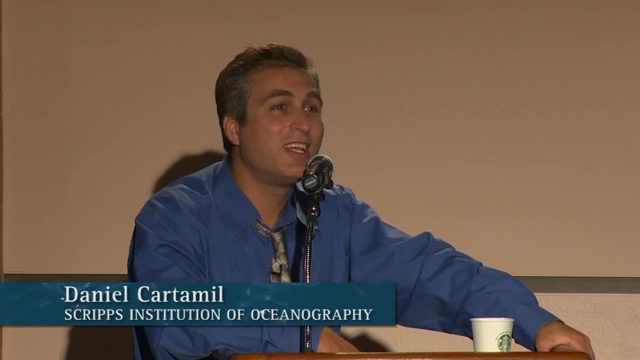 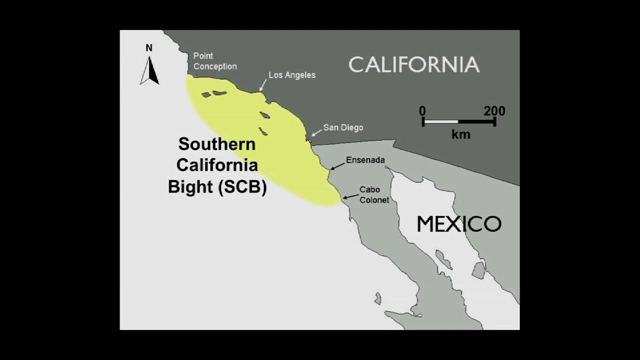 Like the thresher shark, but other species throughout this range, and the connectivity of less mobile sharks and rays. So, for example, one of the things that we're doing right now Is looking at satellite tag studies of Mako sharks and blue sharks, but of the smallest size class. 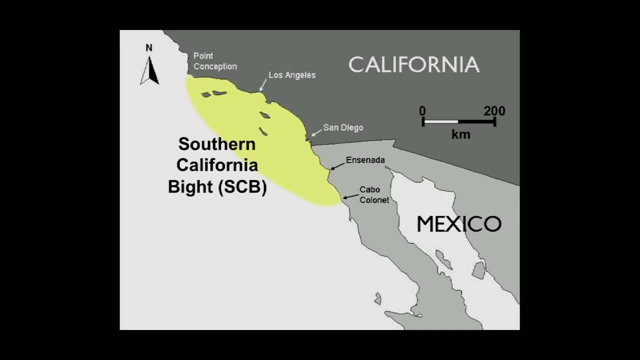 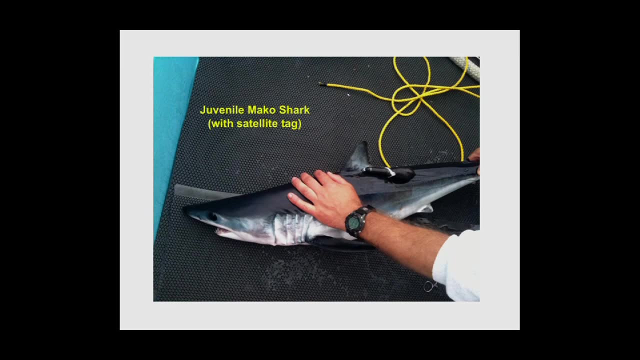 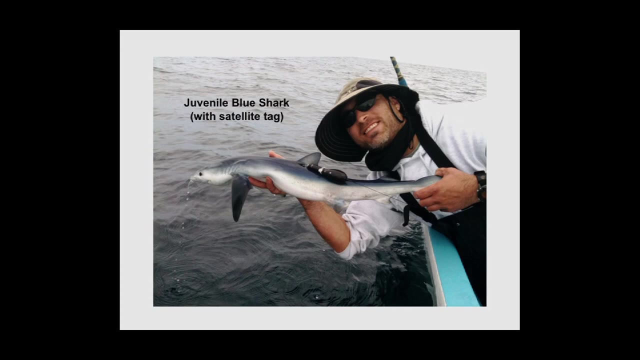 These are the smallest Mako's and blues that have yet been tagged. So here you see it. here You see a baby Mako shark with its tag. That's about as small as Mako sharks get. And here we see a juvenile blue shark with a satellite tag. 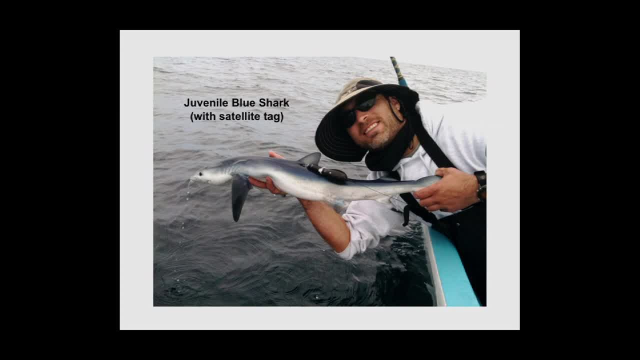 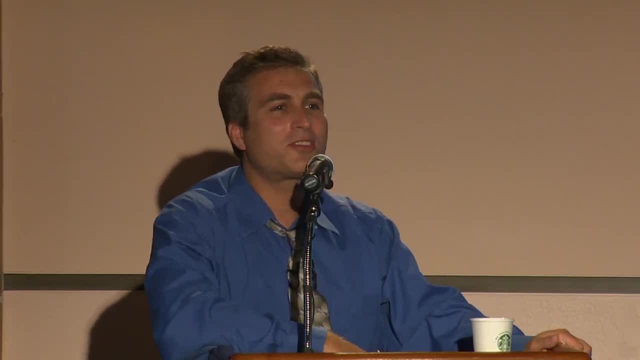 And that's not as small as they get, but that's about as small as they can get and still hold One of these tags without it affecting their movement patterns, And so we're. the other thing that we're we're starting to study is population connectivity of less mobile species. 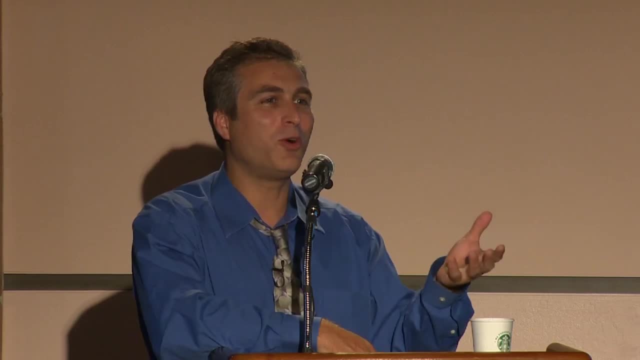 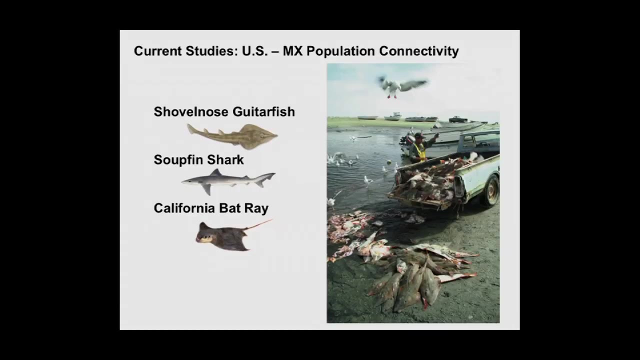 It makes sense that something like a thresher shark or a or a small white shark would move up and down the coast and that there'd be high degree of population connectivity. But when we think of things like the shovel nose guitar fish, which was the top catch in gill nets in Baja, and Baja sewer, you don't really imagine them. 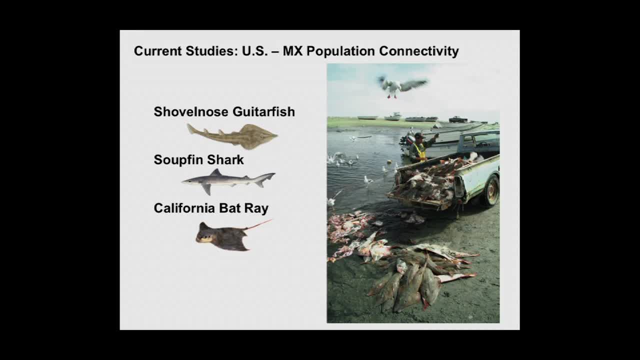 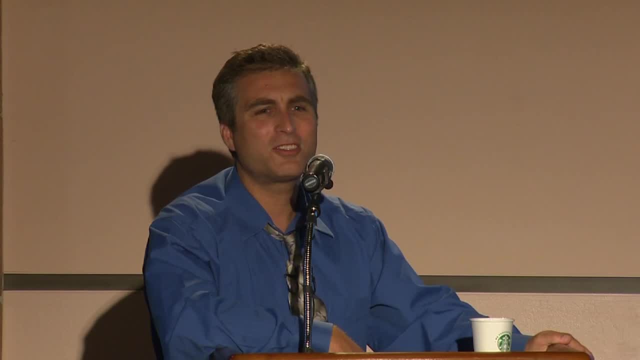 Moving It very much. You, normally, when we see them off the coast they're just sitting on the bottom. but we, we don't know. we don't know anything about them. We don't know whether they migrate or whether they have what their large scale and fine scale movement patterns are. 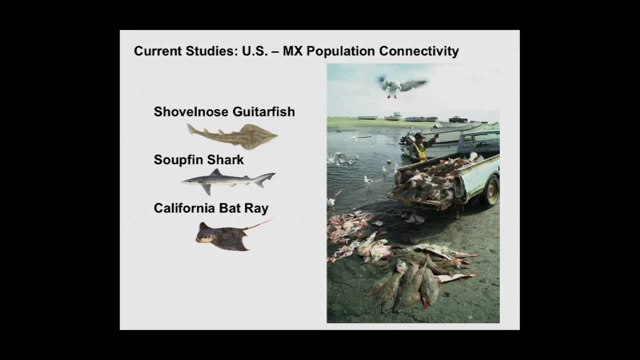 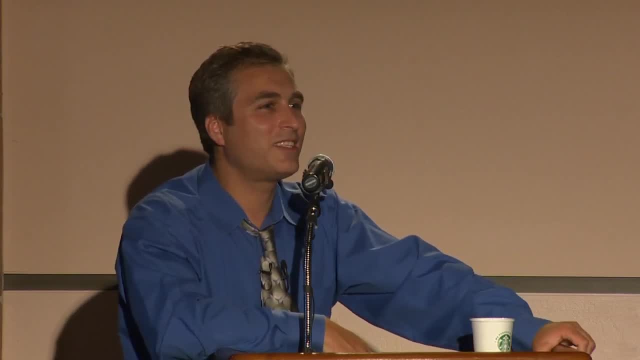 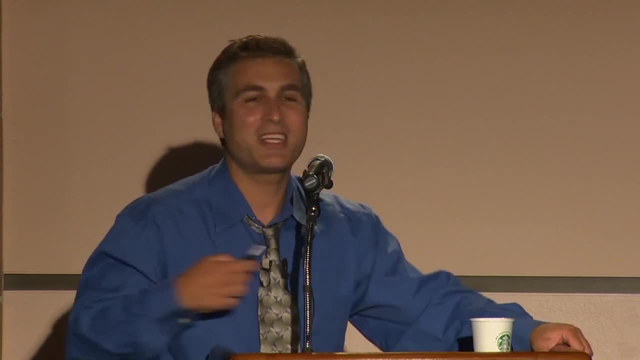 So we're looking into that with genetic studies, and we're also satellite tagging soup fin sharks as well. Finally, one of the projects that that I'm excited about is a photography conservation project. It's very appropriate that we're here today With Octavio abort. those amazing photography. 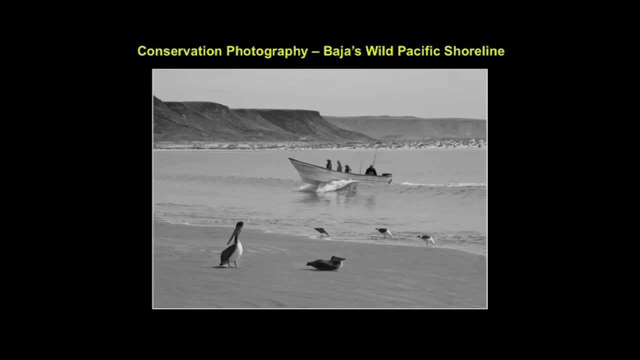 I don't know if you've had a chance to look at it while you're here. Octavio is a great photographer and he's got some beautiful underwater photographs around here, And photography is a great medium to promote conservation, because it really brings the beauty of these areas to life. 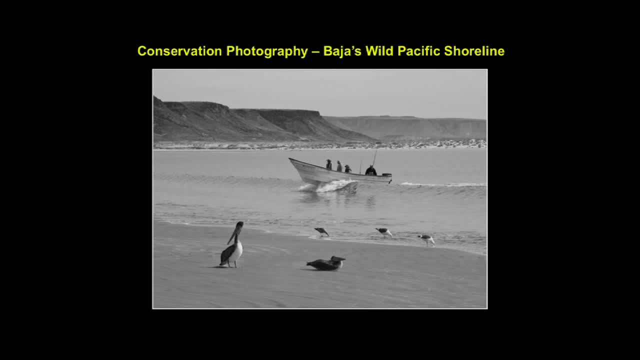 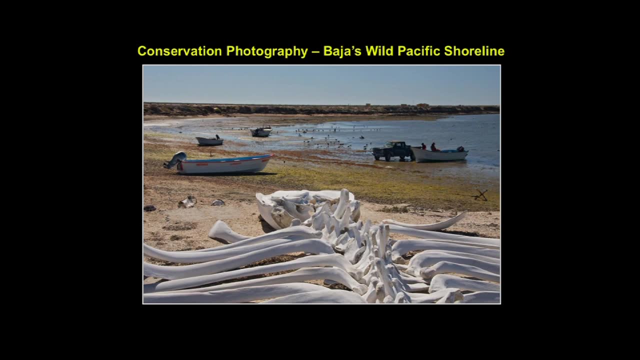 And so we've recently been funded to to institute a photography conservation project in which we will use photography to highlight a lot Of these same conservation issues that I'm talking to you about today with respect to shared marine resources and their management and connectivity issues. 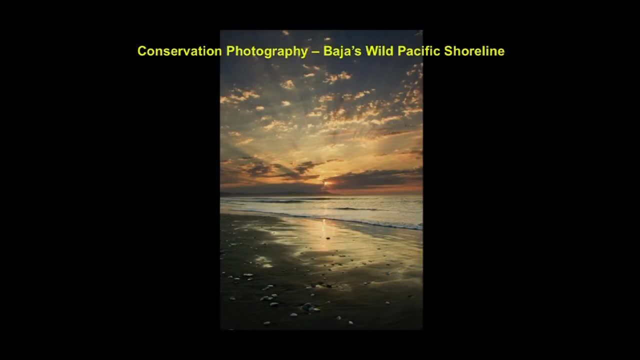 But you know, there are other issues besides marine connectivity, one simply being the aesthetic beauty of places like Baja California. When I first went down there, I was floored and flabbergasted by the beauty and the remoteness. 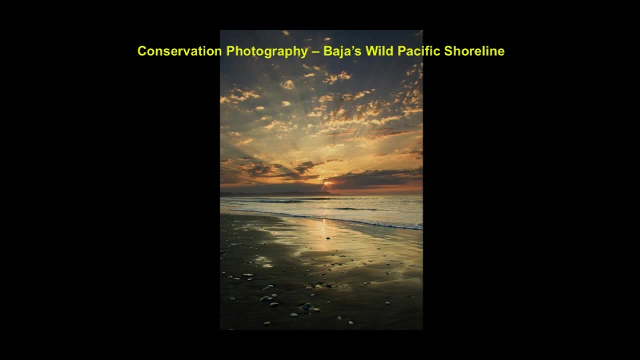 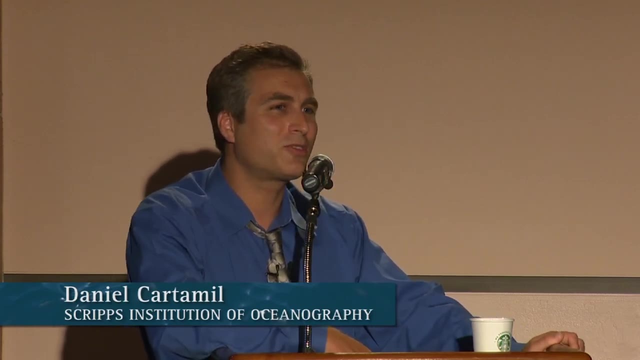 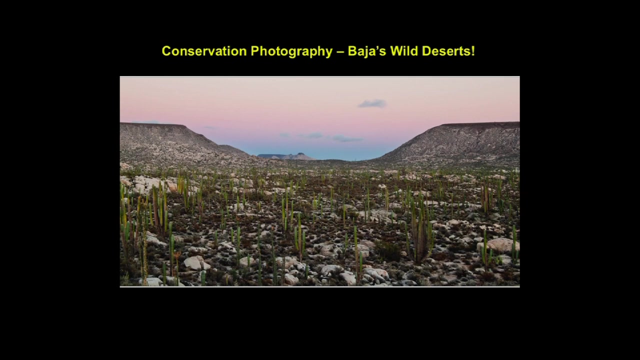 And the undeveloped nature of some of the coastline that I saw and still see, And so I think it's really important to bring some of these issues to light, like potential land development, coastal development and habitat degradation issues, And there are also some other very amazing habitats in Baja California that are little known. 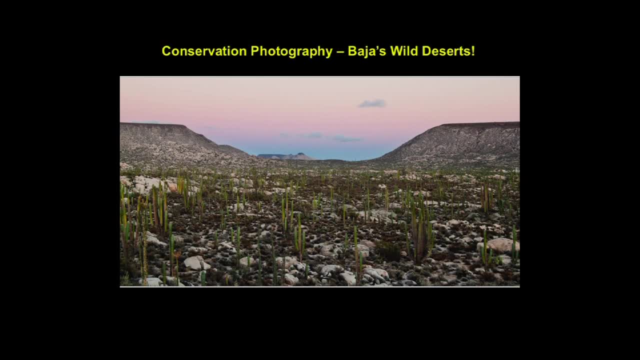 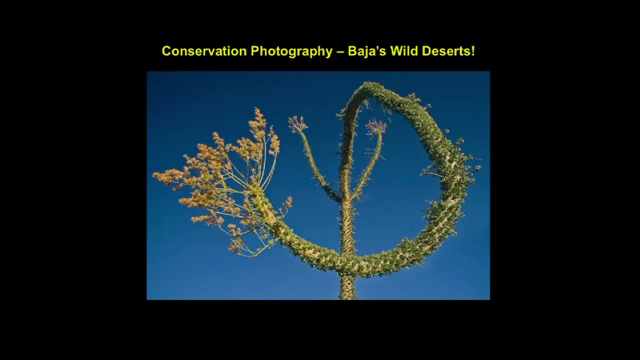 Perhaps the desert isn't as little known, but it's little known to most people, even in Southern California, that we've got deserts in central Baja that are as beautiful As they look like Joshua Tree but on steroids- and and are home to some really bizarre and beautiful plant and animal species. 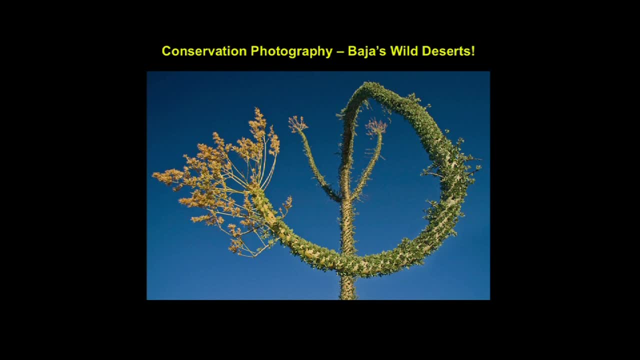 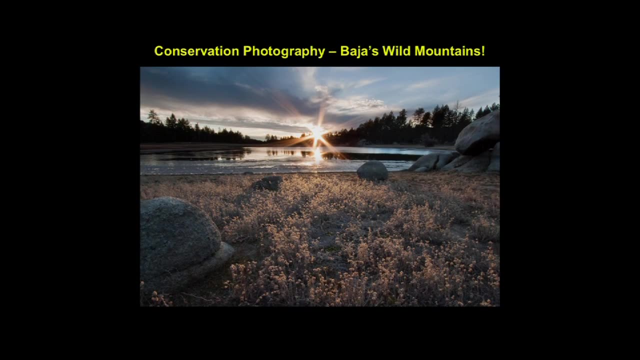 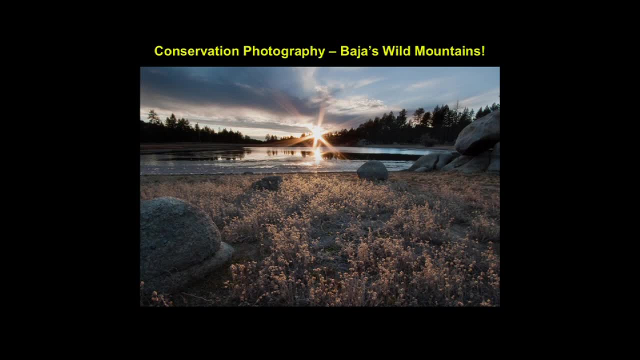 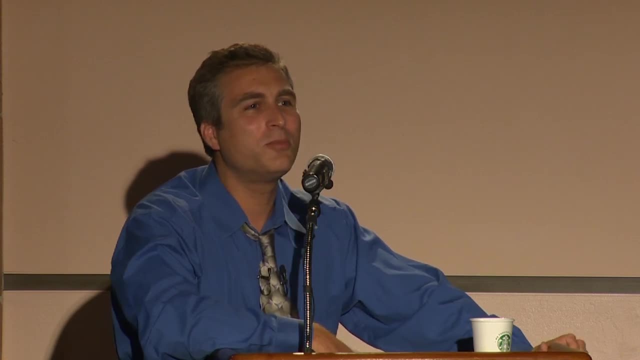 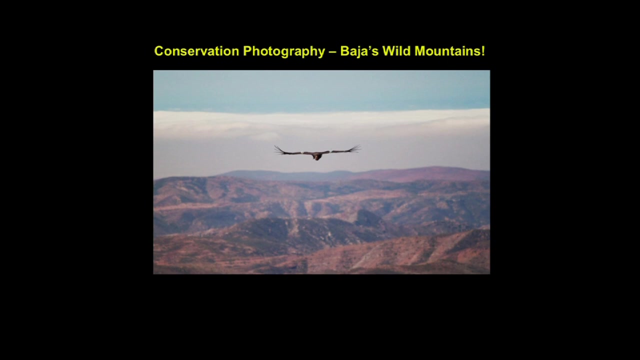 There's peaks in northern Baja that are over 10,000 feet high, Covered by snowpack half of the year, and contain vast pine forests and lakes and streams, And that's not something that's very commonly known. They're home to a lot of highly migratory species, like the recently reintroduced California condor. 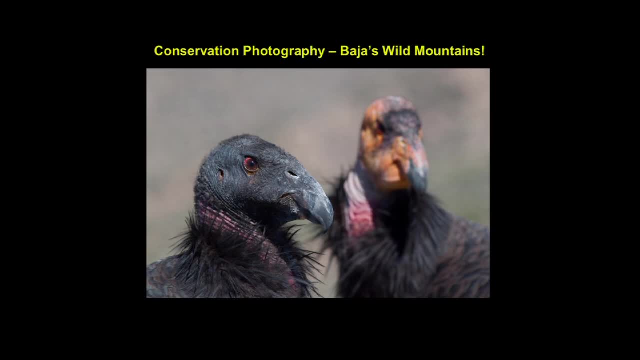 So there is a not. it's not just marine species. There are also a lot of terrestrial and sort of flying species that are not just marine species. There are also a lot of terrestrial and sort of flying species that have a lot of biological connectivity. 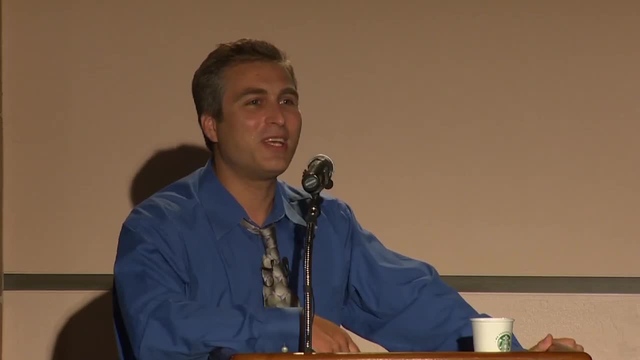 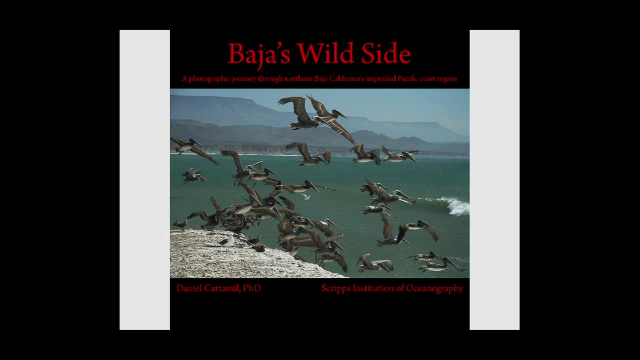 So there's a lot of connectivity in general between the United States and Mexico, and specifically Southern California and Baja California, And that's extends not only to the animals but also culturally and economically, And I think is what I, what we hope to achieve by this photography conservation project is to bring some of these issues into the public consciousness, because, well, anyway, I just want to say thank you so much for being here. 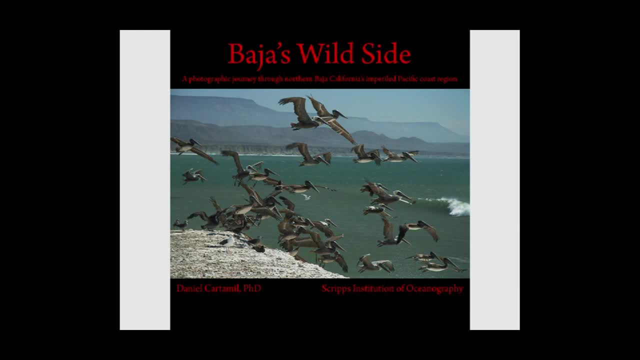 Thank you so much for being here. Thank you so much for being here, And I wanted to show you this, This slide here. This is the cover of the book that will eventually come out. It's called Baja's Wild Side, which which is I refer to the Pacific Coast as the wild side. 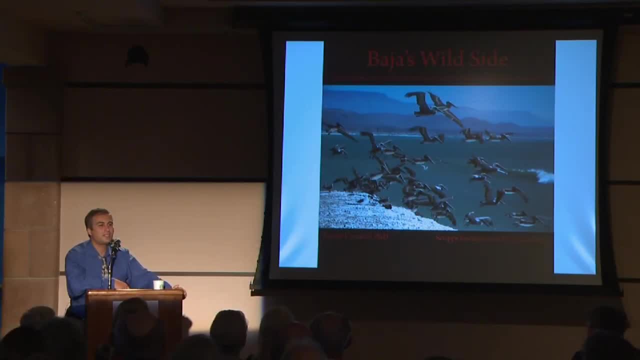 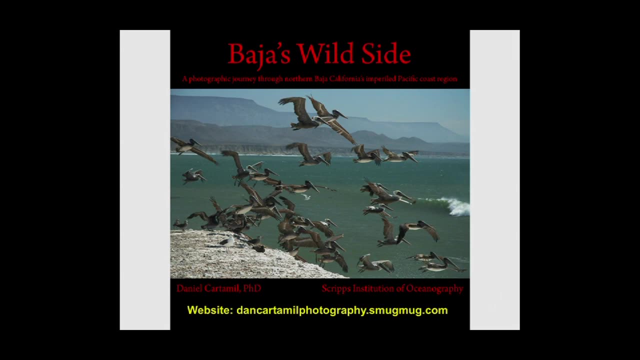 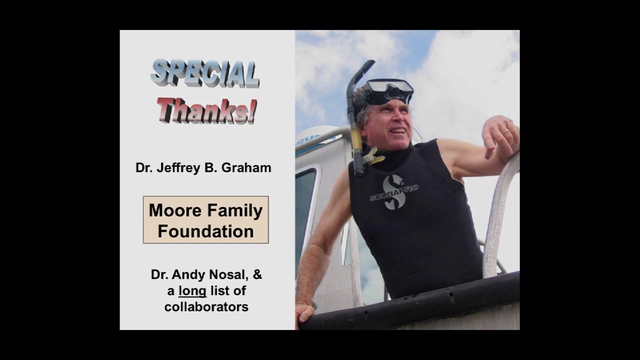 And hopefully it'll be on sale in the aquarium and we'll have a. we'd love to have a photography exhibit, like we do here with Octavio's work, And hopefully that will be available And hopefully it'll be available. We've been acknowledging a couple of people. 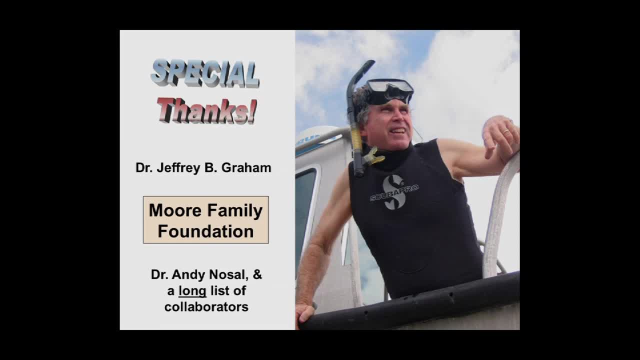 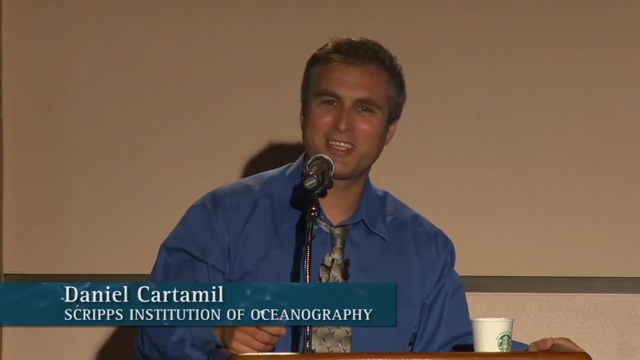 One is the Moore Family Foundation who has been funding us for the last five years. We've been funded by several organizations But Moore has been really instrumental in the last five years in getting a lot of this work done. Dr Andri Nosil is the guy that runs the Scripps Research Shark Research program with me. 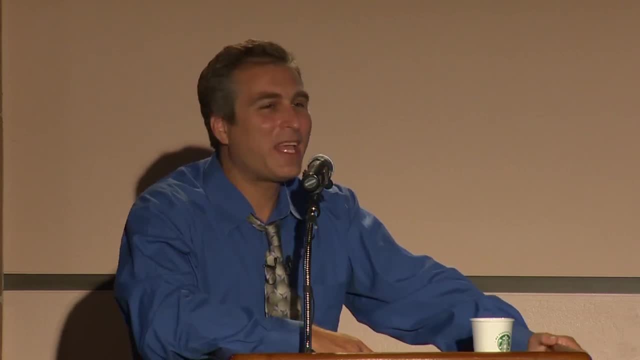 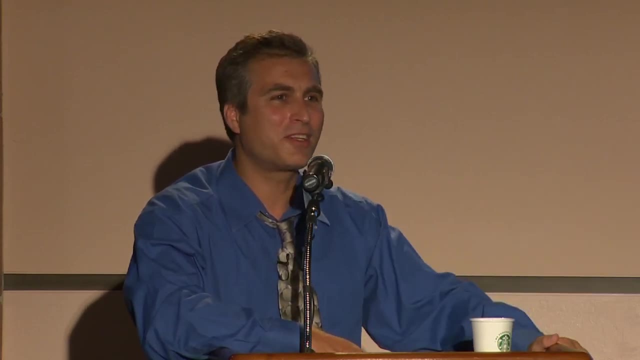 Our supervisor and adviser is Dr Phil Hastings, who's in here somewhere I can't see with the bright lights. Yeah, hi, Phil. collaborators, The work here is just the tip of the iceberg for most of these studies and involves probably about 30 or 40 different people doing a lot of work. It's not just. 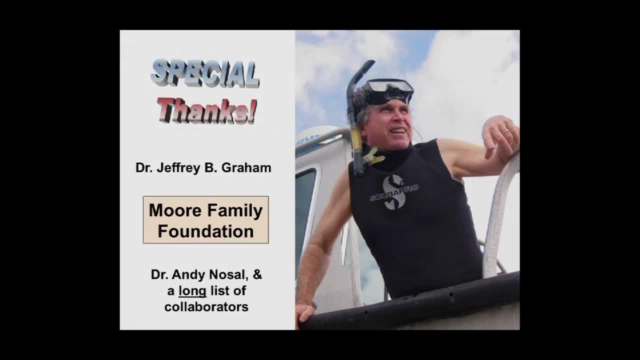 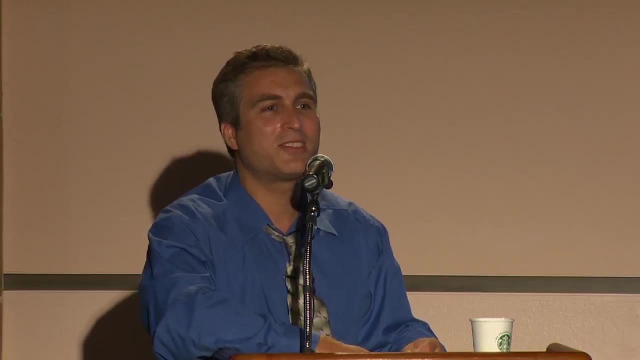 my work by any means. And finally, I'd like to acknowledge Dr Jeff Graham. After all, this is the Jeffrey B Graham lecture series. I had the great fortune of being one of the last grad students to enter Jeff's lab and do my PhD with Jeff. It was an amazing experience. 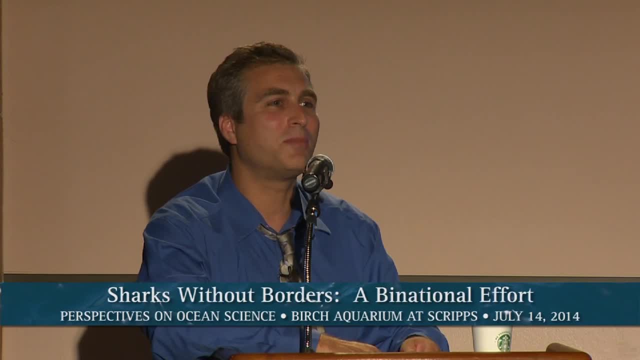 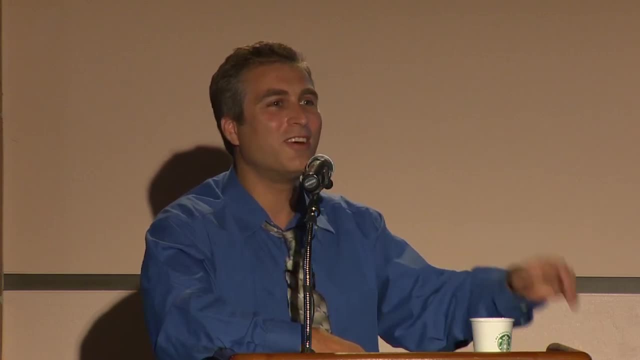 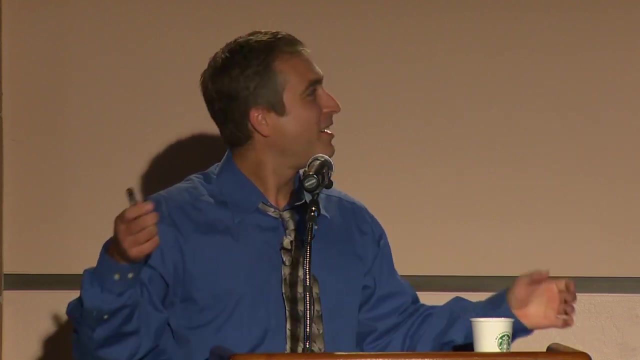 to be mentored by Jeff and to have his friendship, And we're thrilled to have some of Jeff's family here. Jeff's brother and son are in the audience. We're still having support from Jeff and his family And, that being said, I would like to invite you to ask any questions. 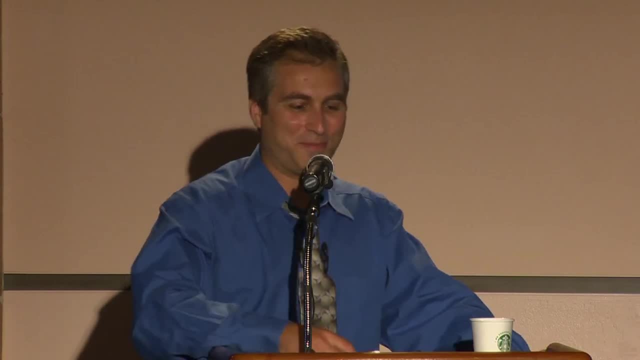 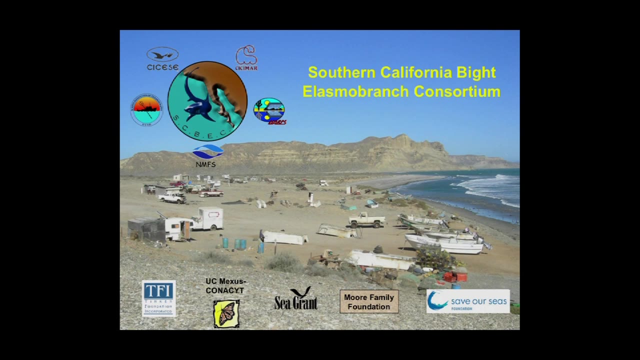 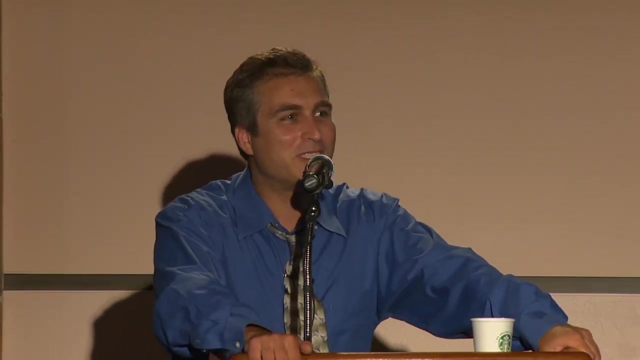 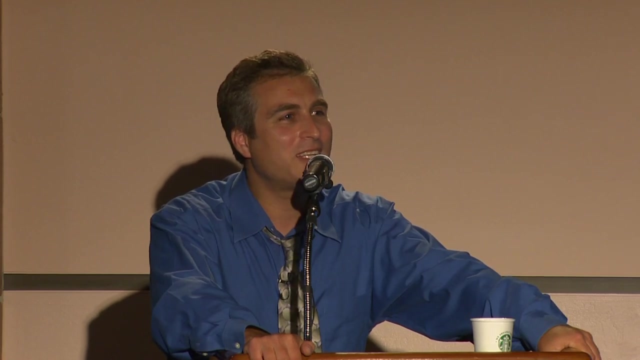 at this time. if you have any, I'd love to talk to you about it, Thank you. So the question is: we've been discussing binational fishing management, fishery management, but what's happening in the United States? Is the United States doing a good job of sustainably? 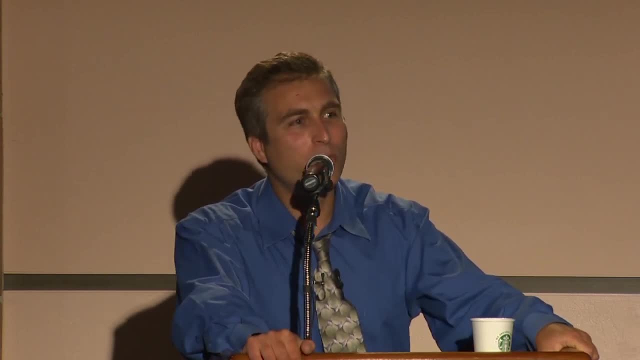 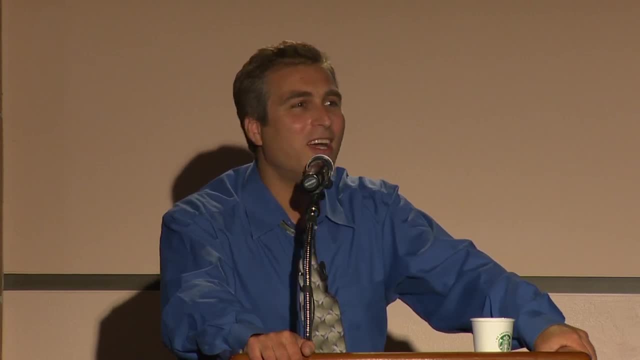 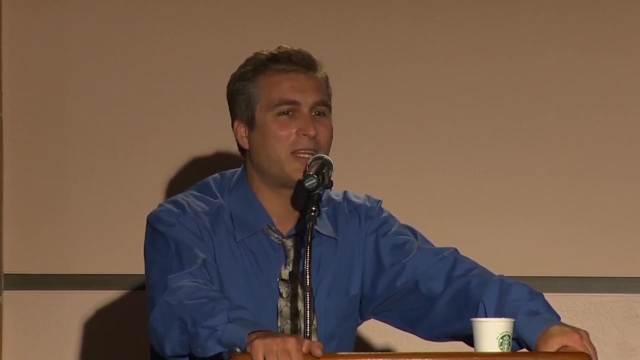 As you saw by that graph. However, in the past couple of decades, fishery management in the United States has done a great job And I would say that there's a high level of collaboration with Mexican researchers and Mexican fishery managers And all indications. 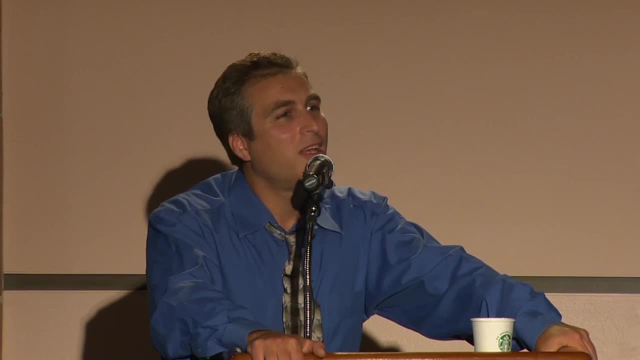 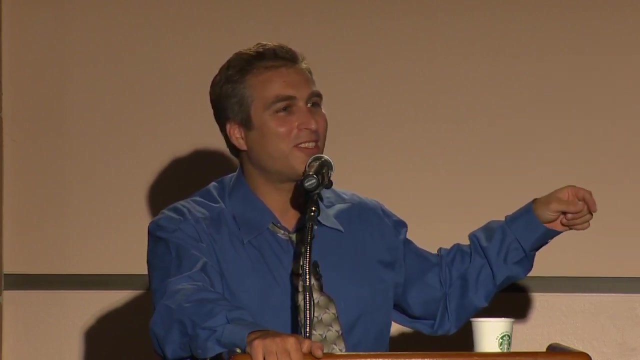 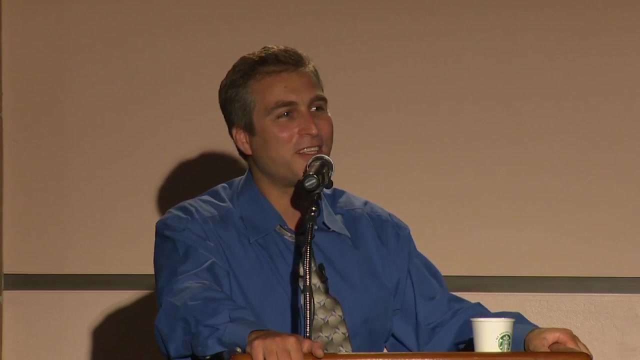 are that thresher shark populations are rebuilding. We conducted an extensive study of Mexican commercial shark fisheries and we did find that concomitant with what was happening with this crash of thresher shark populations in the United States waters there was actually a big fishery, a similar drift, gillnet fishery, based out of Ensenada, that no longer exists. 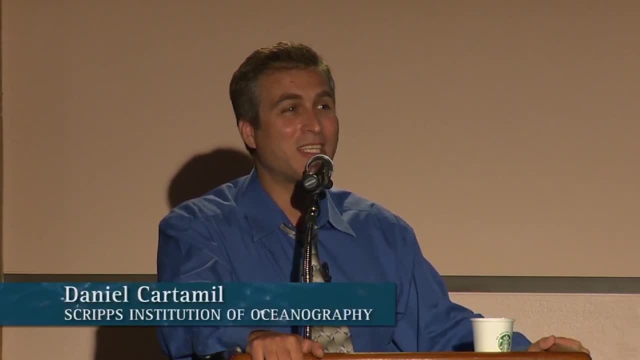 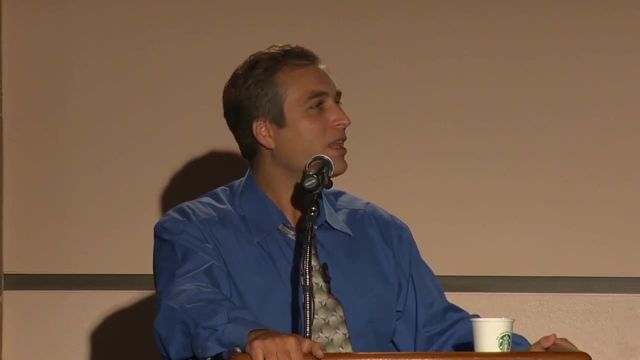 and we didn't even know about. It was a pretty big fishery and they were also taking a lot of fish out of the water. That fishery no longer exists because drift gillnets were banned in Mexico And the Southwest Fishery Science Center, which is responsible for thresher shark management. 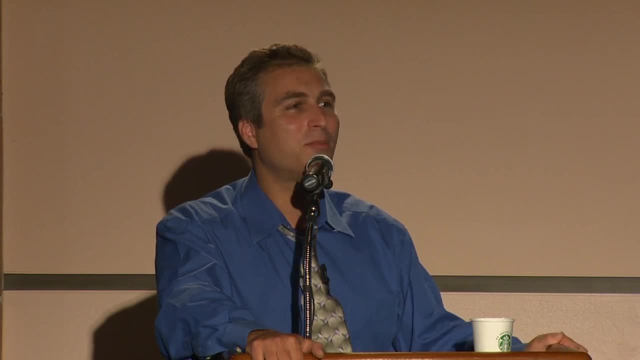 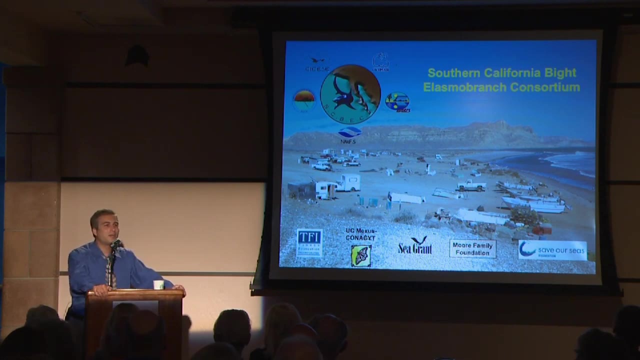 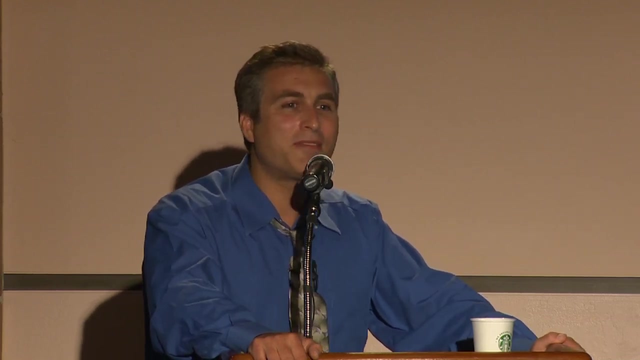 now estimates that thresher sharks are rebuilding their population pretty steadily, However. so that brings up a good point, which is that most of the time when you hear about shark, for example, eating shark, you'll hear something like: well, don't ever eat shark, And that's. 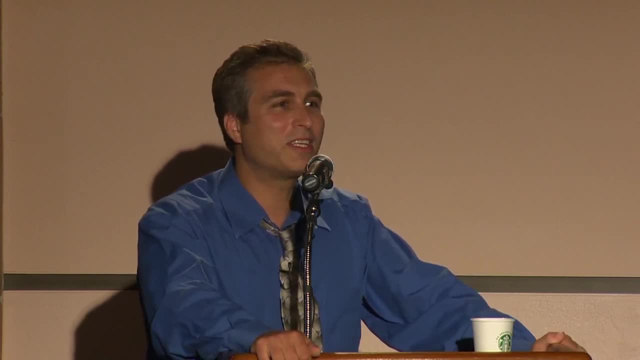 a good guideline that conservation groups want to follow, And that's a good guideline that conservation groups want to follow, And that's a good guideline that conservation groups want to follow And that's a good guideline that conservation groups put forth because, realistically, most people can't distinguish between what's a sustainable 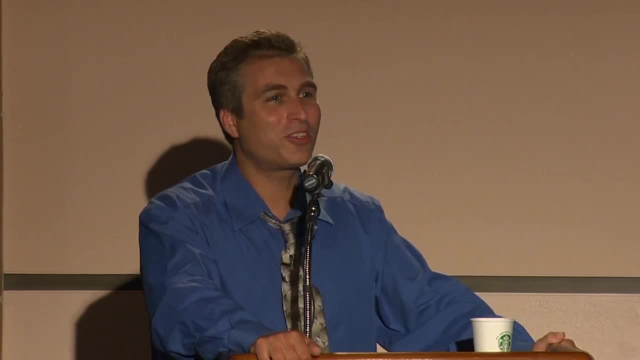 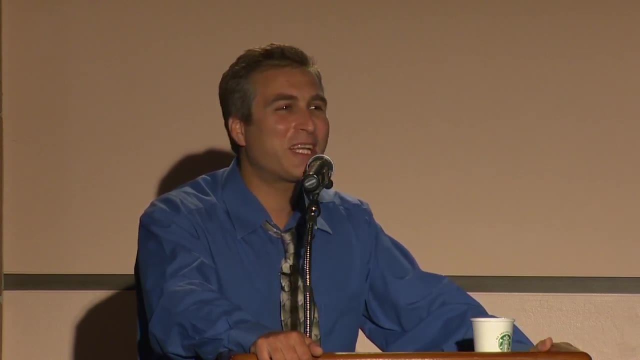 shark species and what isn't. The indications are that thresher shark, as of right now, is a sustainable species, at the rate it's being harvested. But in Mexico, again, we're not sure what's happening. Those artisanal fisheries have not been monitored. 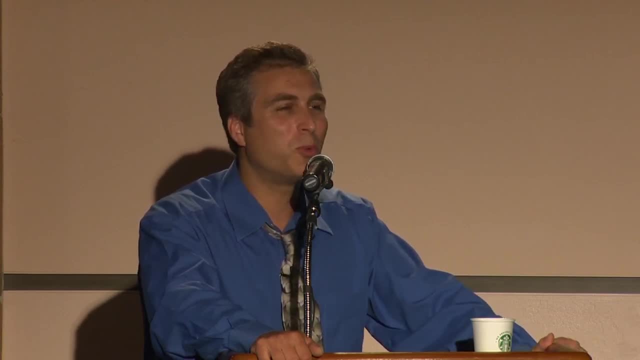 for regularly. I don't think the catch has increased from what we saw, But they're considering reinstituting their drift gillnet fishery. So it's a very complicated and ever-changing story and you have to stay on top of it. Do sharks communicate within each other? Sharks can. 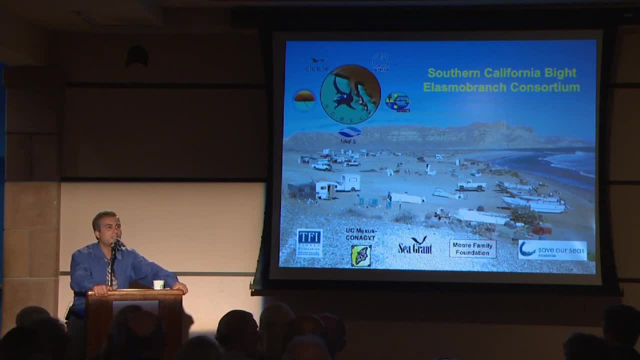 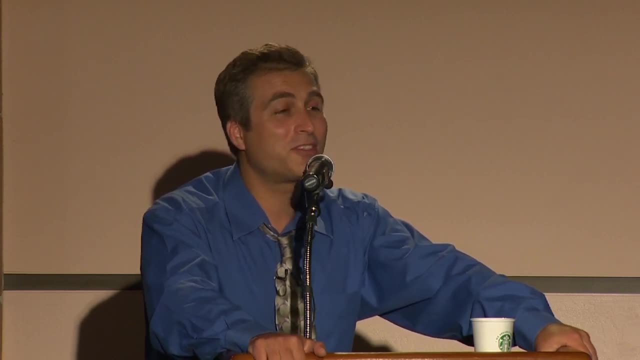 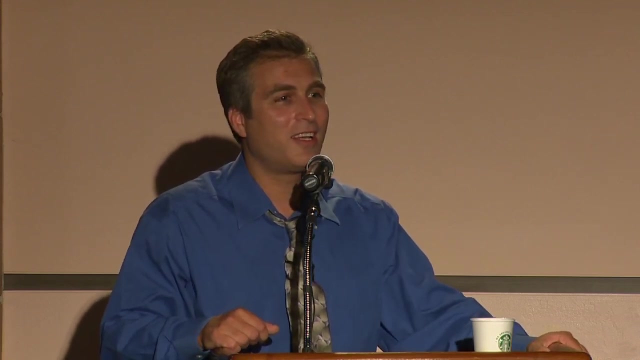 communicate, but not not with sound. Typically sharks communicate via movement, So sharks will, and they communicate with other species as well. So some sharks have a characteristic posture that indicates beware. Other than that, there's not a lot of inter-specific, inter-shark. 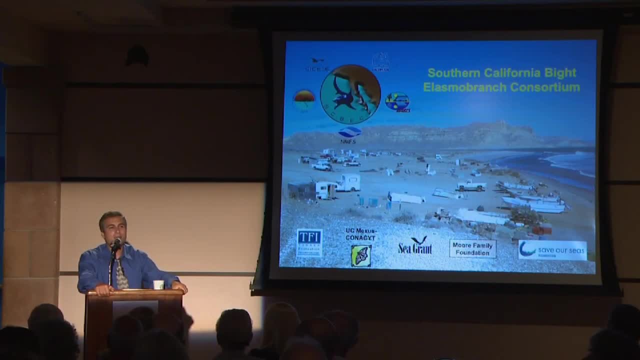 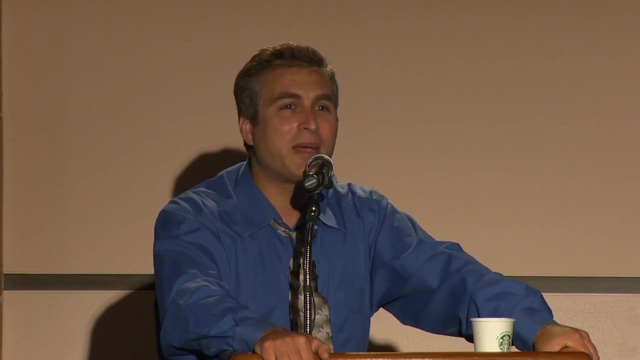 communication. Okay, can I generalize about the state of other sharks such as makos and blues? Makos and blues are a tougher situation because they're offshore sharks and they're also very highly impacted by fisheries like the drift gillnet fishery. The fact that the drift gillnet fishery is very highly 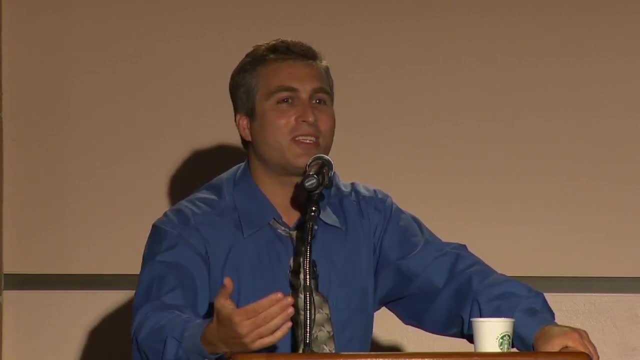 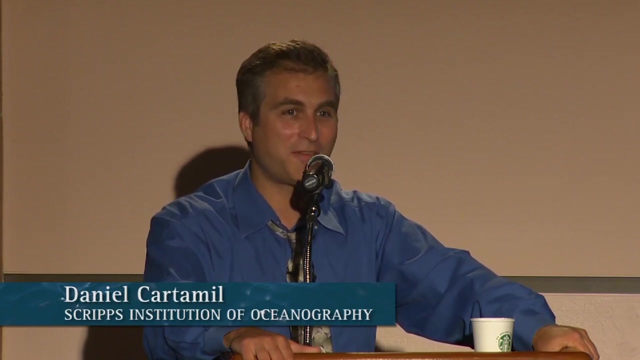 regulated and is constantly decreasing in size because of increasing regulations being put on that fishery is a positive sign, and I would assume that those fisheries are, that those species are recovering as well, but probably not at a very fast rate, and I couldn't give you a good answer for that. What I will say is: that the inshore shark species. we have a much better idea of what's going on. Up until fairly recently, fishers were allowed to put gillnets very close to shore, within three miles of shore, so right up to the beach, fishing for things like sea bass. So you can. 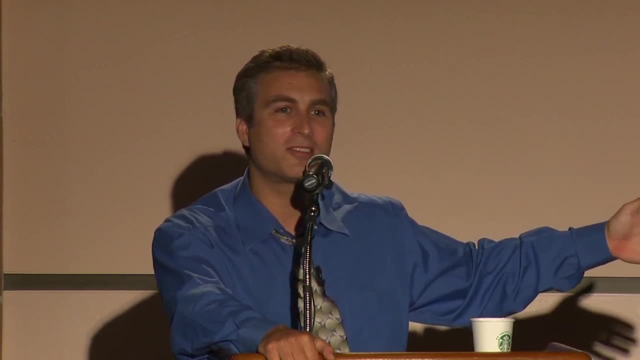 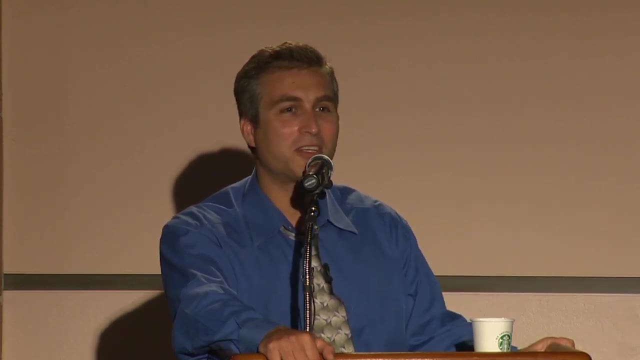 imagine if you have- you've ever been in La Jolla Cove- it's filled with leopard sharks. You can imagine if you put a bunch of nets in there. within a couple of days that huge aggregation of leopard sharks would be in your net and no longer. 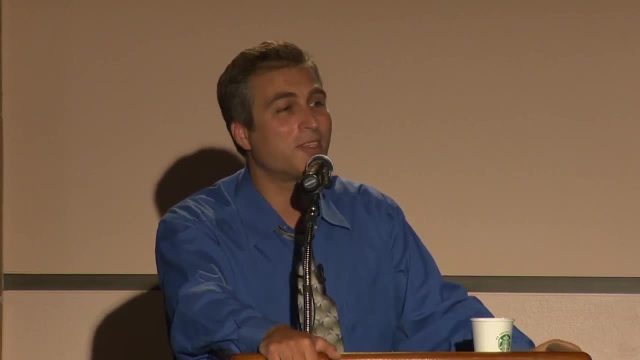 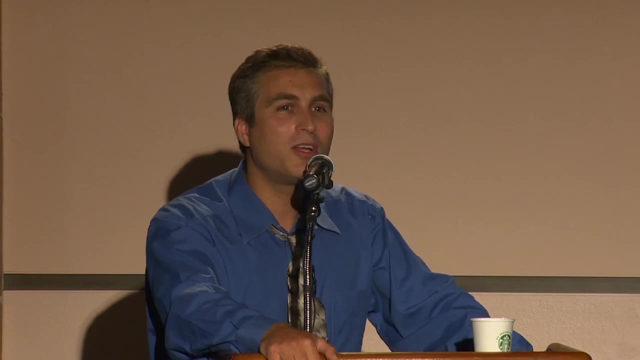 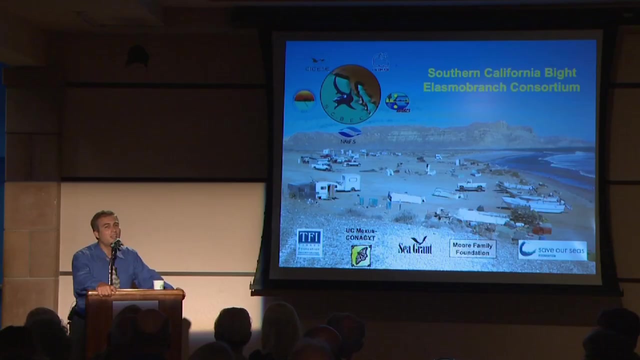 be there and it would take decades to rebuild that population. But since gillnets have been banned within three miles of shore, we have seen a huge increase in the number of near shore shark and race species, as well as other species like white sea bass. So that is a big success story and probably has something to do. 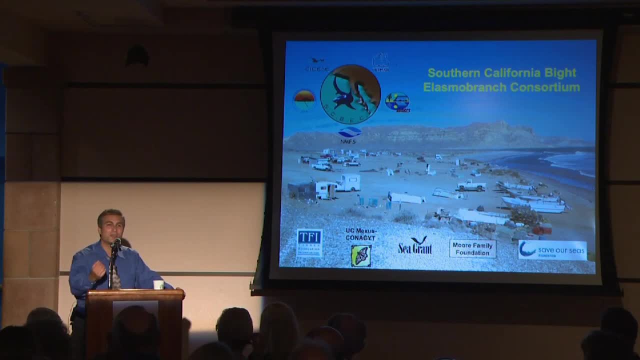 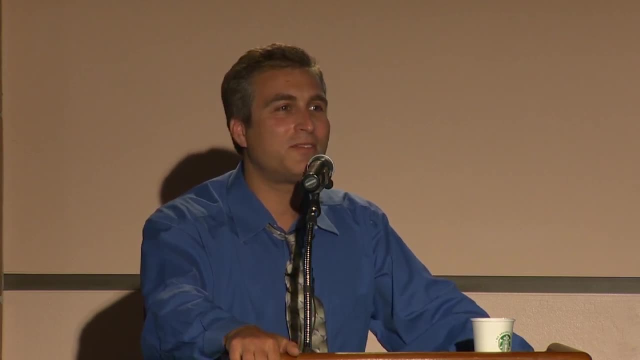 with the rebuilding of things like thresher shark stocks as well, because they're no longer catching as many juvenile threshers, which use the inshore waters as a nursery- And I've heard of some very interesting studies where white shark populations are also recovered- are also thought to be recovering very well because of that. 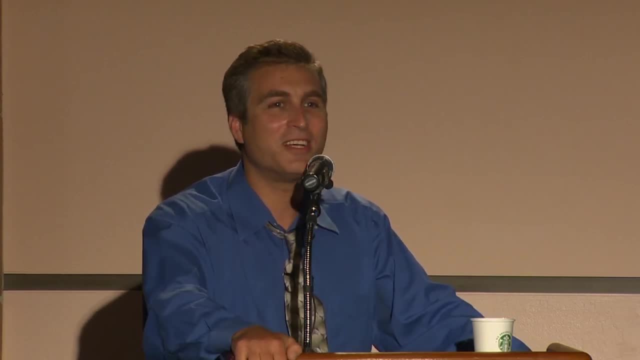 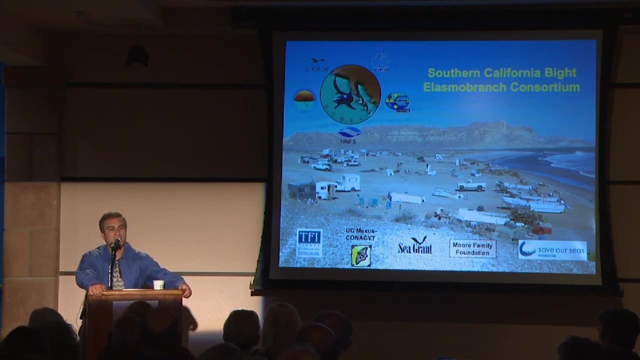 ban and the decrease in mortality on juveniles. Yes, so the question is, when I showed some of those graphs, for example showing the number of species and were the were, it was the catch comprised only of sharks and rays, or were there other fish as well? And that's a that's a good question. Some of the fisheries for 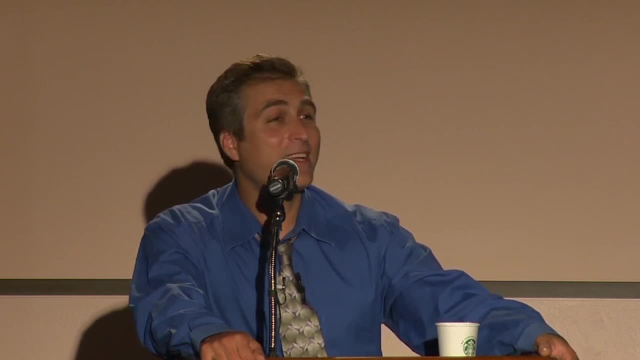 example, the long line. they go offshore and set hooks. You're not going to catch anything from the long line. You're not going to catch anything from the long line. You're not going to catch anything from the long line. You're not going to catch anything. 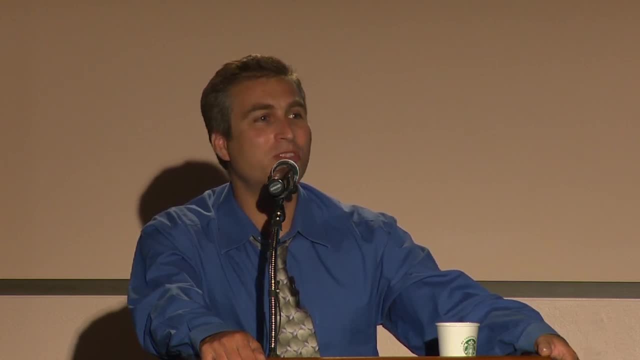 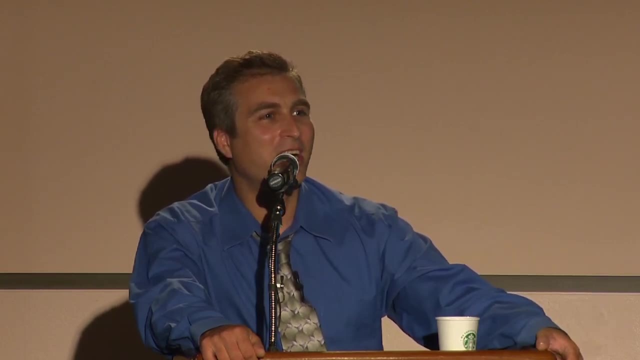 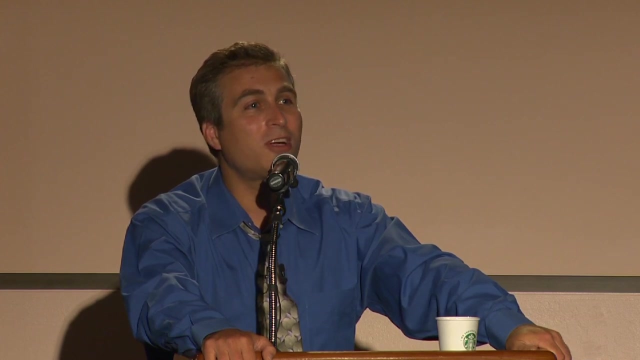 out 20 miles offshore, except for sharks and rays, Blue sharks and makos almost exclusively. You'll catch a couple of other things, maybe every once in a while a rare mahi-mahi or a sunfish or something like that, but those are targeting sharks Inshore. some of the fishermen do target sharks specifically. 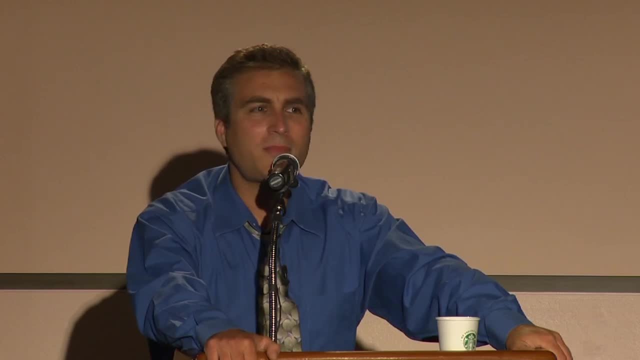 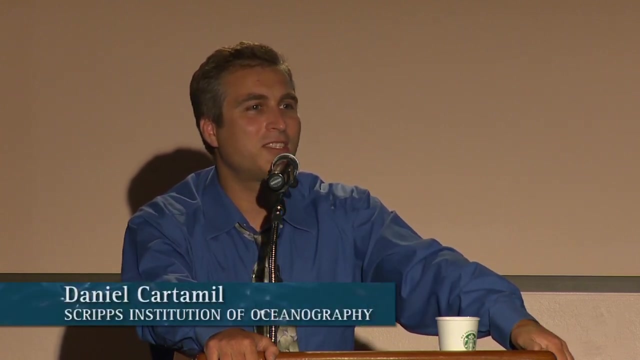 things like guitarfish and they will catch very little else because they know where the guitarfish are. You wouldn't think of a guitarfish as a great target species. We would never eat a guitarfish in the United States, but if you go into Baja and you've eaten fish tacos, chances are you've eaten a guitarfish or a blue. 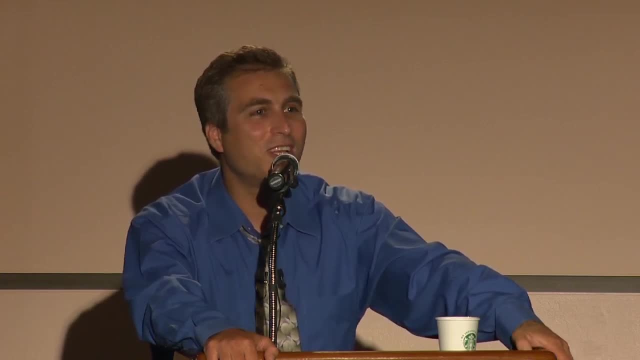 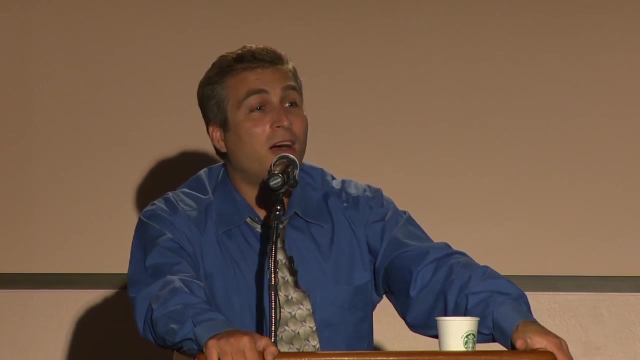 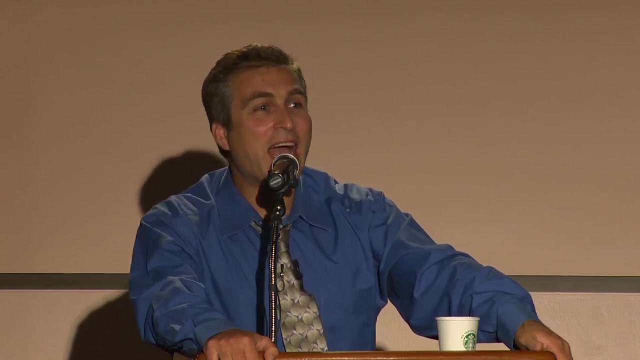 shark, because that's that's the cheapest fish and it tastes just like anything else when you boil the heck out of it in oil. But there are. but, that being said, they do target other things like white sea bass that are much more lucrative, and halibut. Halibut is a very big fishery. 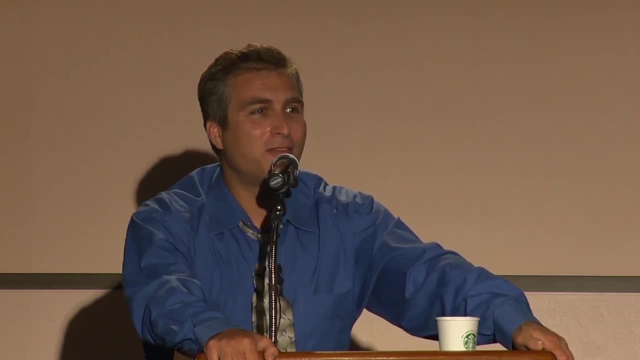 and when you target halibut, the fishermen know where to fish and they'll catch a lot of halibut, but they'll probably catch a lot of other things like guitarfish, soup, fin sharks and bat rays and the like and they will keep those. But we did not keep track of that. it was just way too much where we were. interested in sharks and rays, and so we. if we'd sat there collecting data from every fin fish that came up, we'd still be there. How long do sharks live? Well, it depends on the species, but thresher sharks, for example, probably live to about 40 years. Some other species live a little longer, some live shorter, but thresher sharks live about 40 years. How do they preserve the fish? Well, that's a good question, but it's not that hard even in these remote areas. what happens is a van will come down the road. I don't know how they match these roads with a. 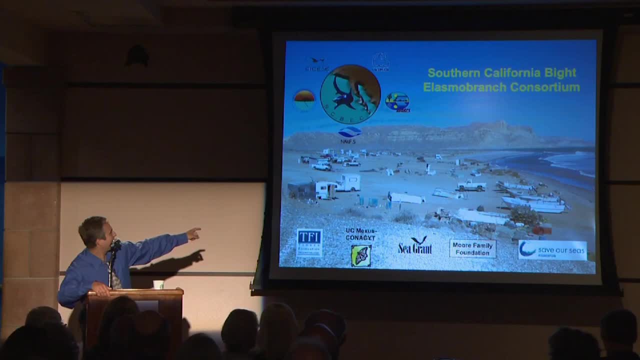 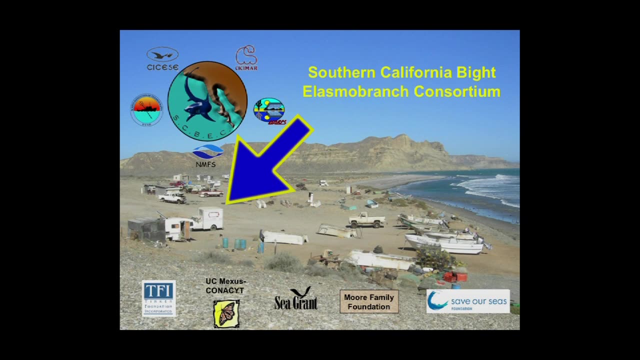 van, but it'll be a van full of ice, and one of these, for example, this one right here, will be just filled with ice, and so they'll throw their catch in there, or they'll have a few of those, and the van will come through every four or five days pick up the catch and replenish the the ice. 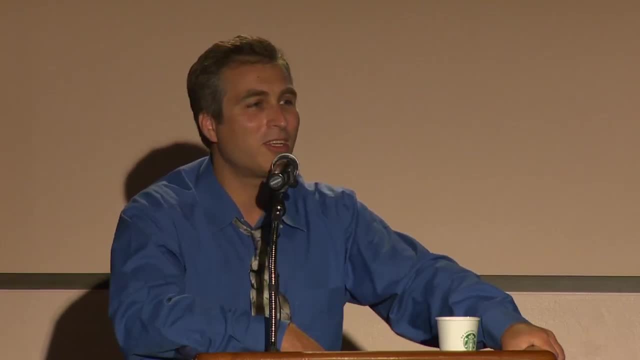 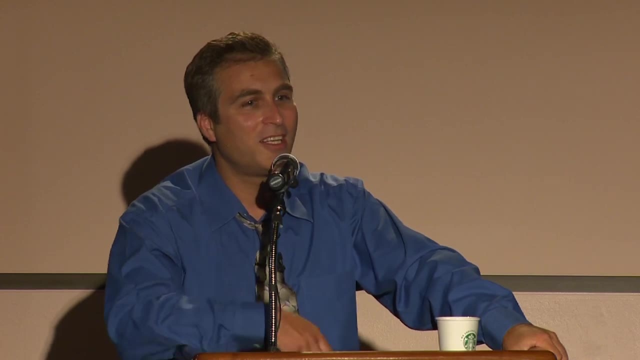 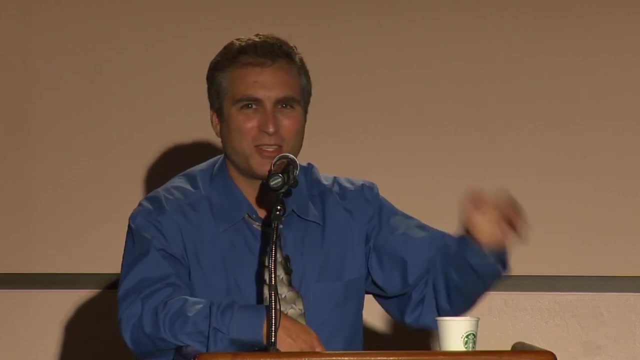 supply. Also, in many cases, the artisanal fishing camps are not this remote. they're located near, within a half an hour of a town, and so the fishermen live in town and they bring the catch back to town and store it- there They're in some refrigerated facility. I think we have time for one more question. 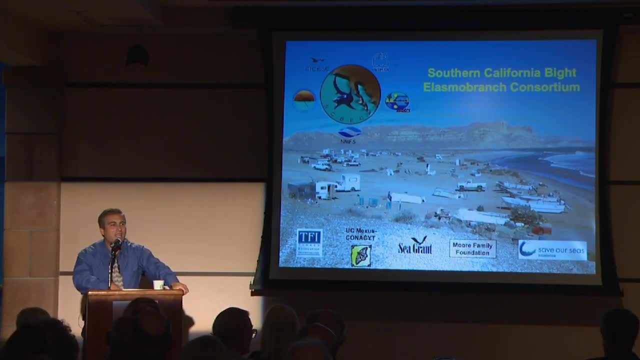 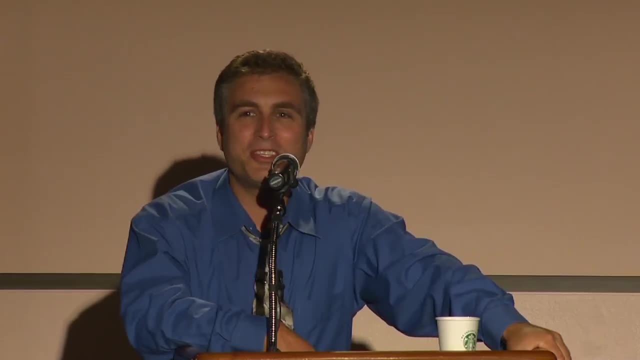 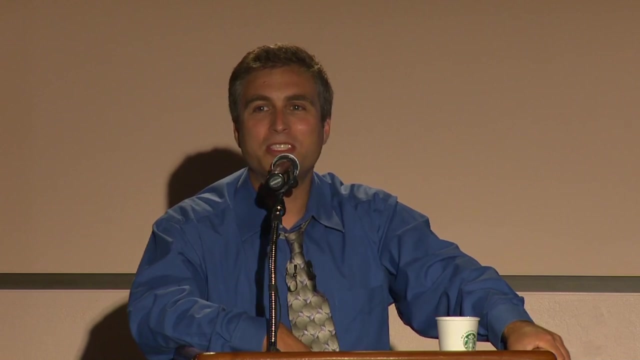 all the way in the back. So the question is, how are the rays doing? and that's that's another really good question. If you consider a species like the California bat ray, which is one of the primary species that are caught there, or even the shovel-nosed guitarfish, these are species that are not harvested in.